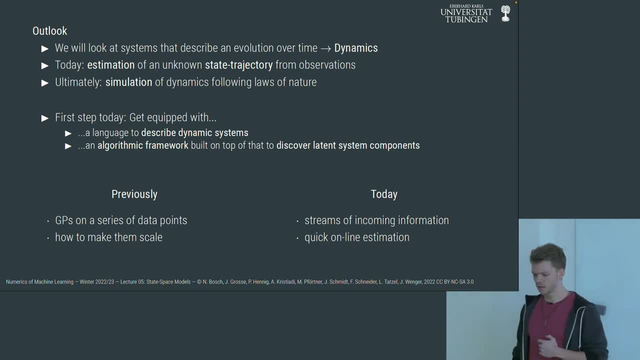 in two weeks. So similar to the structure that Jonathan Wenger and Marvin chose for the linear algebra and Gaussian process lectures. we first have to kind of chew through a bit of theory and we have to look at stuff that has been around for quite a while actually, in order to get to know what cool stuff 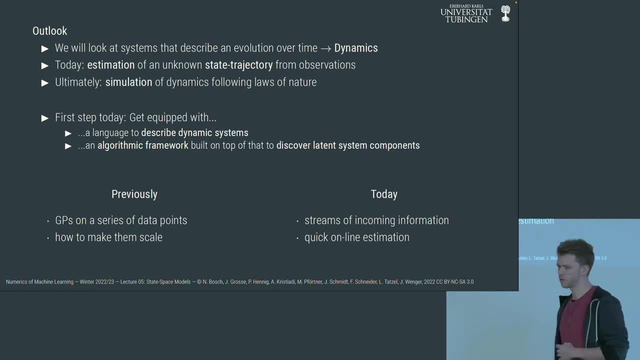 we can use this for. So this is what we're going to do today: We're going to establish a bit of groundwork, We're going to construct a language in which we will describe dynamic systems, And on top of this language, we are going to build an algorithmic framework that allows us to. 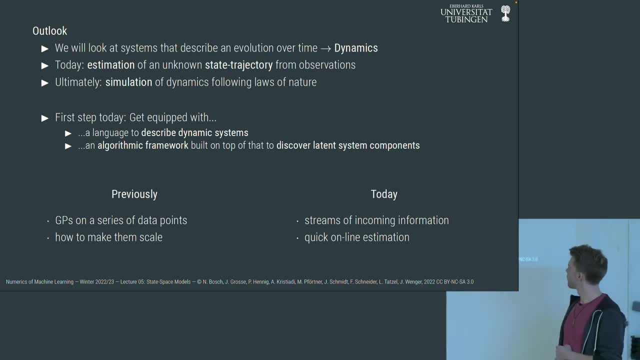 discover latent components of such systems from parts that are actually observable, so from data. To put this lecture now, content-wise, a bit into context. So previously you learned about linear algebra and Gaussian processes, so basically a regression task, trying to find the posterior over a function that describes a fixed set of data. 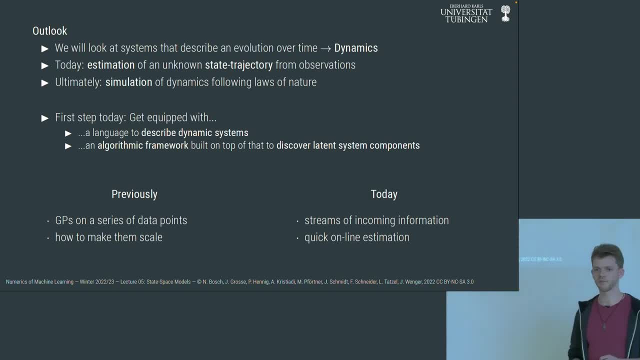 So you're given a data set and you're trying to find a function or posterior over a function that describes this data well, And Jonathan then showed us, last week in particular, how to make these techniques scale on huge data sets- maybe so huge they don't even fit onto your computer anymore. 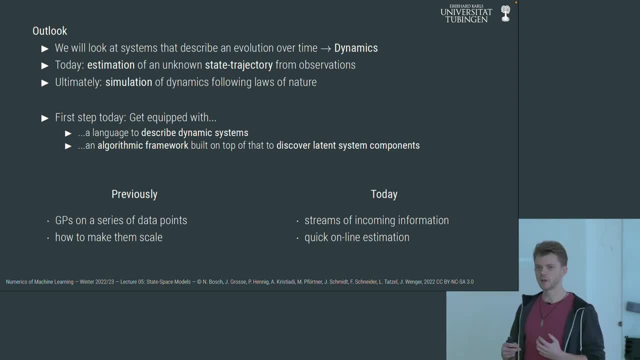 Today we are going to, as I already said, open a bit of a new chapter. Today we are going to shift the setting which we think about a bit to settings in which we are dealing not with fixed data sets but rather with streams of information. 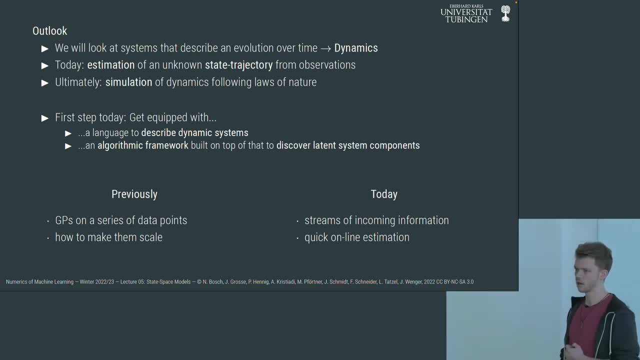 So maybe we don't even know all of the data we are going to see or how big the data set in the end will be, But there's really information trickling in, one at a time. We want to estimate the state of our system in an online environment. 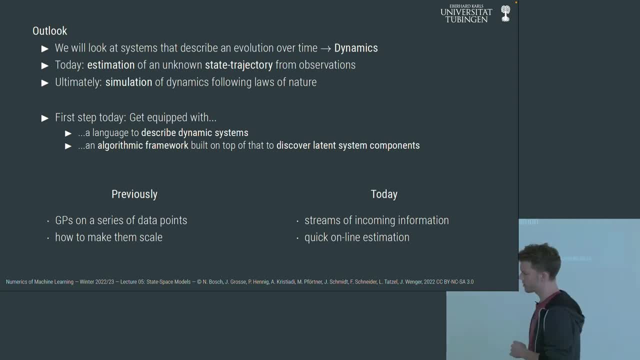 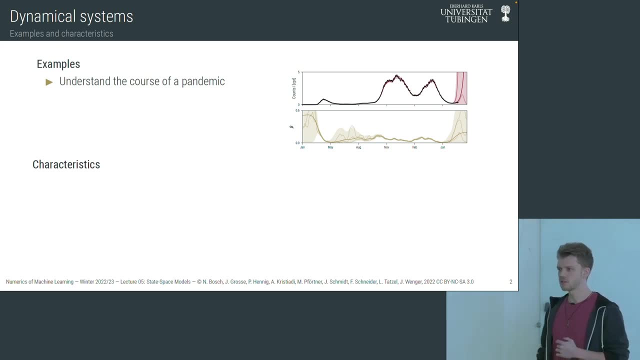 We want to estimate the state of our system in an online fashion And, to start off, let us look at a few examples of such system I've been going on about now And while looking at those examples, I'm not only going to tell you that these systems 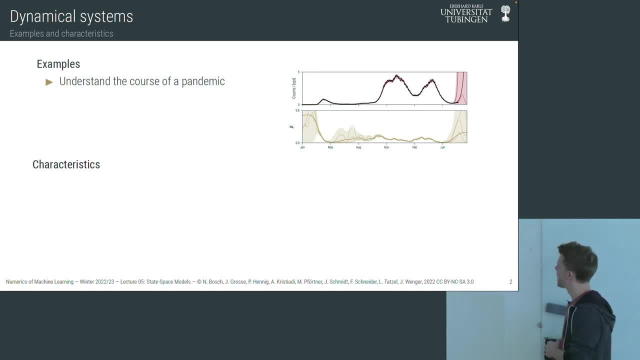 are actually useful, because otherwise I wouldn't be telling you about those. but we are going to extract from this example a few key characteristics of dynamical systems and of this model, or the characteristics we really want to be reflected in the model we chose to model: those dynamics. 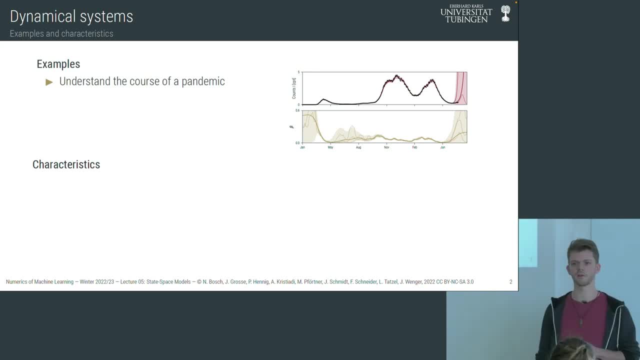 So let us start off with this example. you saw already in the very first lecture given by Professor Hennig. It's data from the COVID-19 pandemic And not only data we see here in this red line. Let's test this. It actually works. 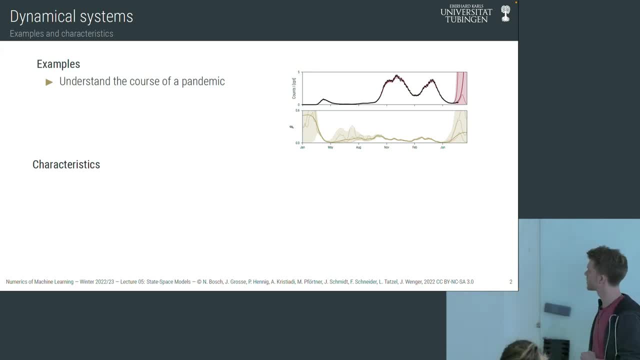 And this red line. we see a Gaussian process posterior fit through this data and a bit of a prediction afterwards. It's the number of infected case counts per every day in this COVID-19 pandemic And on the bottom you see this beta parameter which is also an evolution over time. 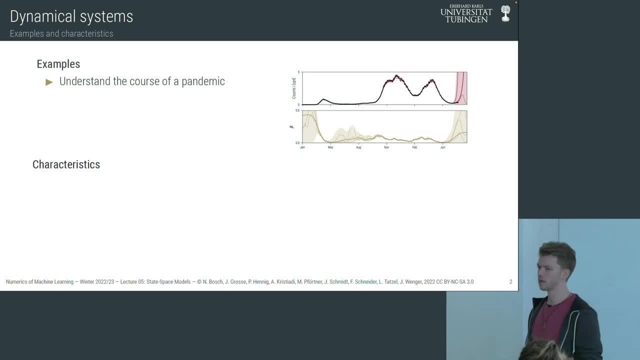 which is interpreted in these kinds of model, interpreted as a contact rate between individuals in a population. And there, of course, you see, as I already said, the key characteristic of dynamical system is we have this temporal structure, We have this temporal evolution right. 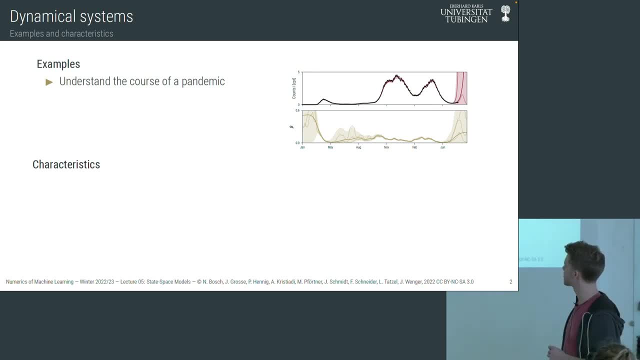 But what you can also think about is that we can only observe parts of the system. We can measure the infected case counts because we have COVID tests. Maybe they are unreliable, but still it's a means of gaining information about a part of our system. 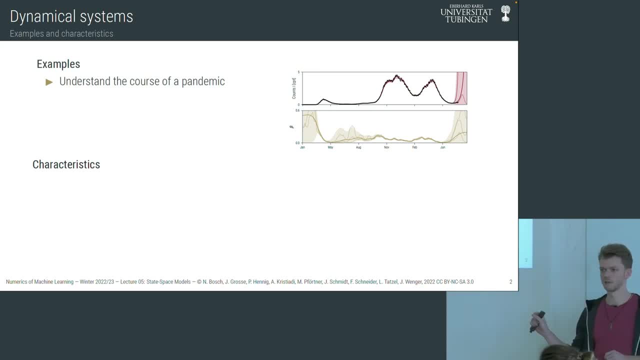 But we don't have any means of monitoring. So we can only observe parts of the system, But we don't have any means of measuring this contact rate. At least I hope so. It would be really questionable if we had means to measure the contact rate between individuals. 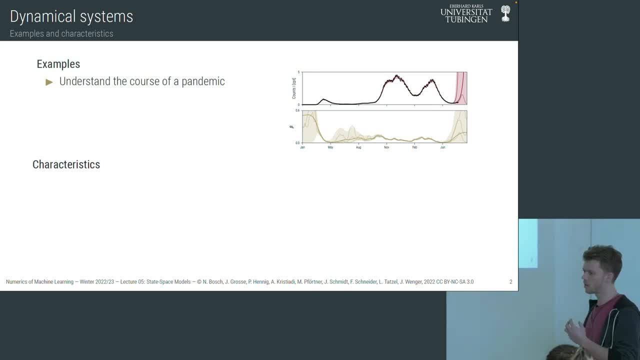 So this is a part of a system that is hidden to us. It's a latent force. Okay, Moving on to the next example, which is a bit different in the way at the speed that data basically trickles in, Because while we maybe get a new estimate for the infected case counts and the COVID-19. 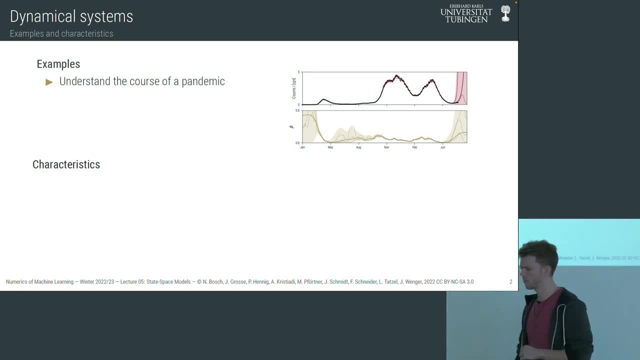 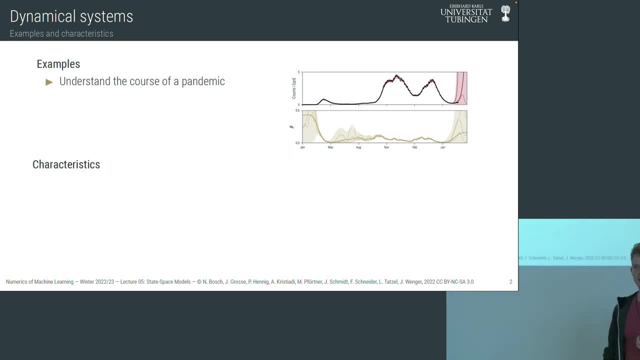 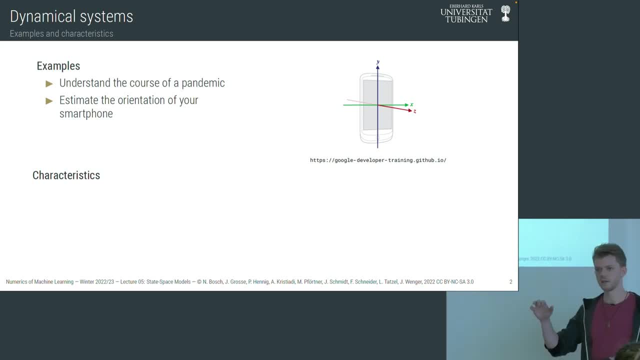 No one really knows. Yeah, If we want to do something… But then this whole drilling question, the box collection, right, which was actually the cost of not knowing that- data beautifully trickles in, because while we maybe get a new estimate for the infected case counts and the COVID-19 pandemic, once a day, if you. 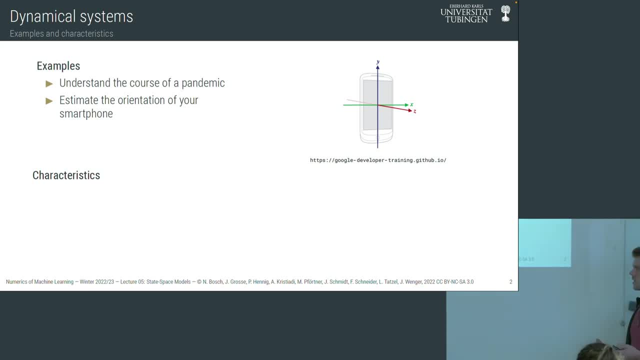 think about an application that estimates the orientation of your smartphone in the three-dimensional space. probably you're going to have to process a rapid fire of information coming from the sensors in your device. Maybe there have some accelerometers built in there and some application on your device. 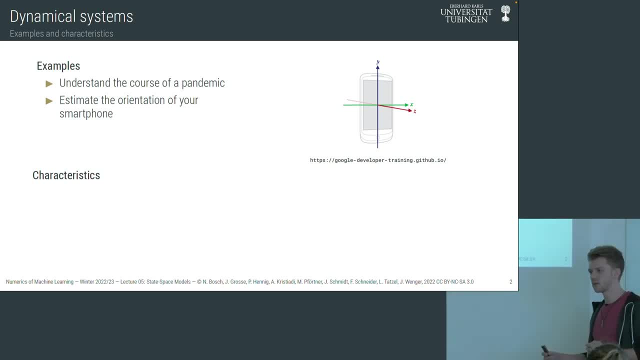 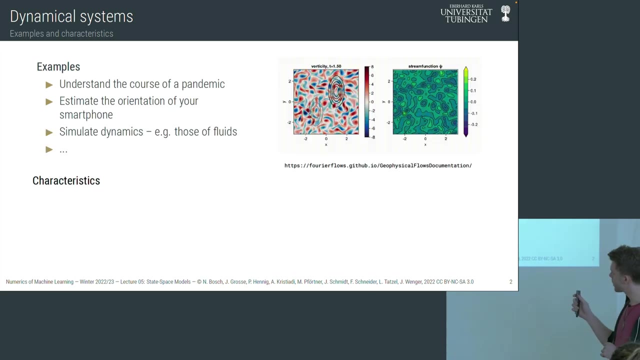 analyzes this data and has a built-in model for these dynamics and estimates the orientation of your data device. So we really have an online estimation task here at hand in which we have to quickly update our estimate And, as I already promised, we are working towards a task that is called 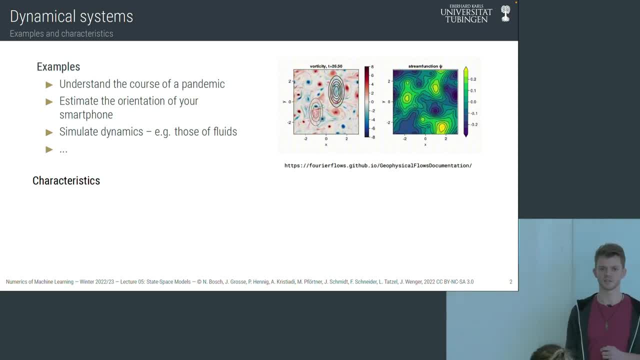 simulation: Simulation of dynamical systems. This is really a very interesting task. Here on the right hand side you see a fancy animation of a very difficult to simulate dynamical system. and we are not going to talk about such difficult to simulate systems, because this is a spatiotemporal dynamic system, so it not only evolves over time, but also over. 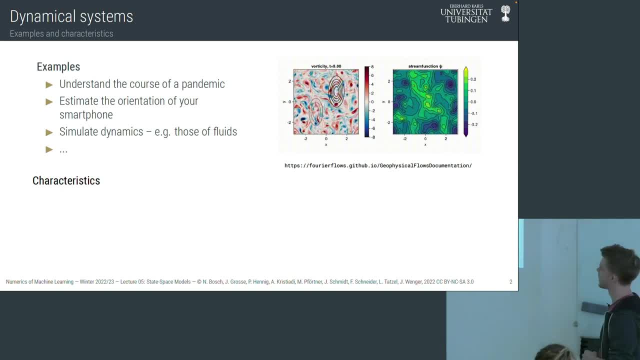 two dimensional space, And this is also a very difficult model to simulate. It's a fluid, dynamical system. I just wanted to show you where this might be leading in the future. So what are the characteristics now that we learned about? We already talked about this. 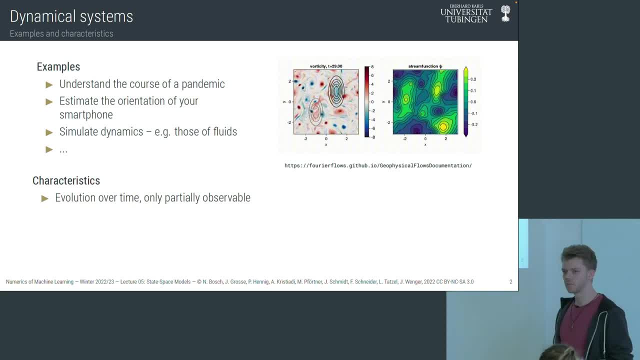 evolution over time and we talked about models being only partially observable. Then we have in these, especially in this simulation task, we are faced with very complex dynamics. So we might be dealing with highly non-linear functions and interactions. So we have to find a way to deal with those. But I think 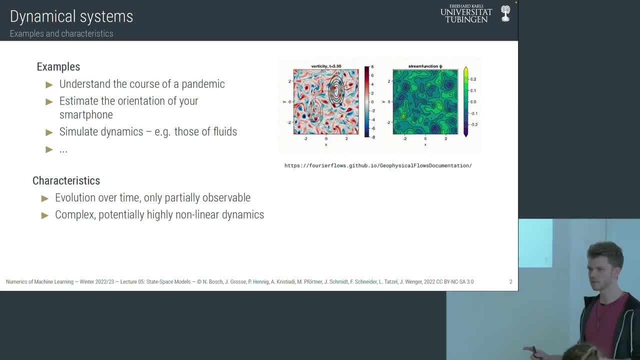 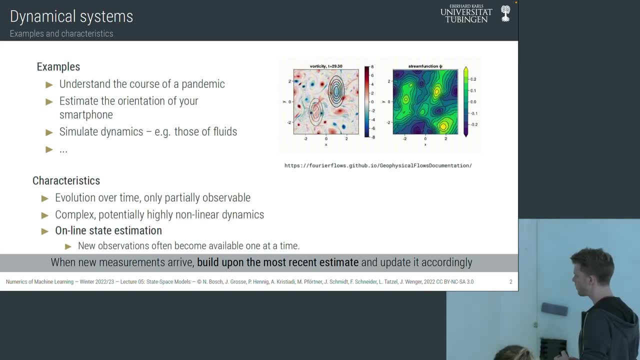 the thing which I want you to keep in mind over the next couple of slides in particular is really this online estimation setting. So we need an algorithmic framework on top of our modeling language that allows us to build upon the most recent piece of information that trickles in and update our belief accordingly. 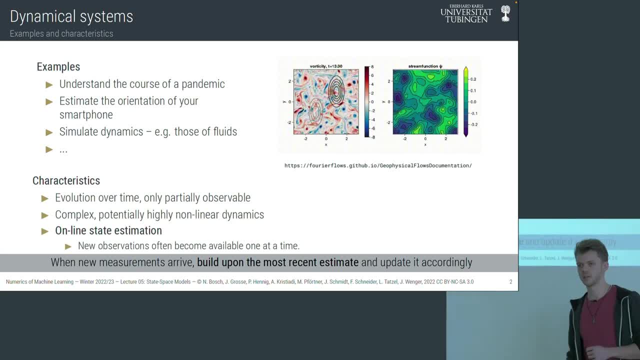 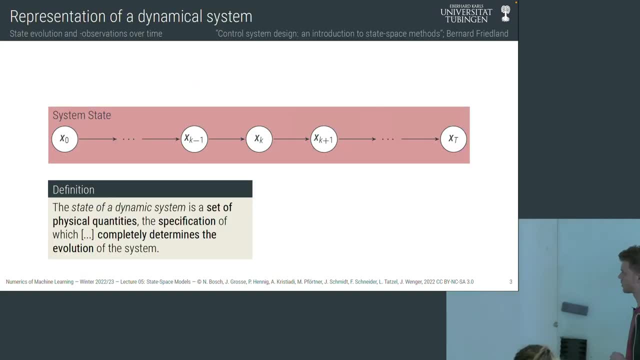 OK, But now that we know what we want to do, let us actually look at how we are going to do this. And we're first of all going to look at a graphical representation of the modeling language we choose, And this is also a figure you saw in the very first lecture. 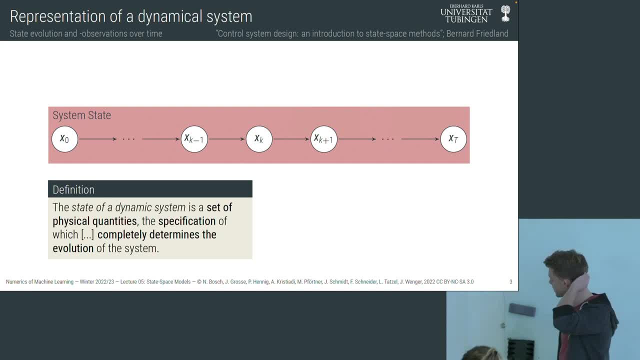 already. Professor Hennig introduced this in the first lecture, And I'm going to walk you through this step by step now. What you see here in this red box, is a sequence of white nodes, And these white nodes represent random variables. These are the variables modeling our system state. OK, First of all, what is a system? 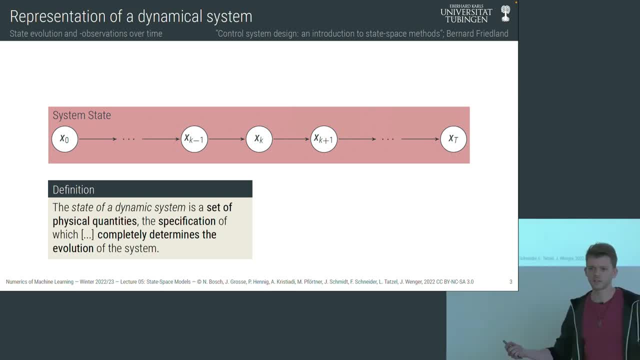 state. In order to define this, I think you could look up 100 different definitions in 100 different books, But I chose one of them because it carries everything that I want to say about these systems. So the definition reads: the state of a dynamic system is a. 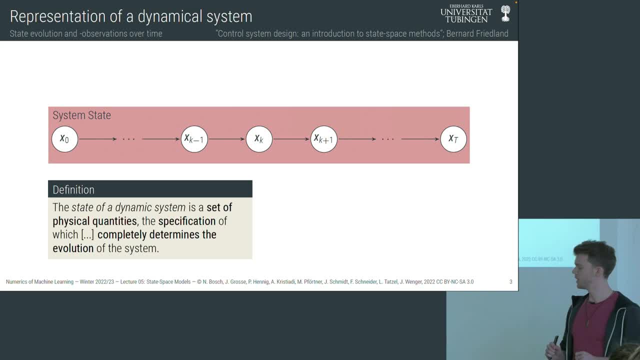 set of physical quantities, the specification of which completely determines the evolution of the system. OK, So there's a lot to be learned from the definition. First of all, a state is not a system. It's not only one quantity, It's not something, one number which we want to model, not one. 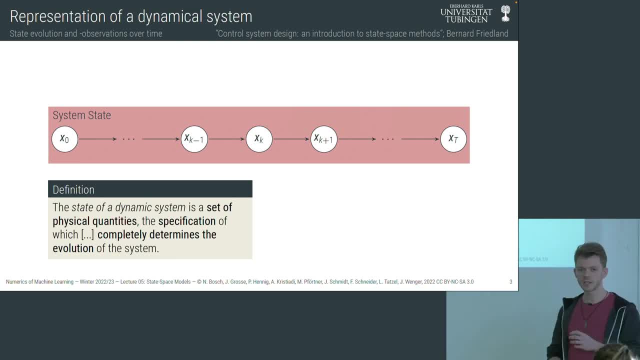 trajectory, but really a set of physical quantities that are tracked in the same state and are expected to interact in a potentially very complicated way. So we have to specify this set of physical quantities And actually I brought some examples what these quantities could be. So, for example, in a very canonical dynamical system that 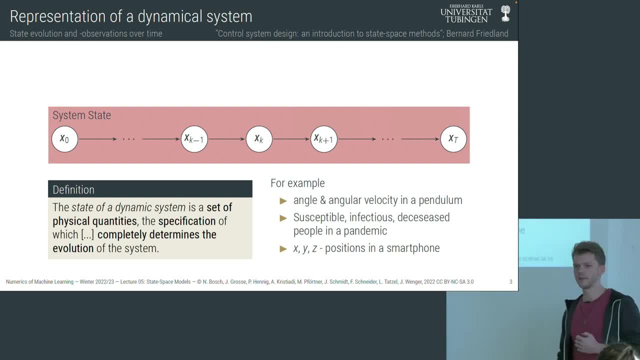 is often used to teach about a dynamical system. it's a pendulum model. There you model the angle of the pendulum and the angular velocity at every time step. So this is quite simple. It's just two quantities that naturally interact with each other, right? But in this COVID. 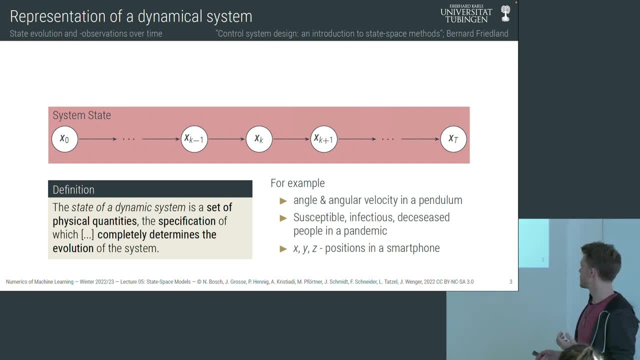 example. it might be a little bit more difficult. So you have to track the amount of susceptible infectious deceased people in a population during a pandemic, but also maybe even more than it first appears. Maybe you want to model such a thing like this contact rate or like: 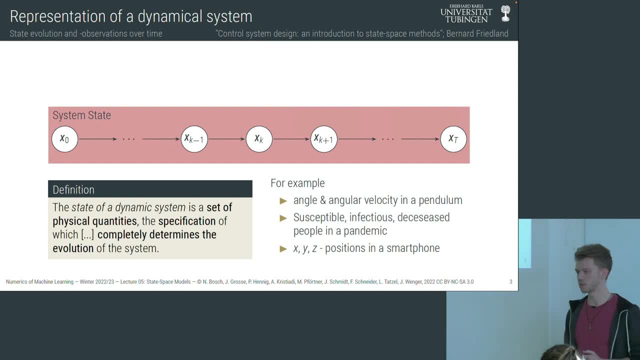 a recovery rate, And all of these are potential components of your state, Or X, Y, Z, positions, velocities, accelerations in three-dimensional space, to do something estimation with your smartphone. OK, Now that we know what a state is, we have to define how we observe the state. And as 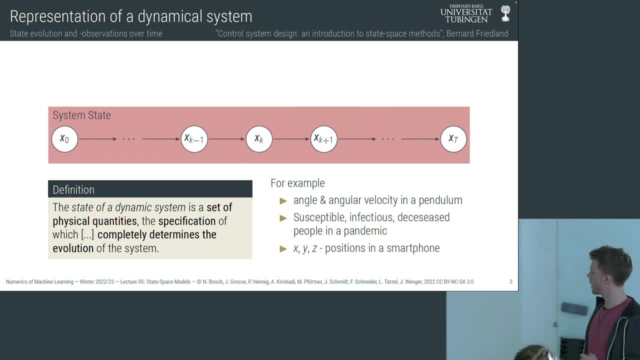 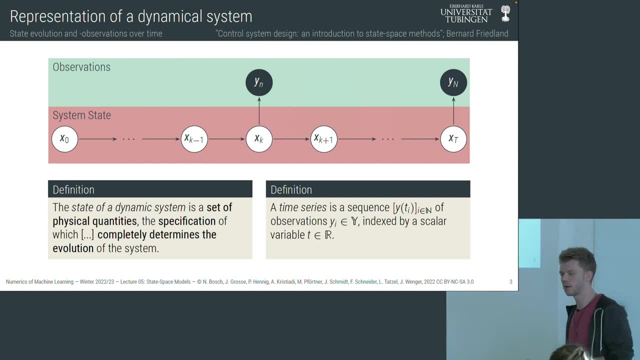 I already told you, in these models they are often called partially observable. We have observations y, So we collect these observations in a random variable y that somehow depends on the present state, And there's a lot. So what I have to take care of in this plot at the moment because I, for example, use 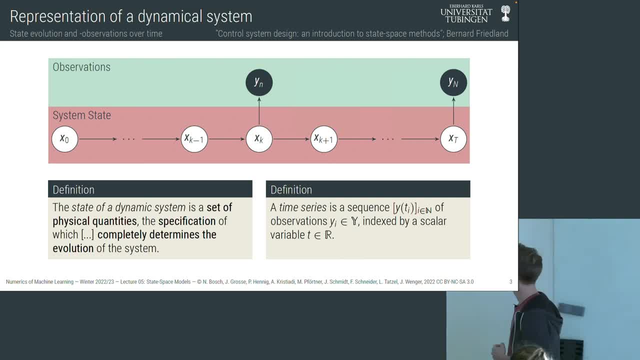 different indices. here We have y sub n and x sub k. So this is kind of confusing, right. But this is just to visually represent the fact that we don't have to collect a measurement at every state or every point in time that we model the state So we can have trajectories. 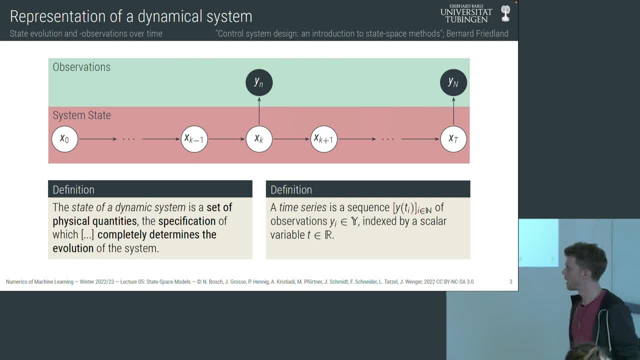 of states where there are no observations available and we can still model them. However, in the future or in the remainder of the lecture, I'm just going to drop these different indices. I'm just always going to write xk and yk so that we just assume we. 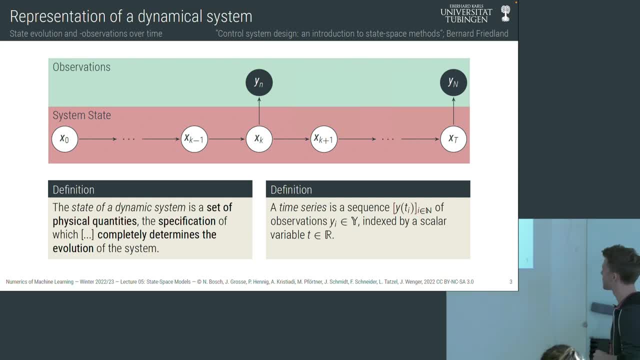 have a measurement for every state of the model, But that is actually not a restriction. So if we now take a step back and look closely at this graphical model, we can actually read off the properties that we want this model to have before we actually go ahead and define. 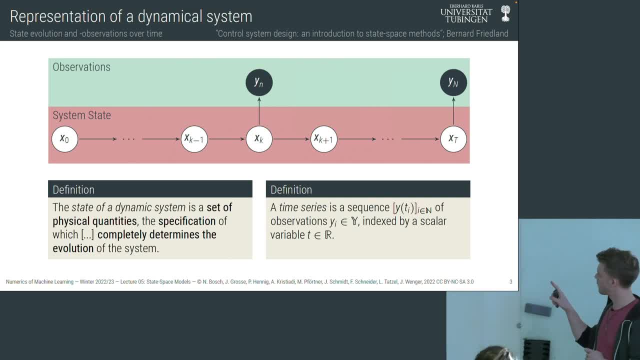 it properly mathematically. The first thing I want you to notice is that there are only errors going from one state to the next. There's no errors going from one state to the next. There's no errors going from xk minus one to xk plus one. Only two subsequent states are connected with an error. 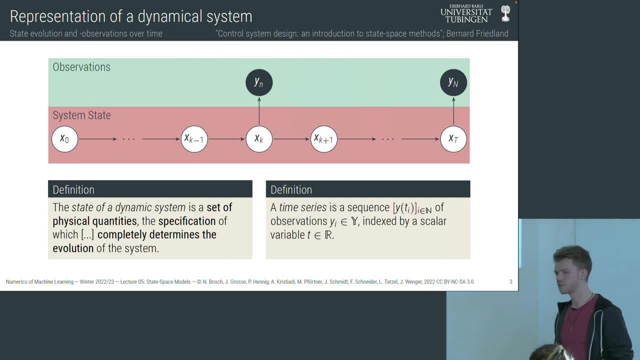 going forward. This is a property of a so-called Markov chain, And this is probably also what the person who wrote this book- I read this definition in- meant by the specification of our current state- completely determines the evolution of the dynamical system in the future. 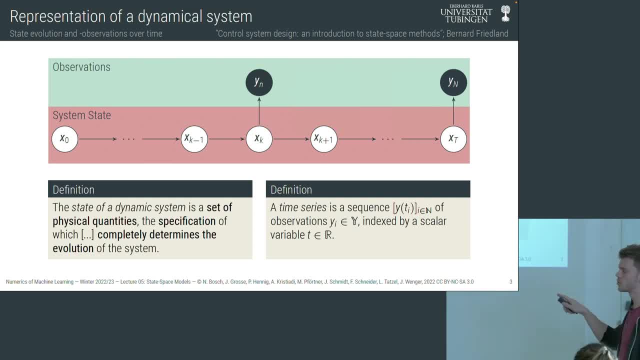 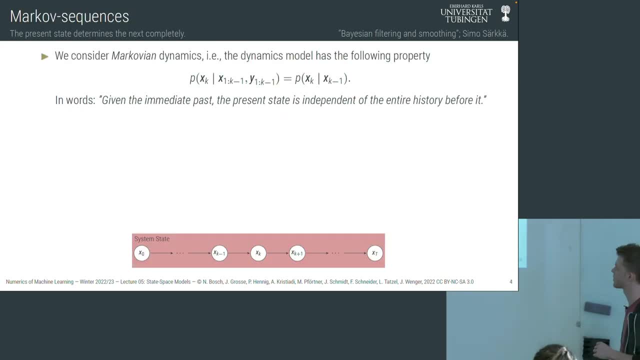 And we are also only going an error from xk to our current measurement. This measurement is not dependent on any future or past states. OK, but enough with the talking, Let's actually make this form. This property, with only an error being between two subsequent states, is called the Markov property, Probably all. 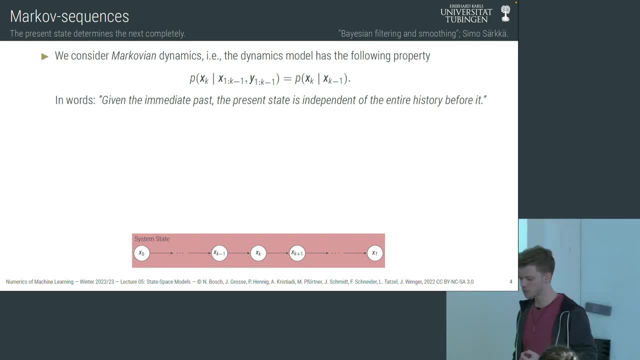 of you know this. The Markov property basically says that if we have a conditional distribution over our current state variable, it is independent of everything else but the immediate previous state variable. This is what this equation here says. So it often reads: given the present. 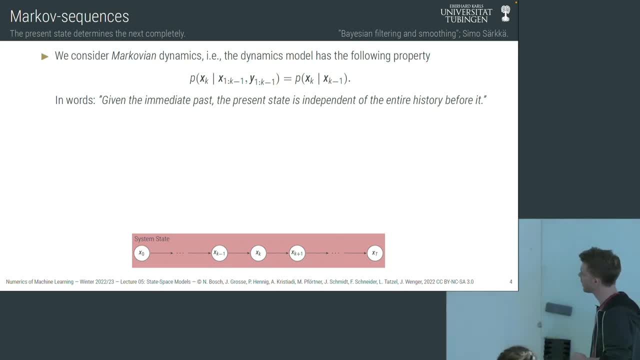 state the future is independent of the entire past. The second property I just highlighted is this of conditionally independent measurements. So our measurement random variable yk is only dependent on xk. This is just an assumption we make which will make computations and derivations later on way easier and very elegant. 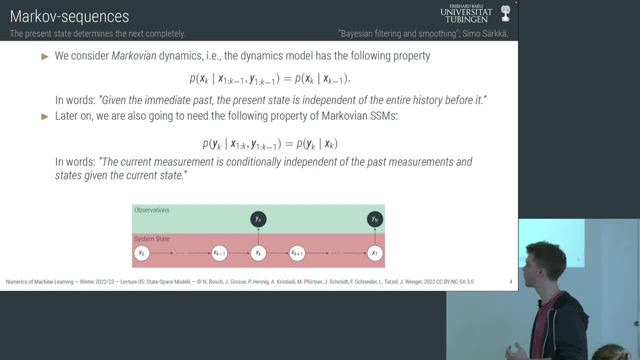 These are two properties which I want you to keep in mind, and they are actually quite intuitive to think about when having in the back of your head this graphical model: The Markov property and conditionally independent measurements. Furthermore, I want to highlight something that I didn't write down here on the slide. 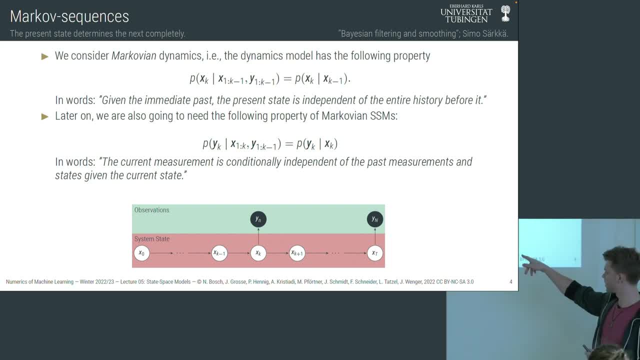 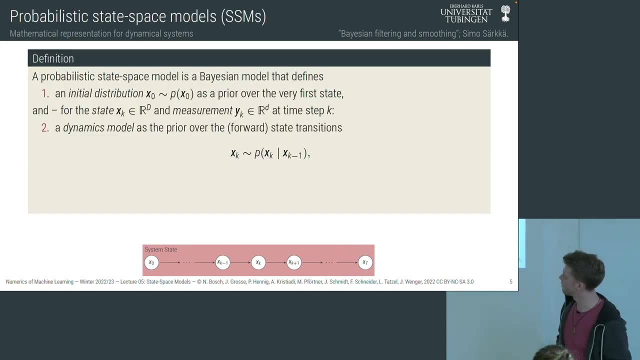 but by extension, you can also read this off from the graphical model: The current measurement is also independent of all future states and all future measurements. With everything that we just learned so far, we can actually now go ahead and write down the definition of a probability. 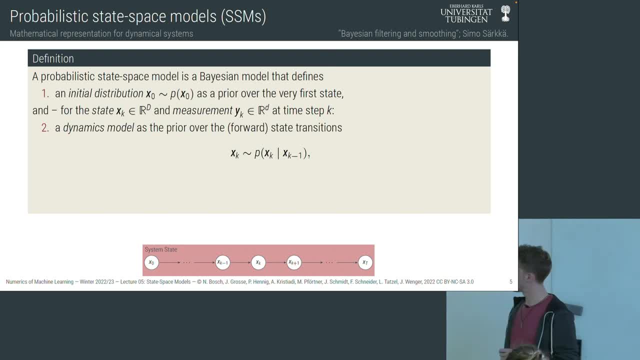 So here is the first example of a probabilistic state-space model, And this is just a Bayesian model that defines three things: First, an initial distribution p of x0 over the very first state in our trajectory And then, for every state, xk in the sequence. 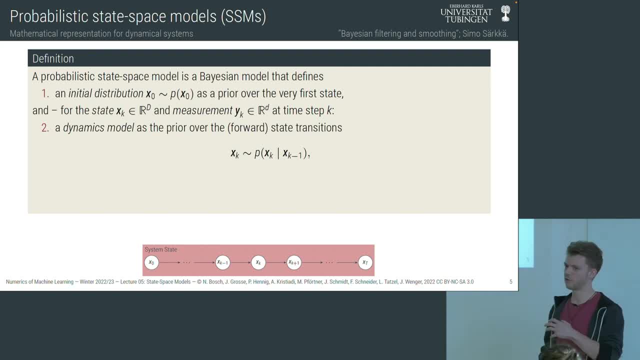 we are considering and for every measurement, yk it defines. Okay, first of all, for xk, it defines a dynamics model as the conditional probability distribution p of xk given xk minus one. So here you see already, Okay. 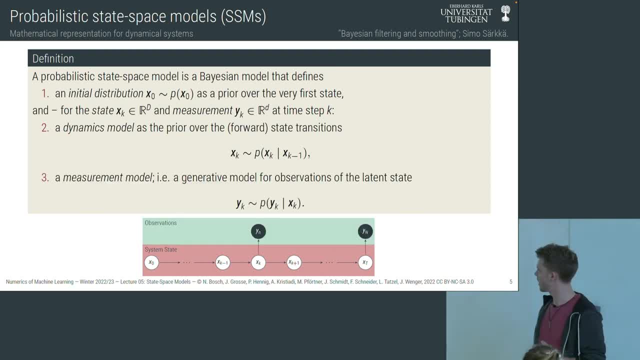 mark of property already, and for the measurements it defines a generative model for our observations. so a likelihood, if you will. it's often called a measurement model. it's just a conditional distribution of yk given xk. it's independent of everything else and this is the entire definition. 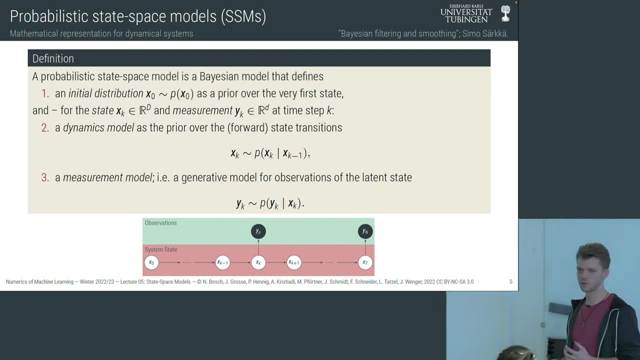 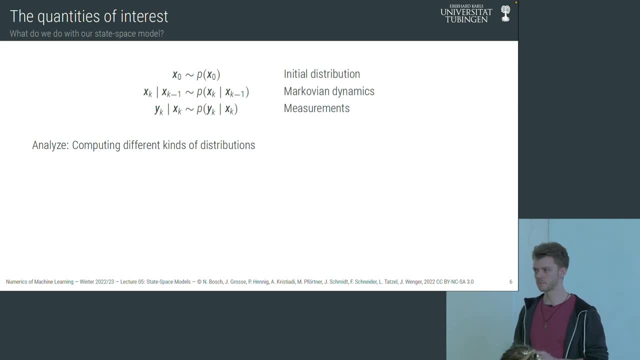 of a probabilistic state space model, the language we are going to use to model dynamical systems. are there questions? so far, i'm going to bring up these distilled components of the state space model throughout a lecture from time to time, because these are really what we are going to use to build our algorithmic framework. 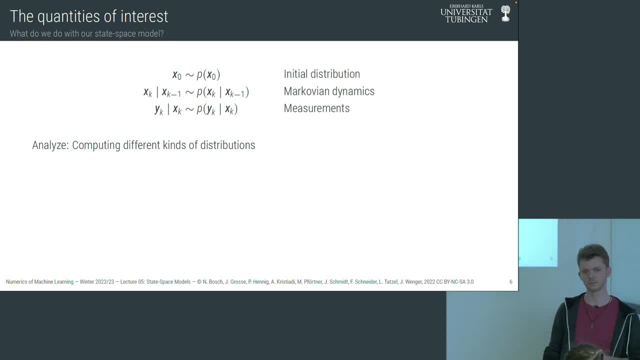 yes for this lecture. a state is the same as a mark of state. yeah, a mark of state depends on the definition of a mark of state. but if the mark of state in your, for your definition, is a state that is given its previous state, you know it fulfills the mark of property, then yes, 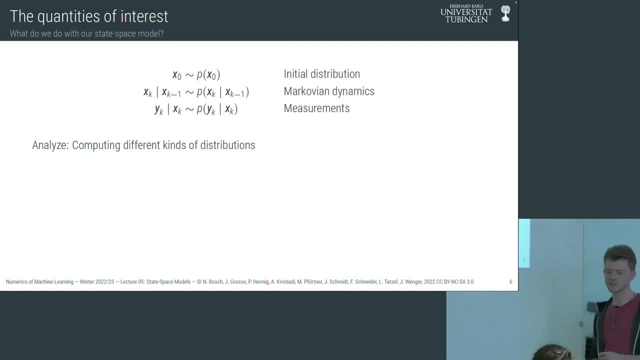 in this case we are considering states in a mark of model. yes, so the question was if the state can be used interchangeably with the term mark of state. yes, yes, implicitly yes. so the question is if xk is independent of xk minus two, but xk minus one is. 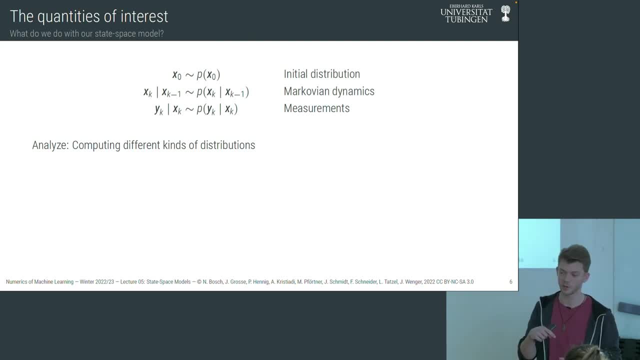 dependent on xk minus two, and xk is dependent on xk minus one. isn't, then, xk also dependent on xk minus two? and yes, that is possible, because otherwise the the we couldn't carry the knowledge onwards. but, um, yeah, it is implicitly dependent on the past. yes, okay, yeah. 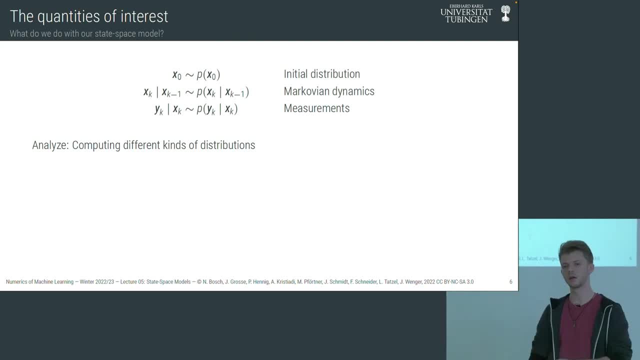 so maybe I have comment on that. might be the difference in that if xk minus one is not kind of observed, then xk and xk minus two is uh- are correlated with xk minus one is observed, and then they're unpredictable, for xk minus one basically captures all these. 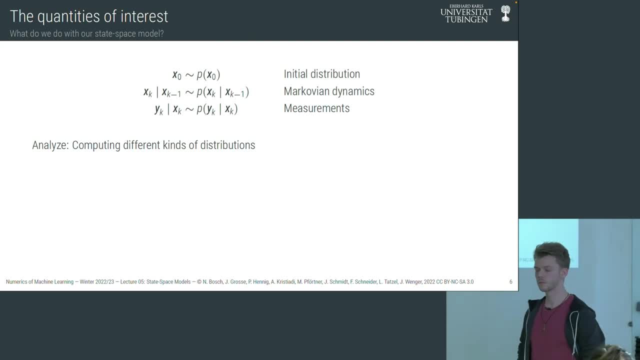 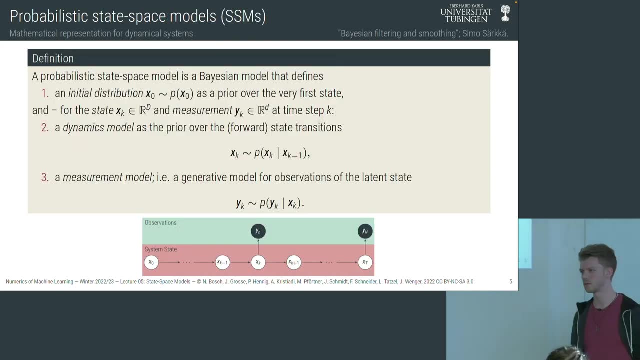 information that xk minus two is required for execution. yeah, exactly, yeah, thanks for the remark. you can also reading this off, actually, from the graphical model. so these, these models are, they are, and so the arrows and the nodes kind of have an in a conditionally independent structure encoded in them. so, um, yeah, this is something that's for. 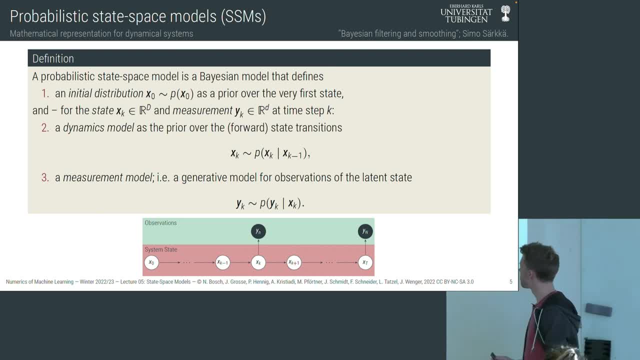 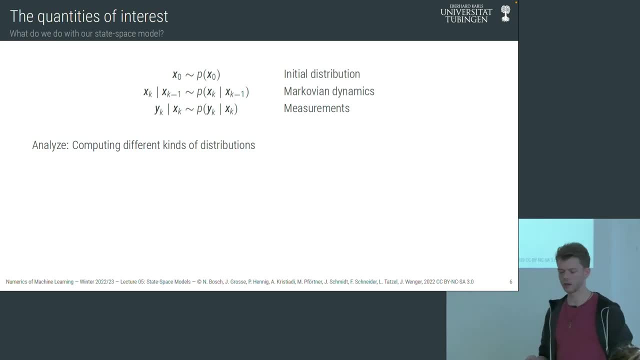 example taught in probabilistic machine learning. um. thanks for the questions and the remarks. um. now let's move on to what we are actually going to do with this definition. now, in order to analyze such systems as dynamics, using these state space models, we are basically computing four different, four different conditional probability distributions. 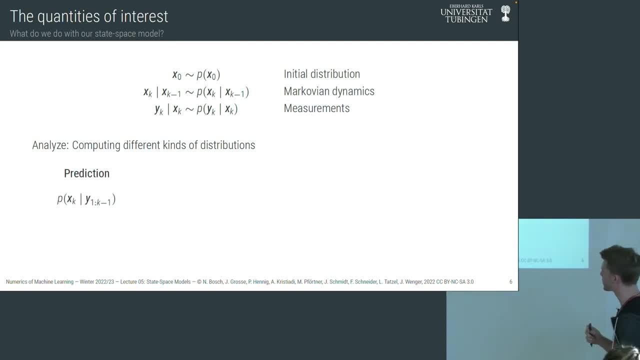 that we can, so to say, label. so first of all, we're going to predict and we're going to compute a prediction distribution which is just a conditional distribution of our present state, given all previous measurements, not including the present measurement. we are also going to compute the 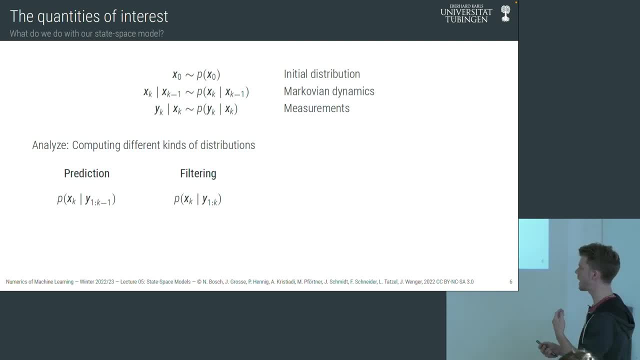 filtering distribution, which then is basically the updated prediction distribution p of x, k, given all the measurements up until k, so including the previous measurements, up until k, so including k. now, along the way we have to compute this quantity, which i call data likelihood, it's just the probability of the current measurements given all the previous measurements. this is something. 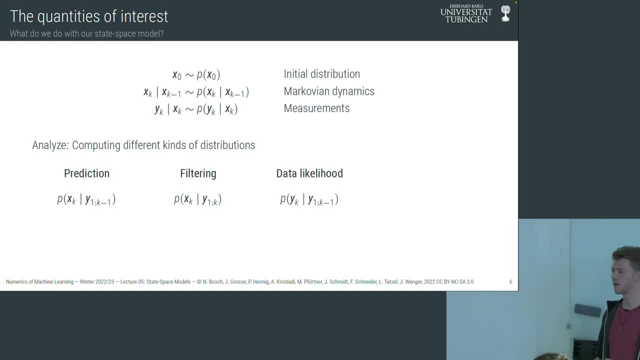 that is not really of high relevance in this lecture, but we have to compute it anyway along the way. so i'm going to show you how, because it's going to be maybe relevant in later lectures. and last but not least, we are going to compute the smoothing distribution, which is the current. 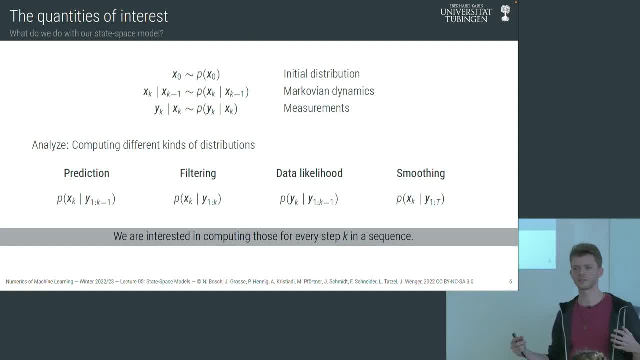 state estimate, given all the data we have. so if we at some point say we have an entire record of the distribution, we are going to compute the smoothing distribution, which is the current state estimate, given all the data we have. so if we at some point say we have an entire, 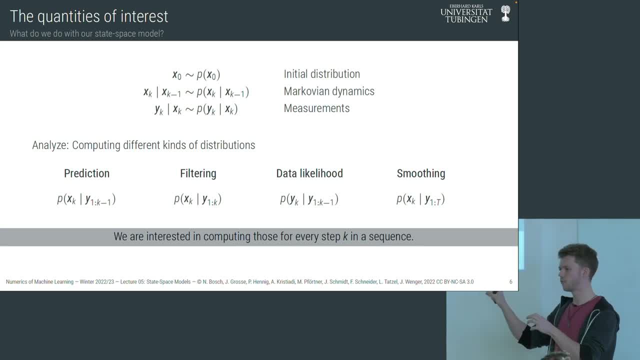 trajectory finished and we want to compute, using future data, the current state estimate. that's called smoothing, but we're going to do that a little bit later in the lecture. and these four probability distributions we want to now compute for every step k in a potentially infinite sequence. of course an infinite, but you know an ongoing sequence. 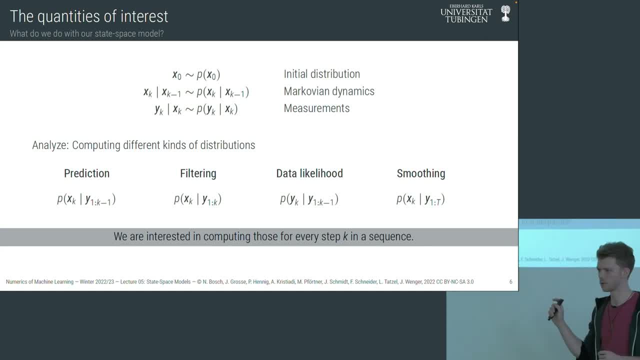 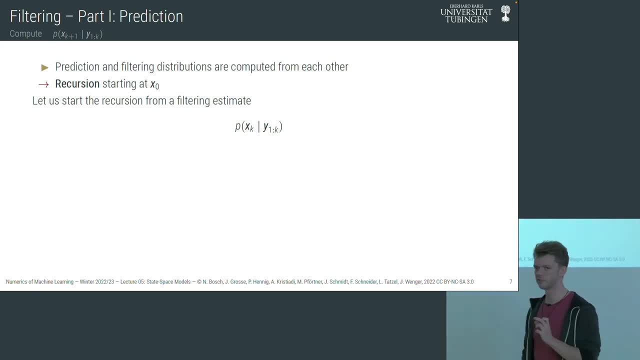 first of all, we are going to derive how we compute the filtering distribution. and in order to compute the filtering distribution we have to learn how to compute a prediction distribution, because those two distributions are computed from each other, so maybe this might seem confusing at first. how can 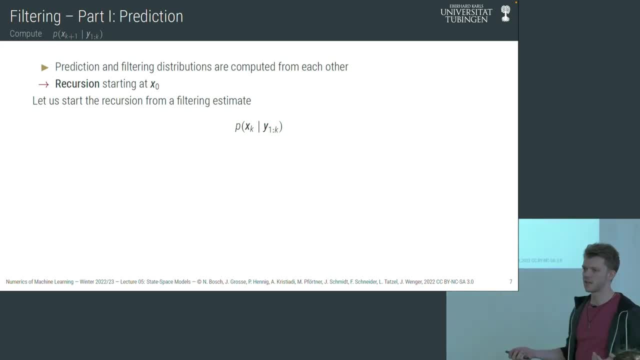 we compute one thing from the other. that's basically just saying we compute a recursive algorithm which a recursion, a recursion starting at the initial time, step x0. so we are not going to start a derivation at x0, we are. we are making this a bit more general and 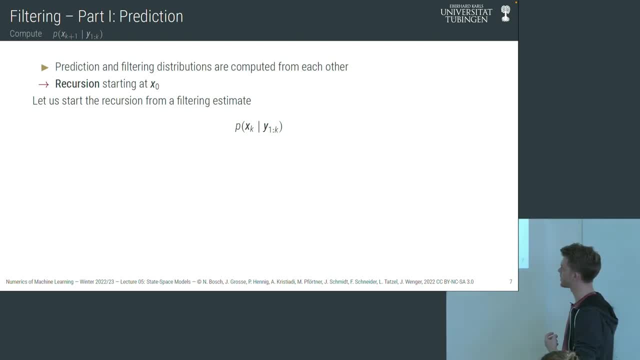 we say we are have one filtering estimate available at time- step k given all the previous data and the including one. so we have a current filtering estimate and from that we compute a prediction distribution. so how are we going to do this? and this is a recurring theme in deriving these kinds 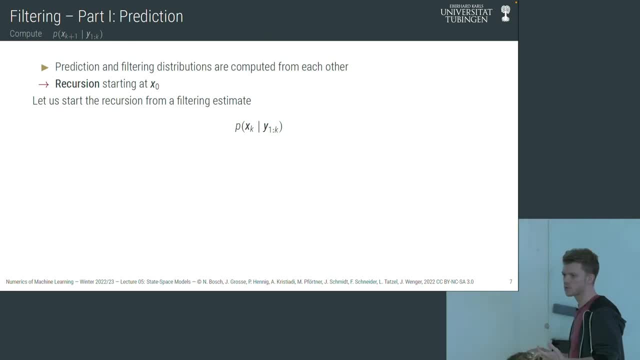 of probability distribution. you just basically introduce the quantity you care about. so from this distribution you build a joint distribution of what you already have together with the quantity you are looking for. so the joint distribution between p of x k plus 1 and x k given y 1 to k. 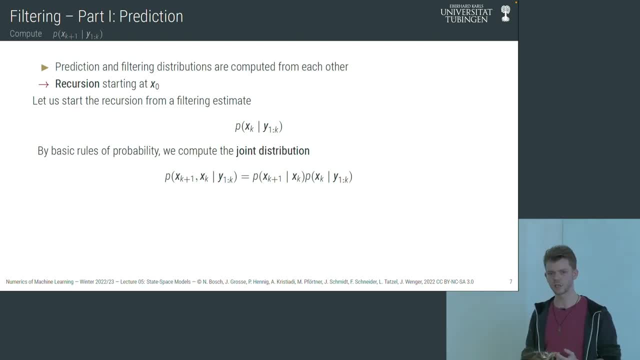 this joint distribution you can split up into the product of two conditional distributions. why do we do that? because we notice that we actually know both of these distributions. the left one is just our dynamics model as defined by the probabilistic state space model- this is given- and the right one is the previous filtering distribution we know is: 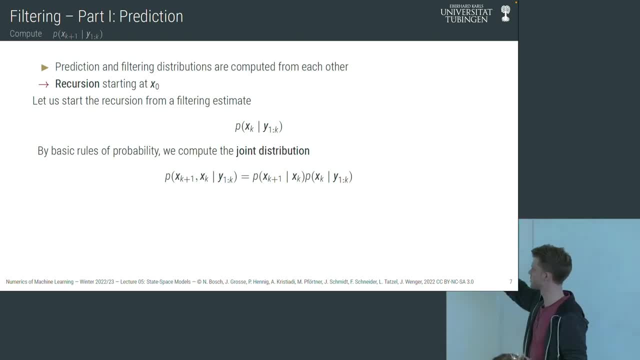 given because we assumed it's given in the very beginning. this is just p of x 0, because there's no data to be written down on the right of your conditioning bar. okay, so now we have to get rid of this x k because we really don't care about it. right, we want to compute p of x k plus 1, given y 1 to. 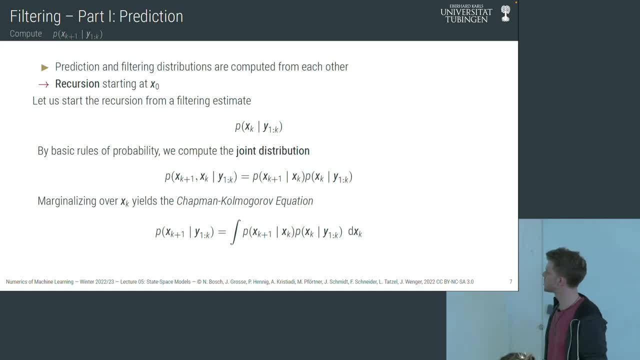 k. so what do we are we going to do? we're just going to marginalize it out using this equation: p of x k plus 1, given y 1 to k, is the integral where we integrate over x k of this product of conditional distributions, our dynamics model and our previous filtering distribution. this 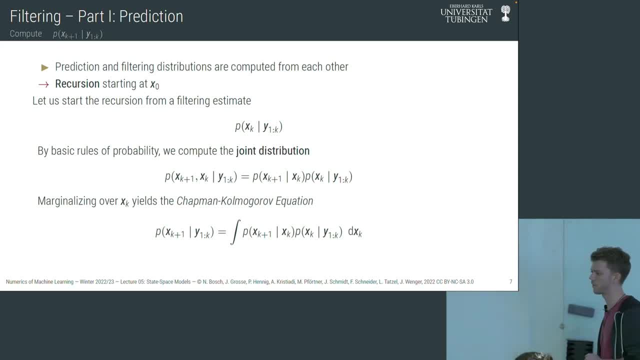 equation is so important it has a fancy name. it's called the chapman karmogorov equation usually, so this is a convention from the research field of signal processing and it's a really important equation. it gives us the possibility to predict into the future, giving past measurements. 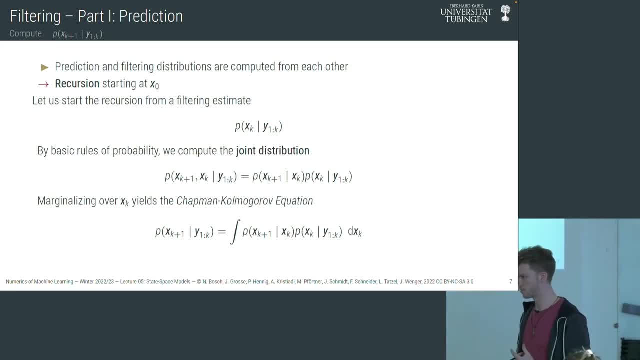 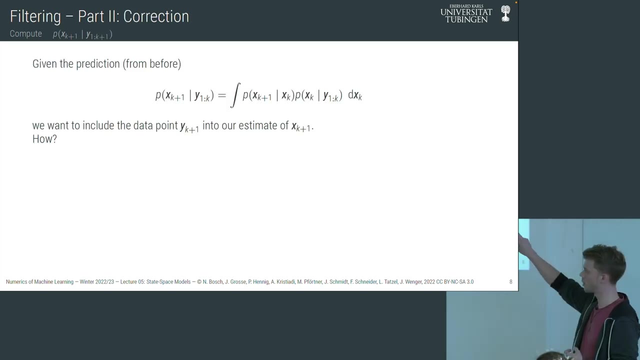 cool. so in order now to compute our filtering distribution, which was our initial goal, we have to. as soon as the new data point x, y, k plus 1 comes in, we have to have a tool to correct for this newly gained knowledge. it's called the correction step. this is just the copied over. 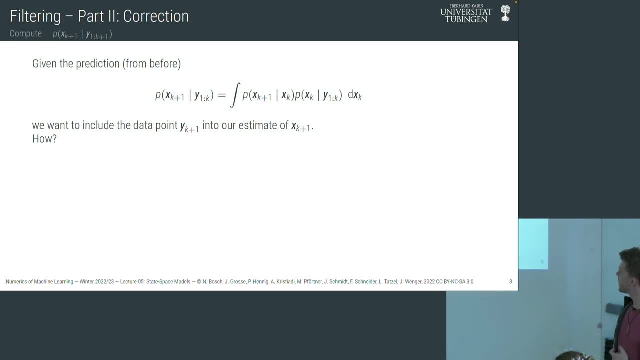 stepman karmogorov equation from the previous slide and now we have a new data point p of y k plus 1, and now we are going to integrate this into our estimate of x k plus 1.. how are we going to do? 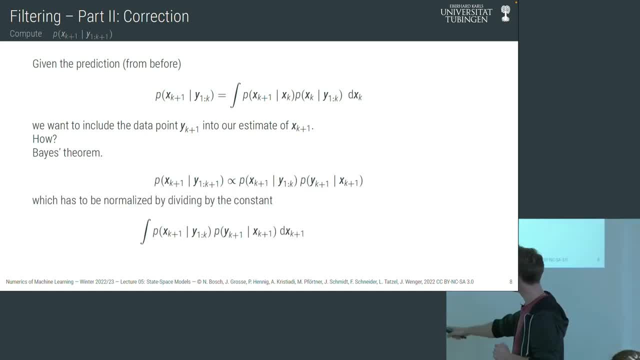 this base theorem. so we just write it down: p of x, k plus 1, so the probability of the next state, given all the data up until this state, is proportional to the product of a prior in the likelihood term. so to say, the likelihood term is easy. 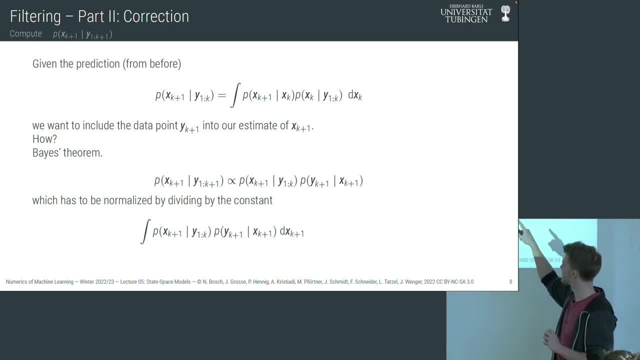 this is just given by our state space model, if you. if you see, it is the measurement model that we defined in our probabilistic state space model. the left term, which can be interpreted as the prior, is just the predicted distribution. we computed using this chapman karmogorov equation. so this: 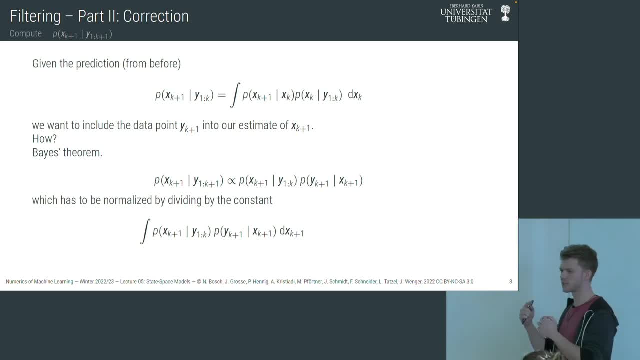 is what i meant by we compute one distribution from the other, and then we have this scheme of predicting and updating, predicting and updating and, of course, since this is a space theorem, we have to divide by a normalizing constant that we compute using this integral, which is sometimes called the evidence, in order to get a valid posterior distribution. 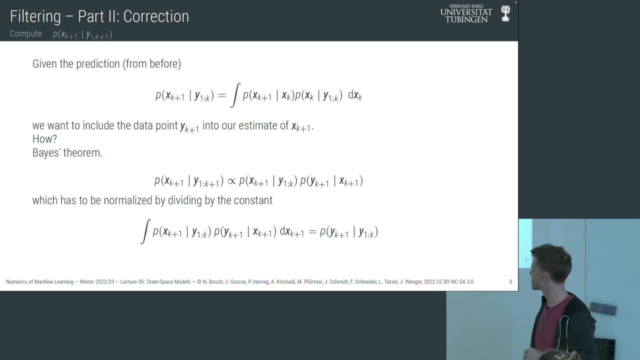 and some of you may have looked closely and noticed that this is actually this term that i phrased- data likelihood- in the beginning, so we have to compute this quantity anyway along the way. this is just the probability of observing the next data point, given the previous ones. 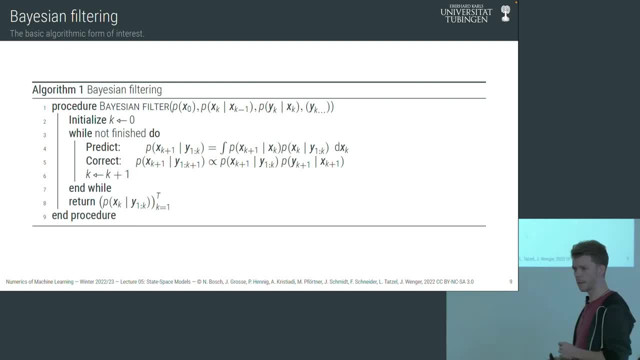 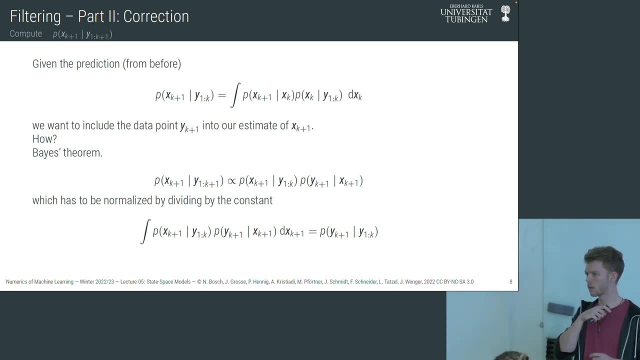 okay, cool, in order to put some structure into this. yes, now we assume that every y has an observation. yes, um, i told you earlier that this doesn't have to be the case. i just use this convention, if you will, such that not too many indices are flying around, because then i would have to. 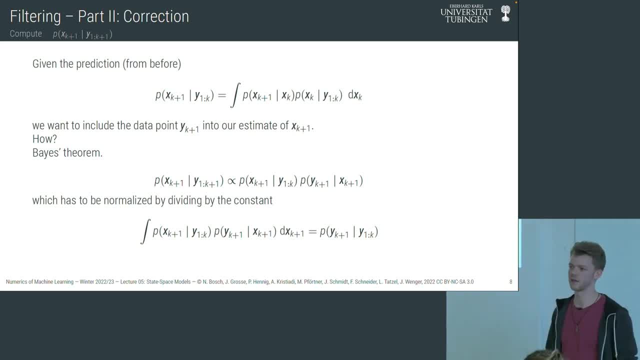 use a different index for n and a different index for x, so it makes everything a bit more confusing and hard to look at, but you don't have to have a measurement for every state that you want in order to be able to predict the model. okay, so then? 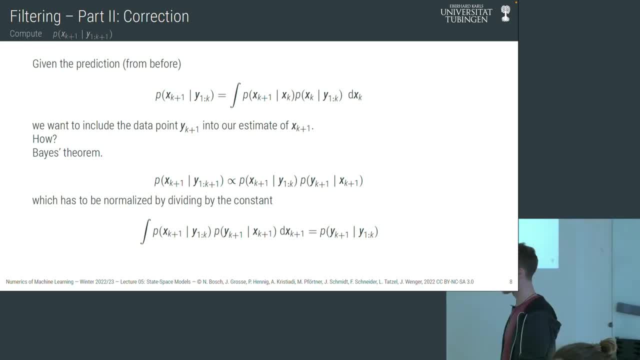 instead of doing the one step in x, you would do multiple steps exactly. actually, we are going to see this later on, but i just basically neglect this here a little bit because, yeah, the algorithm is usually phrased in a way that you don't predict between measurements. but 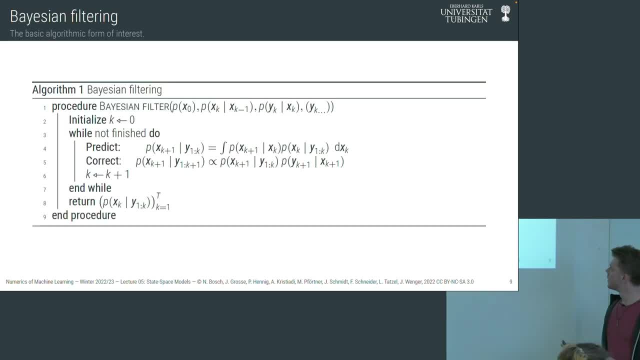 we are going to see this later, thanks, okay, let's give this a little bit of structure. so in form of pseudocode- because this is actually a bayesian filtering algorithm in its general form- we start at the time step zero, and then we enter this y loop. this is not a for loop, because we 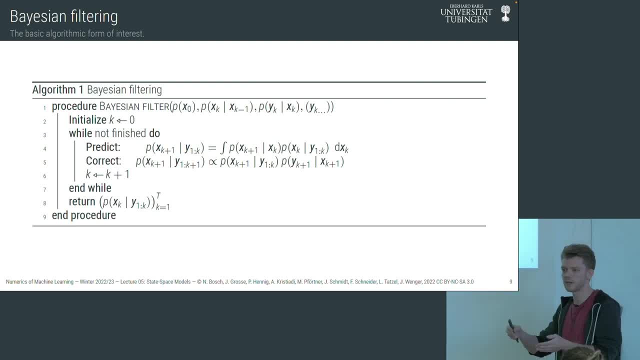 don't have a finished data set or a fixed data set, because new observations could trickle in at any time. right, and we just predict up until the next step using the chapman chromography equation and we correct using bayes theorem, these two equations you just saw. these are the prediction and 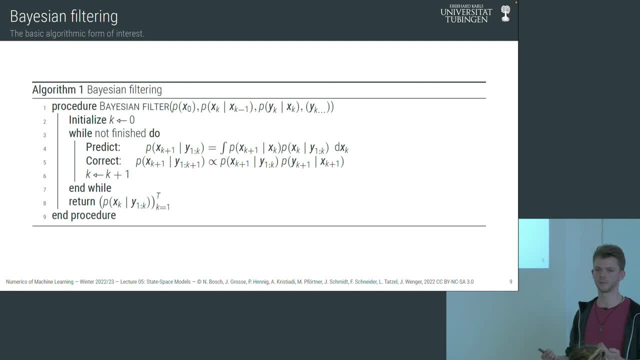 correction equations. we increase our time step and go on and so on. notice that we never go backwards in this algorithm. as soon as we see the next data point, we don't update our previous state estimates, even though we could give provide them with more information. but we are still in this online estimation setting. we want to be quick with. 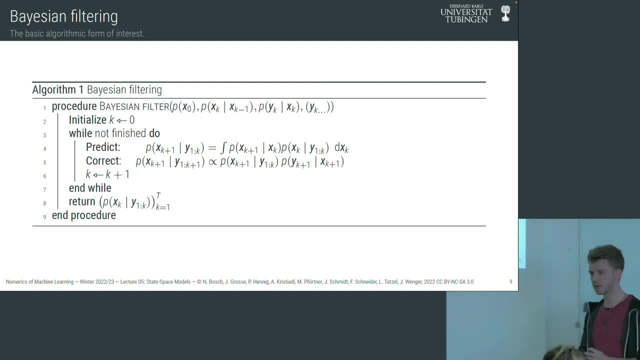 our estimates and our most recent state always saw all previous measurement, so we can't get better than this. but we we have one linear time loop here and if we decide at one point that we stop our state estimation algorithm- we can't get better than this- we just return this sequence of distributions, of filtering distributions. 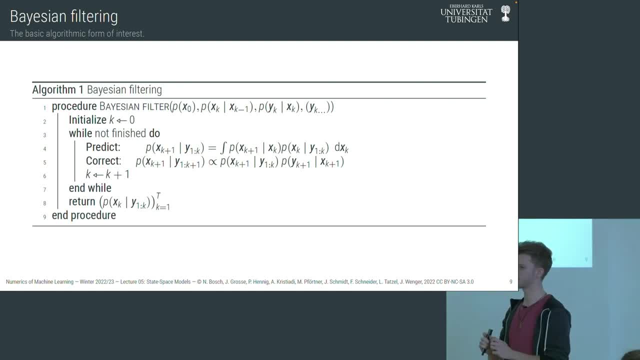 the distributions over the current state, given all the previous measurements. i say this so often because it's very important. okay, what i didn't show you yet is how to actually compute those things right, because there are integrals flying around there and there's also an integral hidden in this proportional sign. 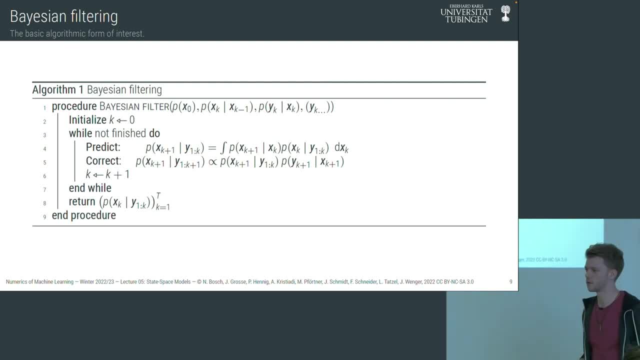 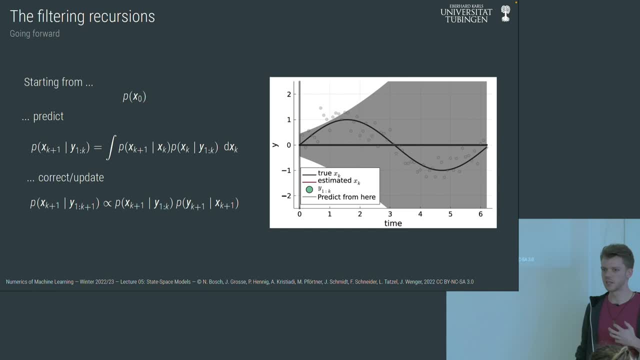 so, and we don't even know what our model is yet, so we cannot really compute anything with that. it's just a general collection of formulas. so we can't compute anything with that. it's just a general collection, formulas. And the next step I'm going to take is actually build a model that can produce plots. 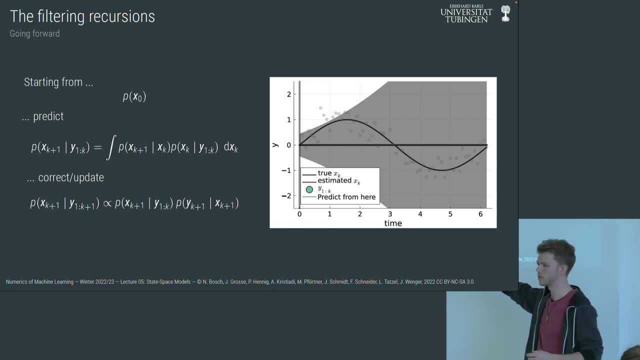 like this, where you see here on the right-hand side of this vertical bar denoting our time step k, our current time step, currently being at zero. The right-hand side is the prediction. The left-hand side is then the filtering estimate, which is currently not visible. I have not told you so. 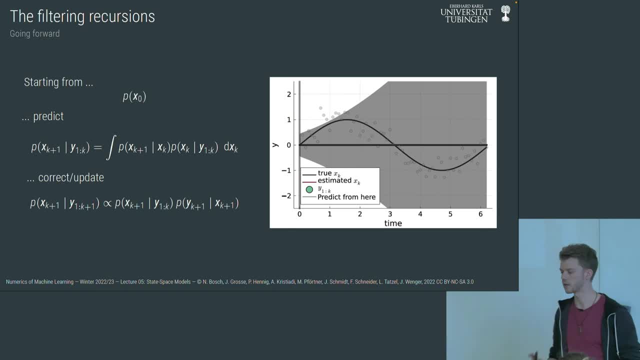 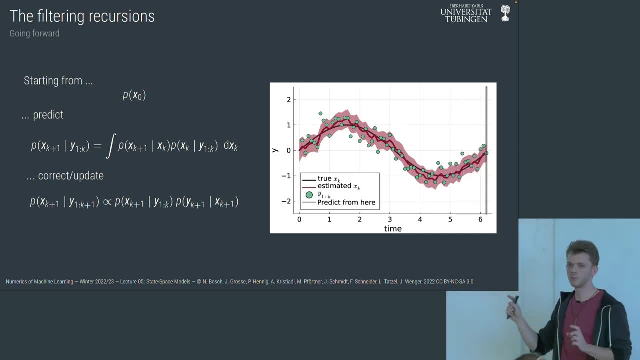 far how to produce this plot, but I'm going to tell you on the next slide, And this is roughly what it's going to look like. You see here, always on the right-hand side, the prediction into the future. You would not compute this prediction normally, because it's just not really informative. 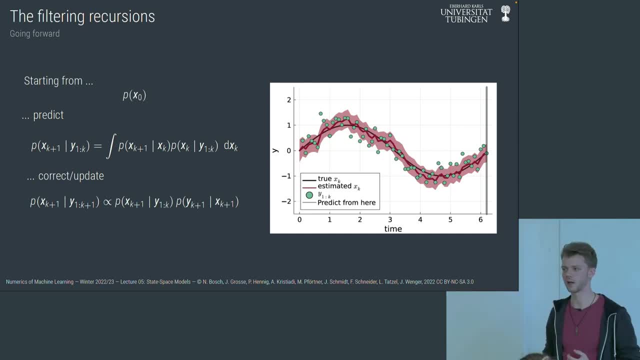 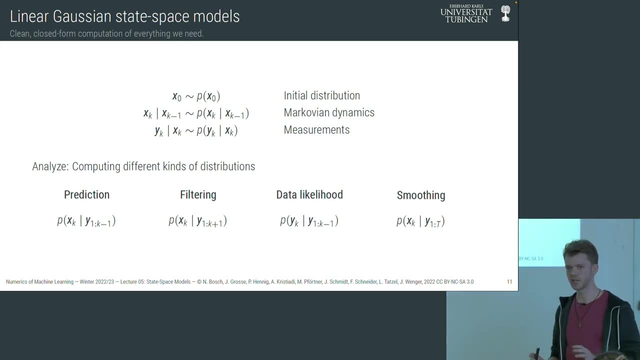 This is just for visual reasons, such that you can look at how these predictions could look like under a certain assumption of a model which we are now going to look at. Okay, back to our general setting. We have our state space model, We have those distributions. We want to compute. We cannot. 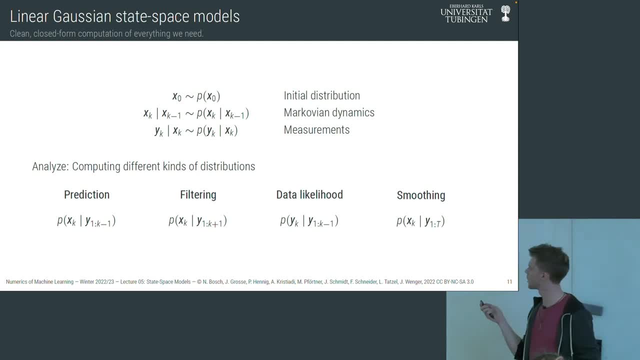 compute yet because we don't know what our model is. So let's insert actual models into this, And we are going to choose Gaussian, a linear Gaussian state space model. We're going to start off with an initial Gaussian distribution distributed according to some mean mu zero. 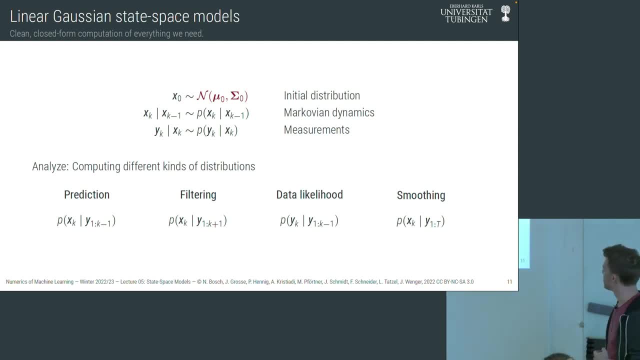 and a covariance metric sigma zero. And now it gets really interesting because we are going to consider linear transformations of the previous state to get a distribution over our next state. So xk, given xk minus one, is a Gaussian distribution that arises from a linear transformation of our 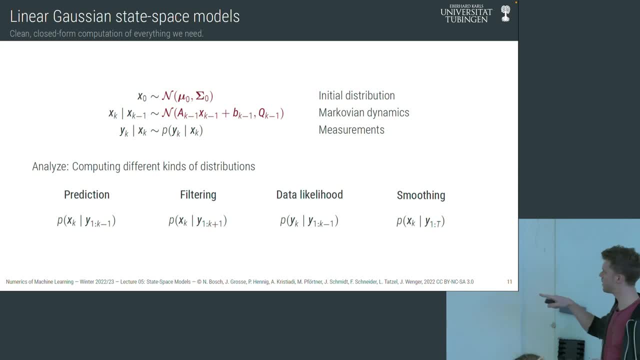 previous state. I say linear because I don't want to use a linear transformation of our previous state. So linear it's actually affine. We have this plus b here. But anyway, I would confuse it so much that I just stick to linear now. But I mean affine when I say linear because it's more general than 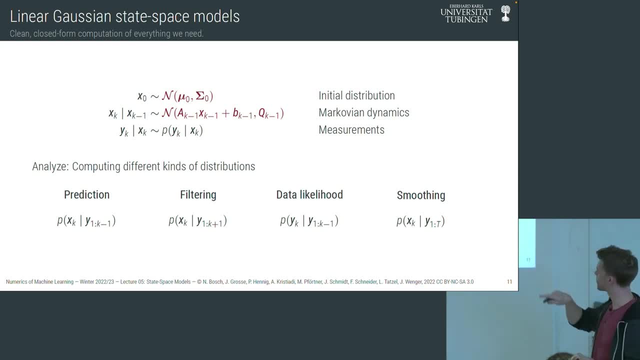 that Under a additive Gaussian process noise given by this covariance matrix Q. These two matrices have names: A is called the transition matrix and Q is called the process noise covariance matrix And I will call them that in the remainder of the lecture. It's just a convention from 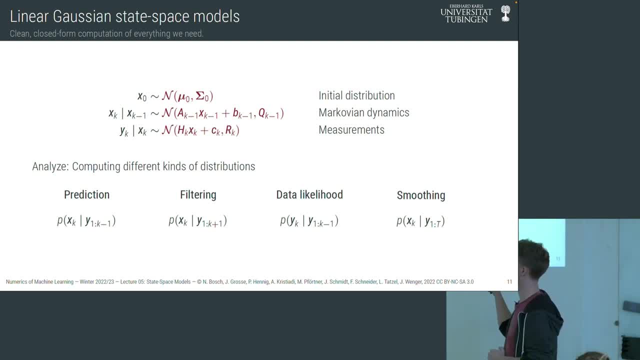 processing And we are going to choose the same kind of model for our measurements as well. We are going to consider linear Gaussian models. We have this measurement matrix H and this measurement covariance matrix R, And this is our state space model we are going to choose- Most of you probably- 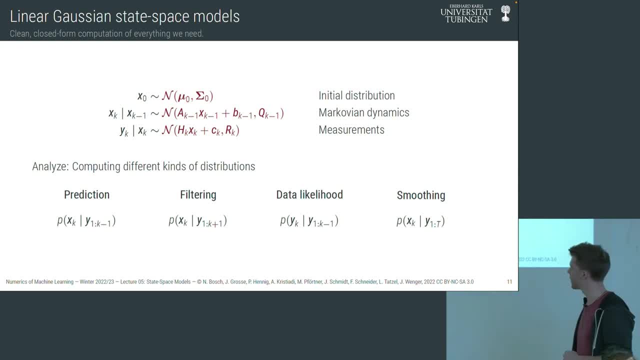 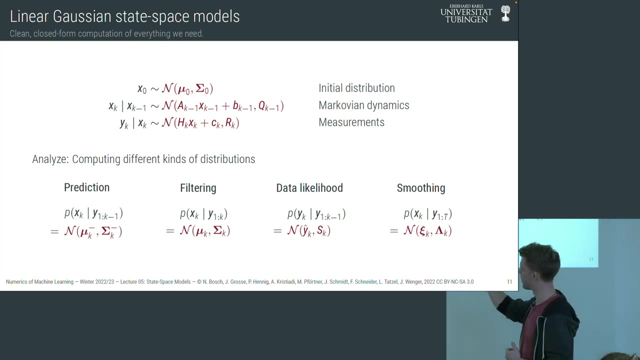 know why we are going to choose this kind of model? Because linear transformation of a Gaussian random variable is a Gaussian random variable And you could think that all those distributions then are also Gaussian random variables. We are going to call the prediction moments denoted with the superscript minus. We have this: 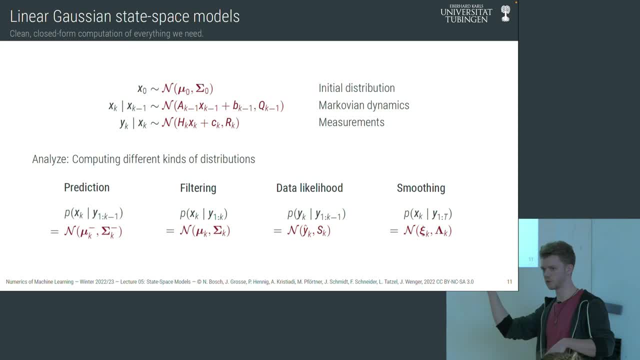 filtering moments mu k and sigma k. This data likelihood is computed along the way, And later on we are also going to see that the smoothing distribution is actually also Gaussian. So this is quite convenient. How do we know this? We know it by Gaussian inference, By the theorem of Gaussian. 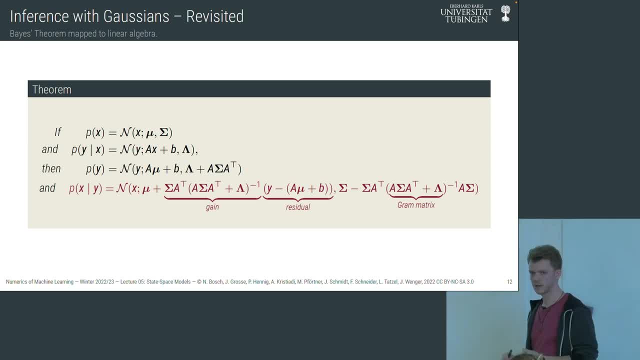 inference. You already saw this, probably more than once, And I think also that all of you understood this. Otherwise you would have had trouble to understand the previous three lectures, because Gaussian process is really built on this theorem. But I want to read it out very quickly again. 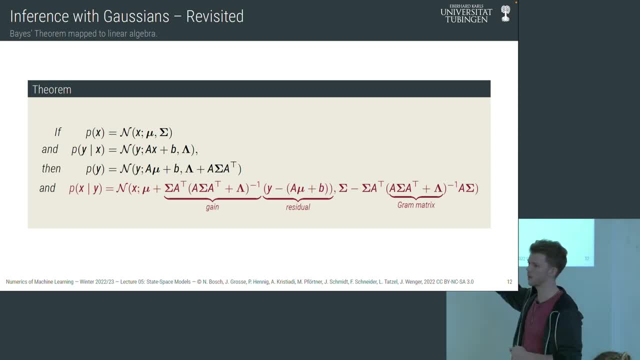 because later on I want you to recognize these terms again in our algorithm. If we have a Gaussian distributed random variable, X, distributed according to some mean and covariance matrix, and we have an affine transformation of that and we have this p of y given x as a random variable, with this affine transformation of x, then we can compute p of y, which is a Gaussian. 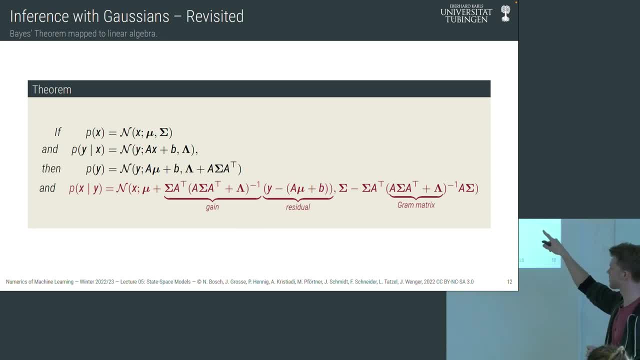 but I'm not really interested in that right now. What I'm interested in is this posterior distribution p of x given y, And it's this really complicated collection of terms that you probably all saw. We see here that we add to our prior mean this product of this gain term times this: 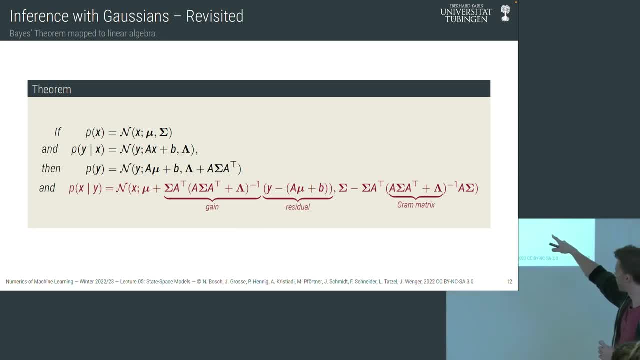 residual term And we have here for our posterior covariance. we subtract from the prior covariance this product of sigma times a transpose times this gram matrix and then, from the right hand side, again multiply this a sigma to this gram matrix. Okay, so if you keep now these terms, that 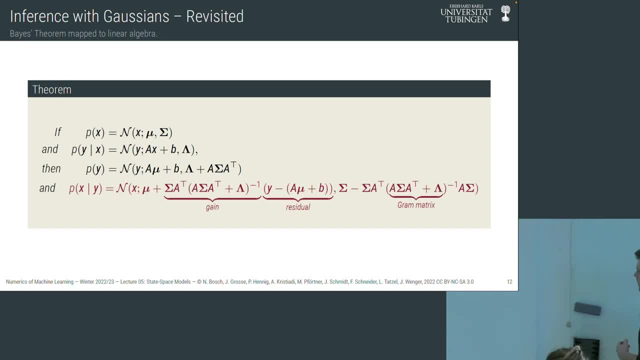 I labeled here in mind. we can proceed now to an algorithm that allows us to compute the prediction and filtering moments, given our linear Gaussian state space model in closed form, just using Gaussian inference- And this is actually a name which most of you might have already heard. It's: 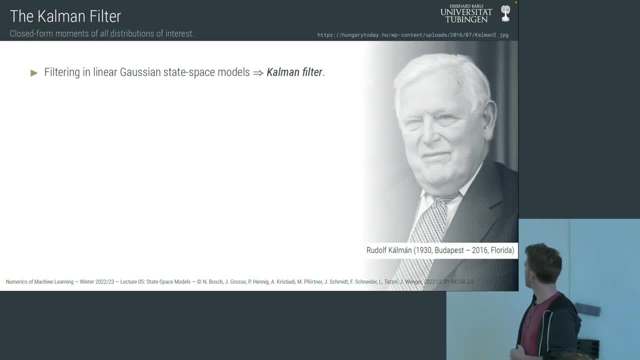 called the Kalman filter. It is named after the scientist, Rudolf Kalman. It's a Hungarian researcher. He was a Hungarian researcher. He died in 2016 and he is the person who gave this algorithm, this very useful algorithm, its name. This algorithm just allows us, as I already said, to compute prediction filtering. 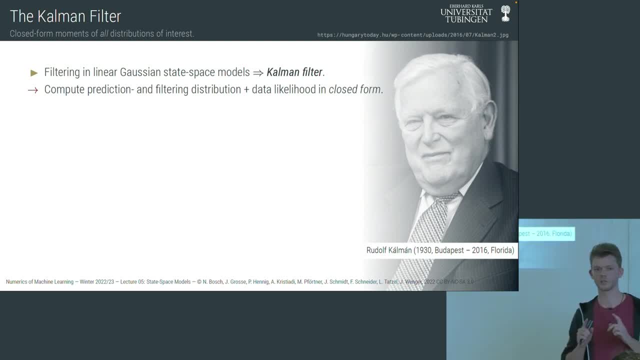 distribution in closed form, And I'm not going to derive this here, because I want you guys to derive this in your homework sheets by inserting our linear state space model, Gaussian state space model, into our prediction and filtering equations. I'm just going to show you. 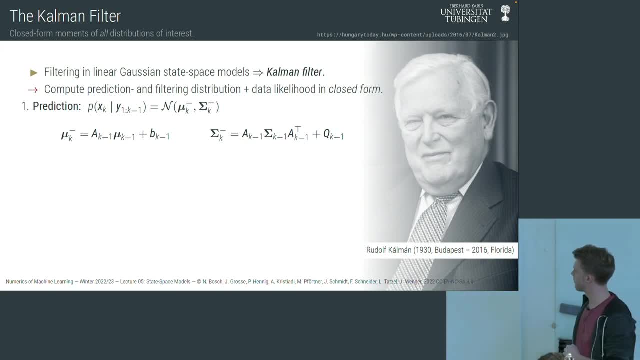 these equations here. So the prediction equations are given by these two things. So we have to compute the predicted mean, and this is just a linear transformation or the affine transformation of the previous filtering mean. This is quite easy, right For the predicted covariance matrix. 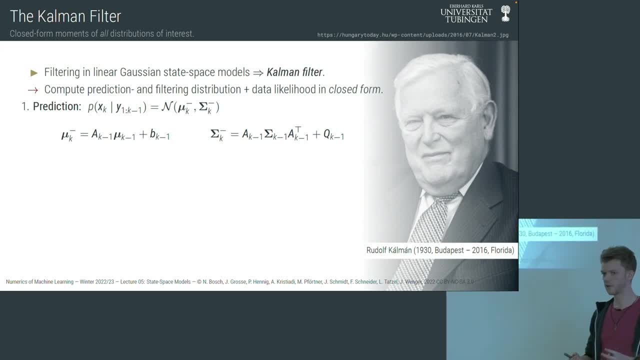 we just multiply the previous filtering covariance from the left and the right with the transition matrix and we add the process noise covariance matrix to the previous filtering covariance matrix. So quickly we have computed our predicted moments For the correction. you will probably recognize terms from the previous slide. We first compute this measured predicted mean. 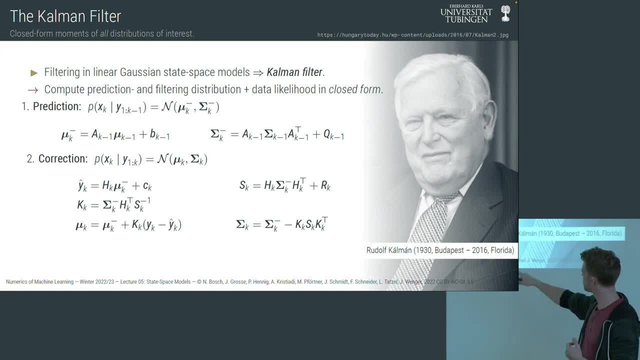 so to say, and save it in this variable y hat. We compute this matrix S as the measurement matrix times the predicted covariance matrix times the transpose measurement matrix and add this measurement matrix R. Then we compute this matrix K As the predicted covariance times the transpose measurement matrix times the inverse of this. 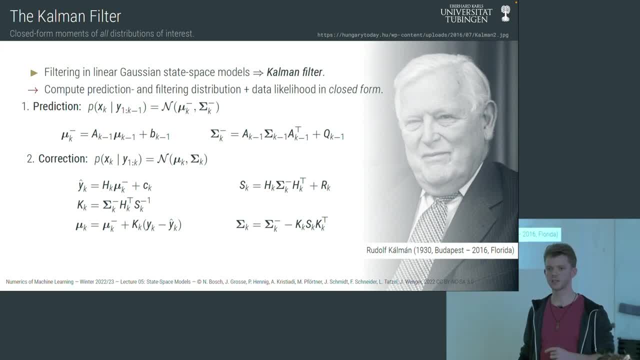 matrix S And this is a very important quantity. It's called the Kalman gain. If you remember gain from the previous slide, you will see that the structure is actually very similar And the gain kind of. so it has a meaning. It kind of translates from your measurement. 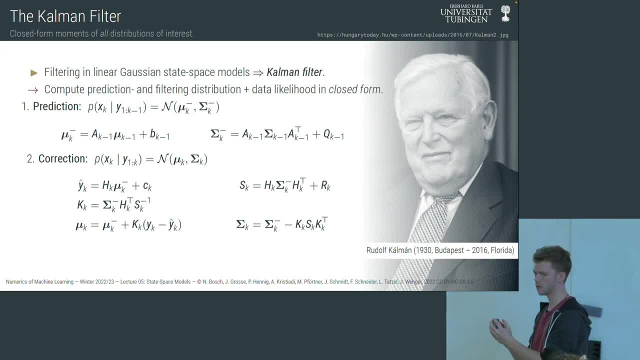 space to your state space, Kind of maps the information that you gained in your measurement space and maps it onto the state space And therefore we use it to update our filtering mean by multiplying this Kalman gain matrix with our residual term, where we just subtract from the data point our measured predicted mean. 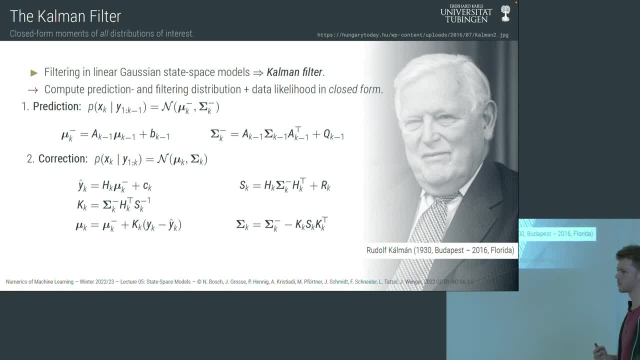 So basically, the difference between what we really observed and what we would have predicted to observe And the filtering covariance matrix is then just the prior covariance matrix or the predicted covariance matrix, minus the Kalman gain multiplied from the left and right to this Gramian matrix S. 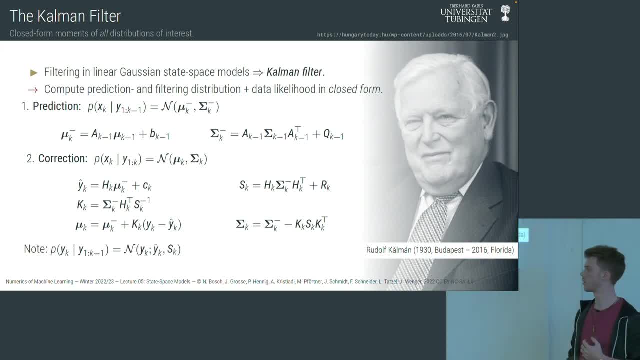 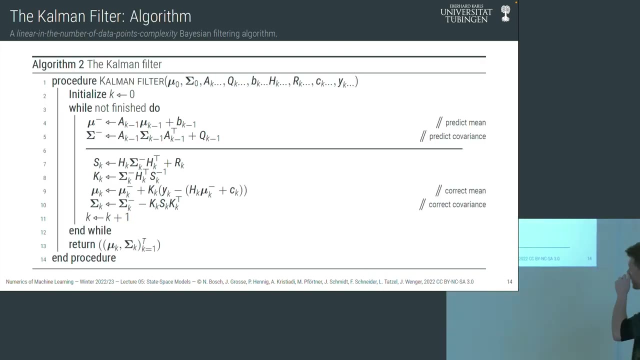 And actually along the way, we did already compute this data likelihood term, which is also Gaussian, And the mean is just given by this measured prediction And the covariance is given by this Gramian matrix S, And that's the Kalman filter equations. We can write this now down into this algorithm. 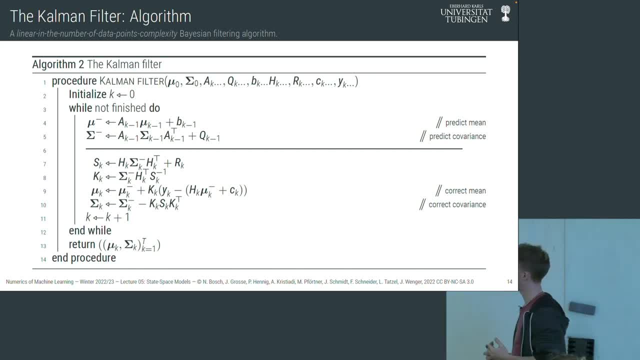 where we just basically have the exact same structure with as we had with our Bayesian filtering algorithm, But now we can compute these distributions and actually we can compute them in closed form. We have again this Y loop And we compute our predicted moments and our corrected moments according to the equations. 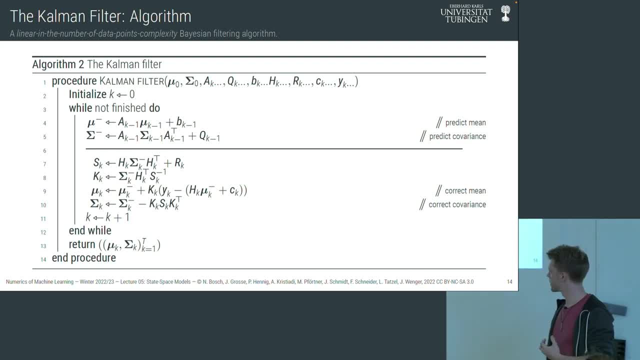 you saw before, and in the end we just return a sequence of means and covariances that completely specify your filtering trajectory, which is just a collection of Gaussian random variables. And again I want to highlight this again- this is only ever informed of the previous. 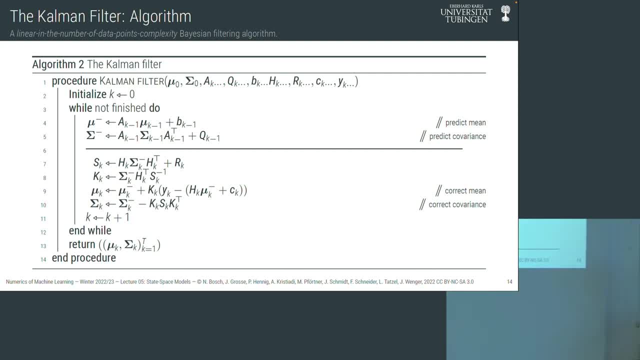 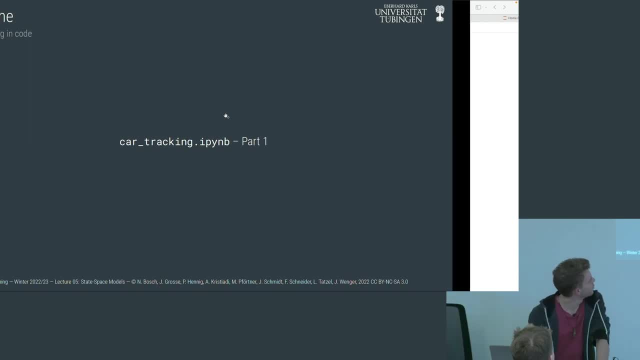 and present data points, not of the future. Okay, Now I'm going to do something risky. I'm actually going to show you code, so let's see if this works. as the name already suggests, we're going to look at a car tracking. 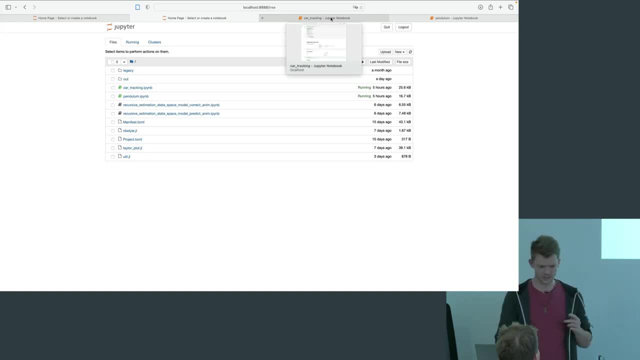 example in practice. so the setting is: we have a car going from its start position to its destination in an xy plane. so of course cars are moving in a three dimensional space, but we neglect the third dimension. just basically imagine a map, a trajectory drawn on a map. 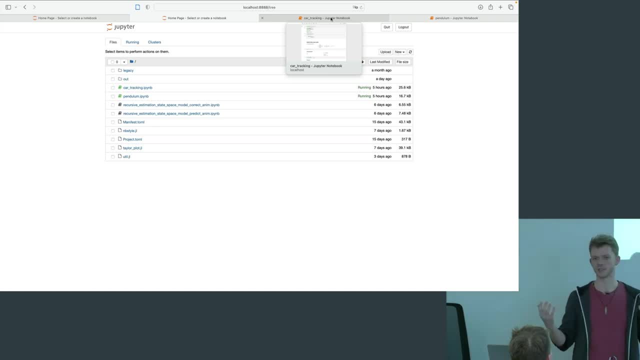 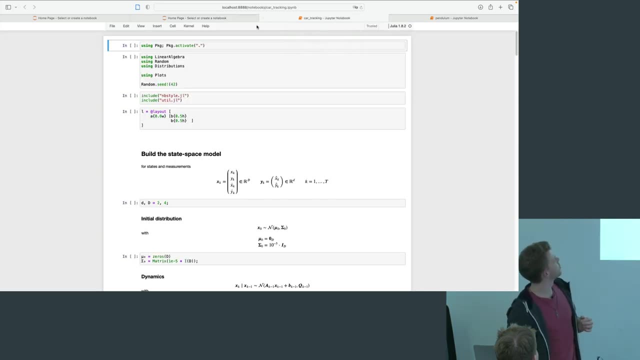 and we want to, based on noisy measurements, so, for example, GPS measurements of this car. we want to find the true trajectory, and all we have to do for that is open this notebook, quickly realize that we are not staring at Python code. this is actually Julia code, so 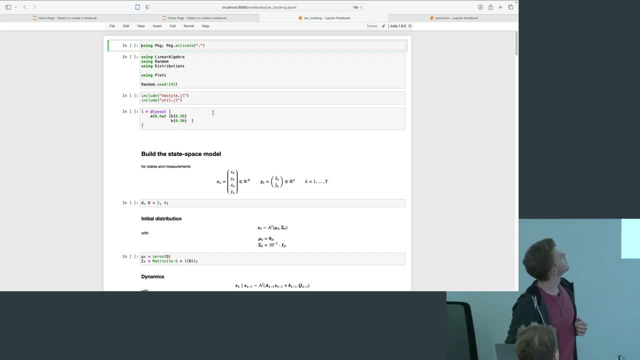 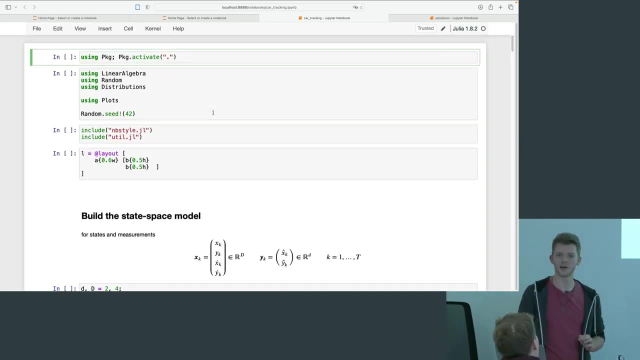 larger. let's see. yes, thank you. I hope everybody can read this nice. anyway, we're looking at it's Julia code. this is not Python code. I have no special intentions. I don't want to advertise Julia or anything, it's just maybe it's interesting for you to see. I'm using Julia myself in my PhD. it's a. 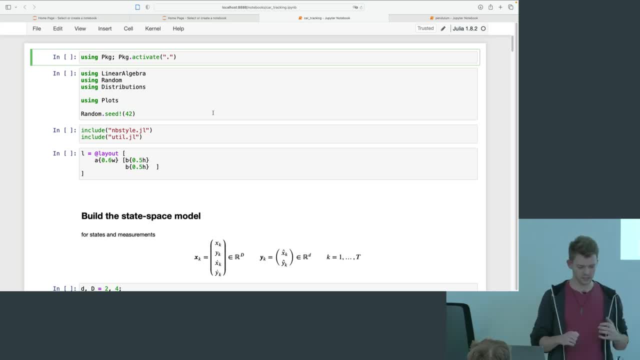 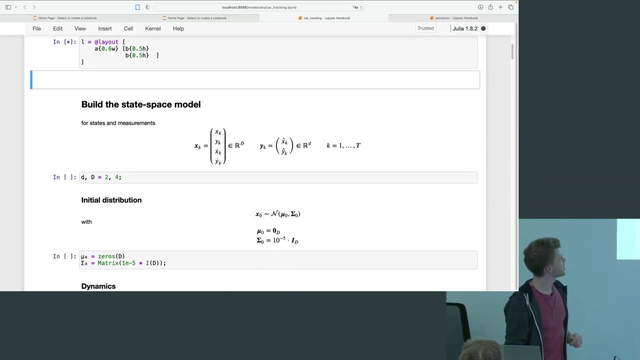 quite nice and emergent programming language, but of course it has its advantages and disadvantages. so if you want to use Python in your homework, please do so. it's completely fine. okay, this is just some setup we actually don't need. we have to begin by setting up our state space model. 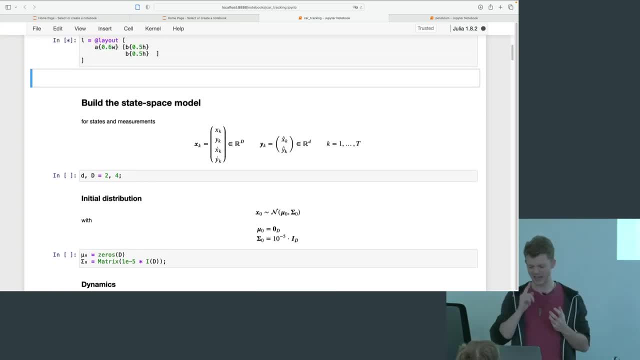 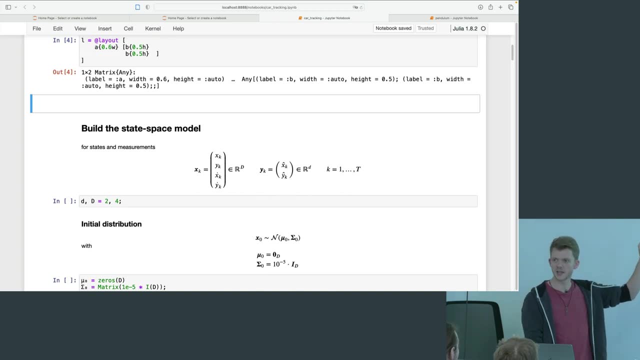 okay, so this is just some setup we actually don't need. we have to begin by setting up our state space model. okay, remember, we have this car tracking example here. right? so the state is going to consist of four components: x and y position and x and y velocity. the velocity is respectively denoted with this dot. 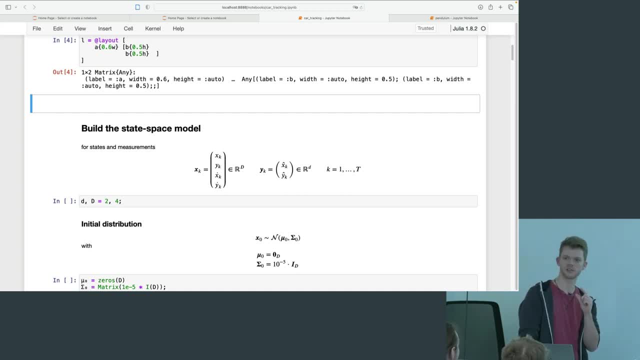 and we're only ever going to measure the first two components of the state vector. we're only going to get GPS measurements, instant measurements of the position. this might be completely different in practice, but this is just how it how it is for this example. okay, this is our state. 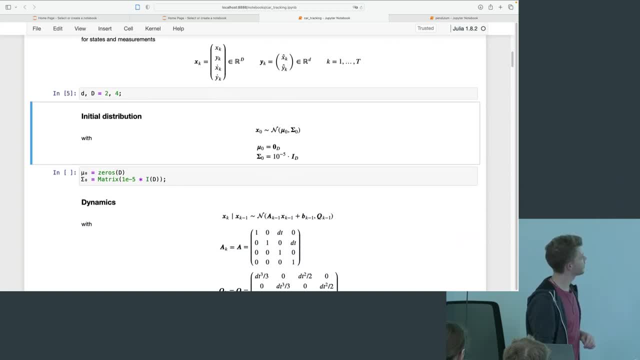 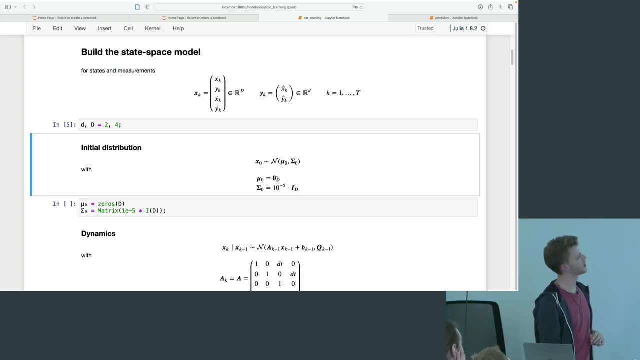 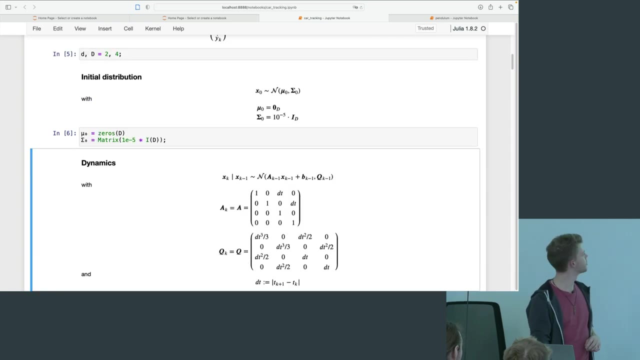 we have a measurement dimension and state dimension of two and four respectively. we are going to initialize this with a Gaussian distribution with mu zero and sigma zero, mu zero just being the zero vector in four dimensions. sigma zero is just a scale identity matrix. okay, we're going to write this down. execute the cell. cool, so far, so easy. 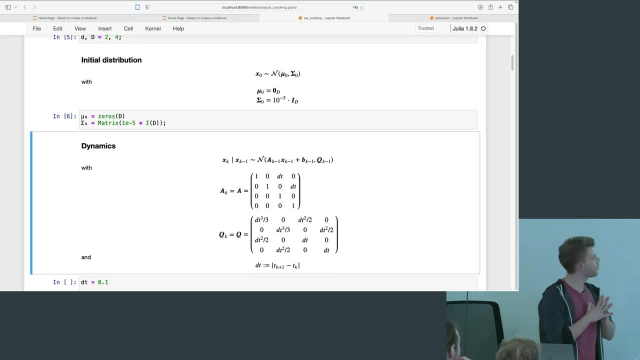 right now it gets complicated. we have now our dynamics model. it is a linear Gaussian model, as we already said, because then we can do Kalman filtering. we are going to to assume that our matrix A doesn't change over time, so it's constant. but it's quite complicated, right. 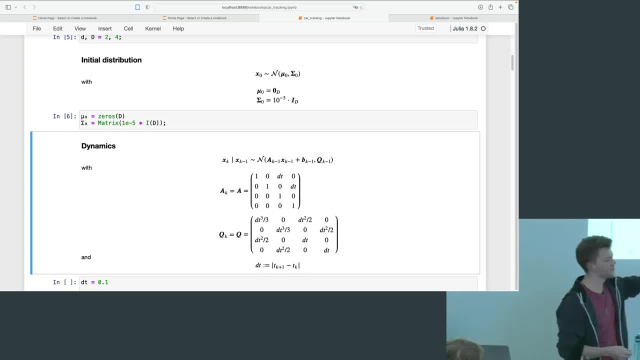 So, okay, maybe A is not as complicated as the process noise covariance we are gonna talk about in a minute. It's just this thing with ones on its diagonal and something that involves DT on its off-diagonal. DT is just as the name already suggests. 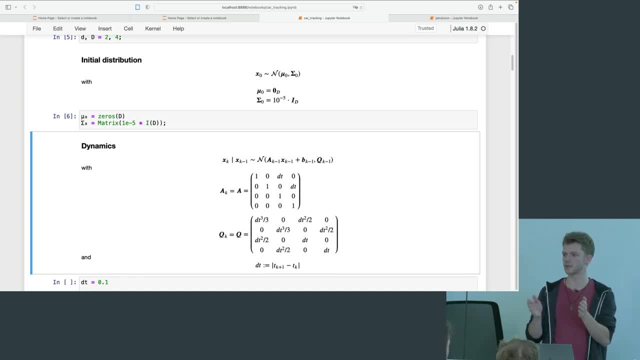 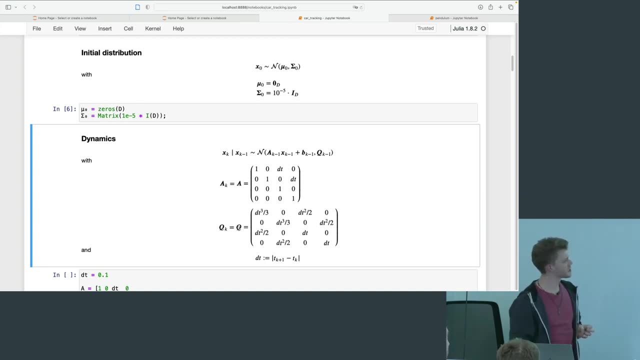 it's the time step. so the difference in time between two subsequent steps, k and k, plus one as I wrote down here, And q, you can see, has an interesting structure and also involves kind of polynomial terms of this DT somehow, and I'm actually not going. 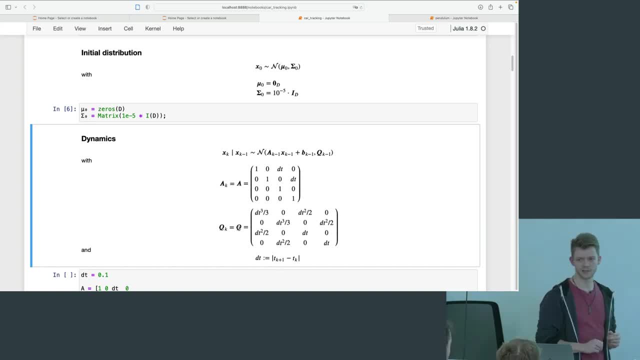 to tell you why, because it's very complicated. It, roughly speaking, arises from the discretization of a continuous stochastic model, a stochastic differential equation, and these objects are really complicated to study and we don't have the time to discuss them here. 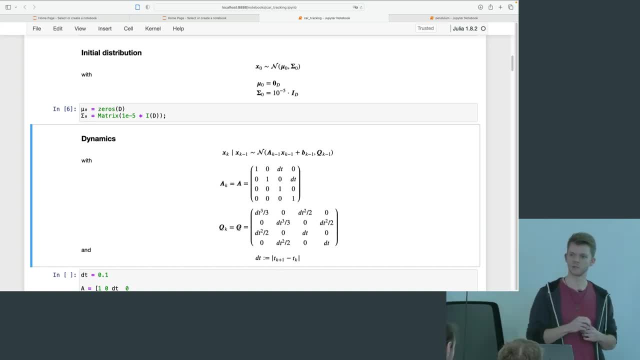 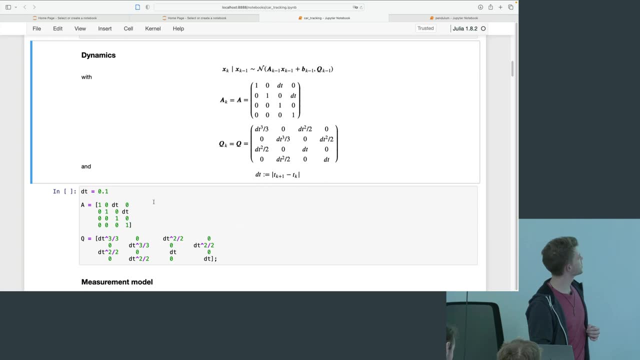 but you recognize that it has some structure and you just have to believe me that it makes sense to use the state-space model. Okay, cool, We can actually just translate this to code. We say our time step in between two subsequent k and k plus one is 0.1, and we just write down. 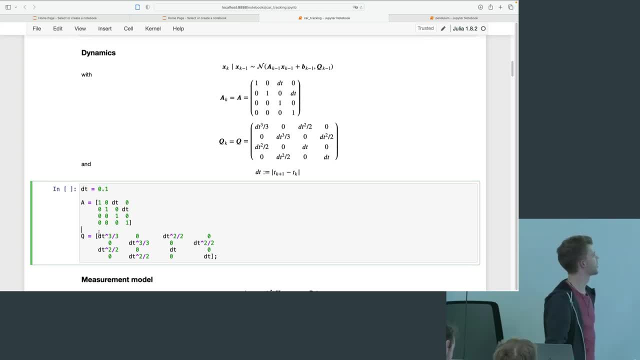 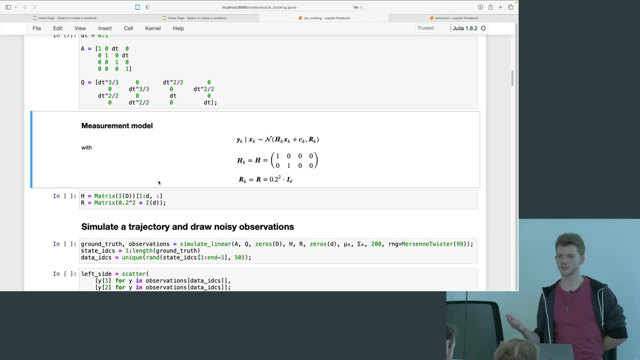 this matrix, these matrices transition matrix and process noise covariance matrix A and q. Okay, as for our measurement model, as I already said, we just measured the two first components of our state vector, so we have this projection matrix h. here is our measurement matrix. 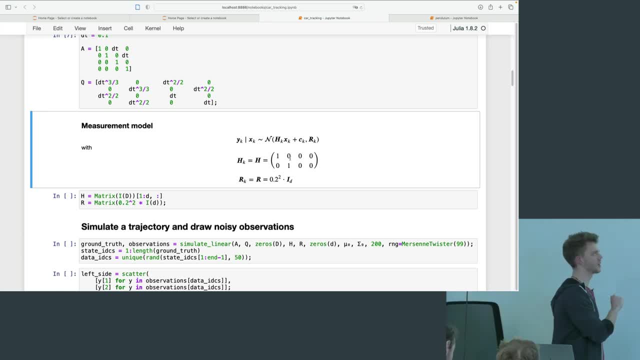 It just selects basically x position at x velocity and oh x position and y position from the state vector, and the measurement noise covariance matrix is just the scaled identity matrix again. Okay, So far, so easy. Let's execute this. 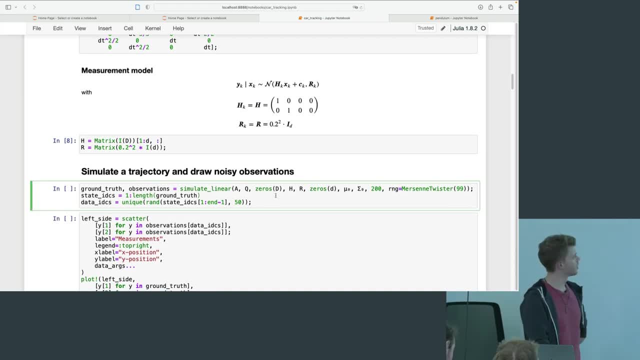 What we're going to do. what we are going to do next, is we simulate this dynamical system. once We are going to draw a trajectory from these dynamics and we are going to draw bunch of measurements from this trajectory, that is going to give us our 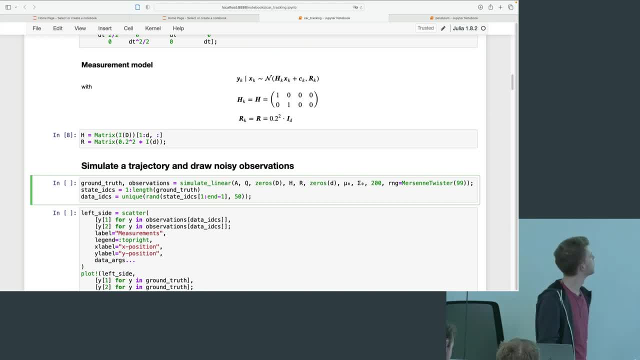 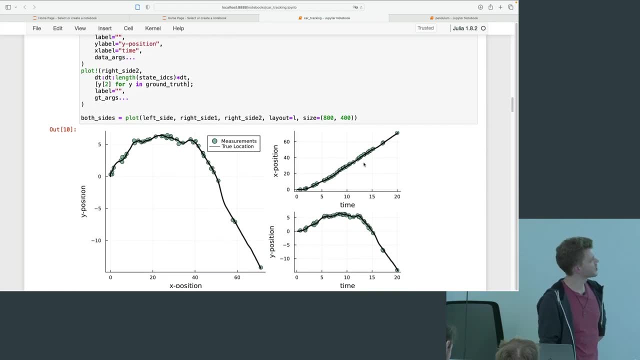 ground truth and our observations on which we make inference later on, And we can visualize them Just a second. So here we have the time series plots here on the right, So we have the x position over time and the y position over time And we 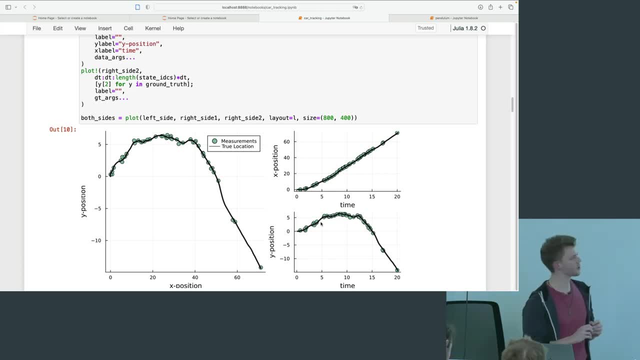 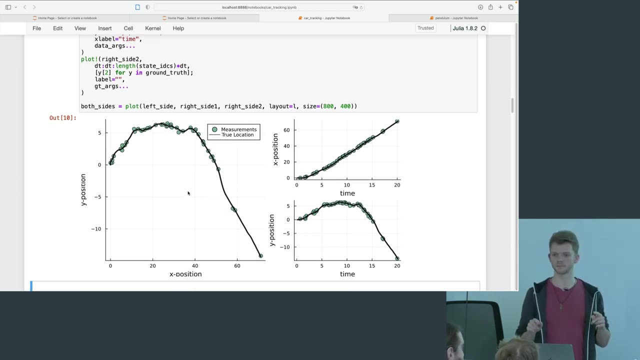 see that we have not equally spaced measurements over time. These I chose random from the sequence of measurements Because these two plots are a little bit hard to interpret. I always plot this trajectory of the car left from these two plots in the xy plane. So basically the car starts here and then drives around. 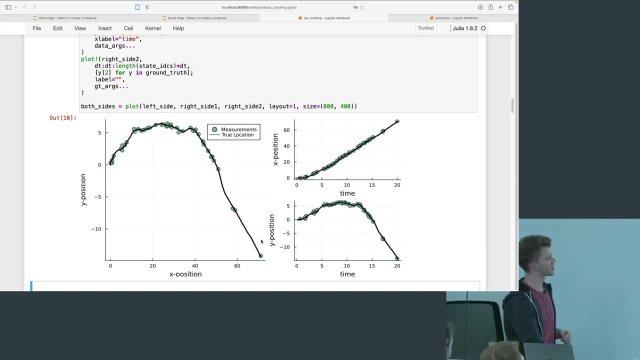 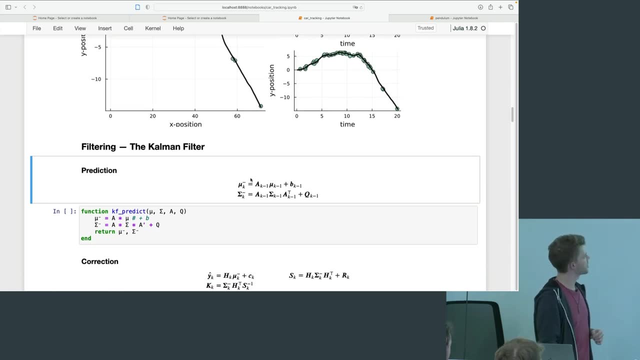 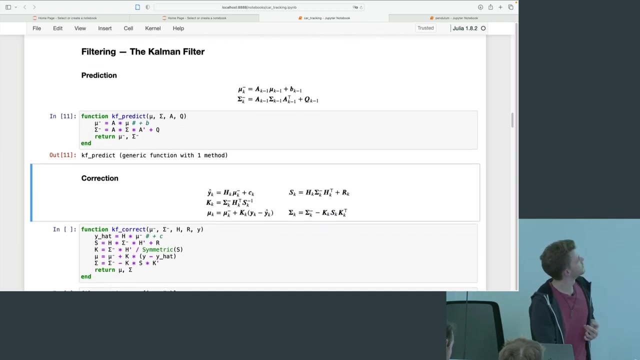 this trajectory and reaches its destination here. So now what we're going to do is implement our Kalman filter, First the prediction step, and it basically compares the two plots. So we have the xy plane and the xy plane And we have the sets of measurements, And then we're going to apply these to our 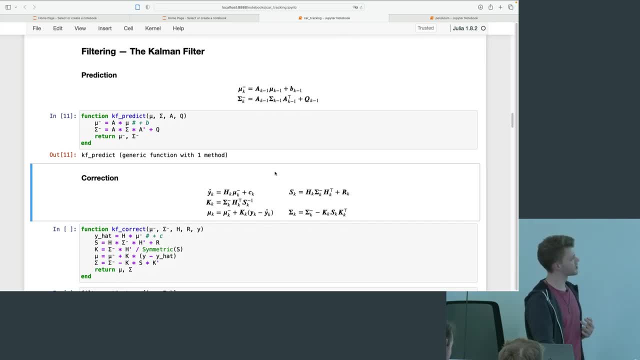 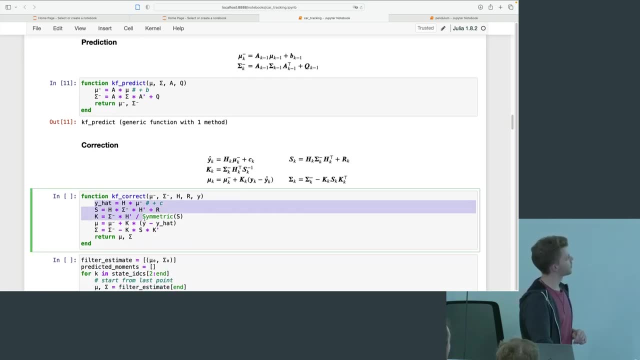 query, And then we're going to do the same for the correction. We have all these terms that we already saw. You saw them in two slides already, So I'm not going to detail them any more, Just to show you. we translate them here into Julia. 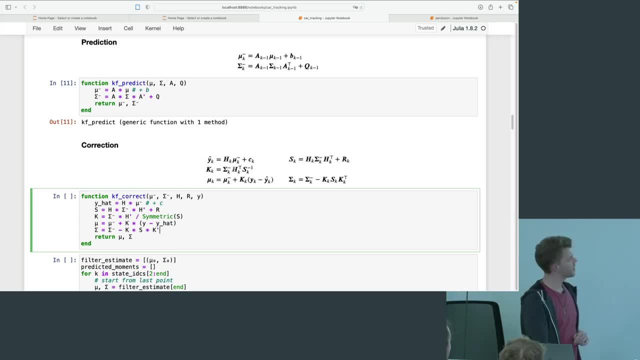 code. Notice that this matrix K involves the inversion of a matrix, And this we learned in the second lecture given by Marvin. we don't do What I do, instead, because I'm lazy and Julia is awesome, I tell Julia, our matrix S has structure, It is symmetric, And then I can just use this. 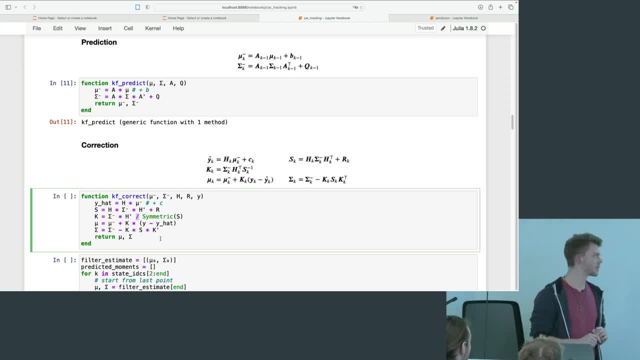 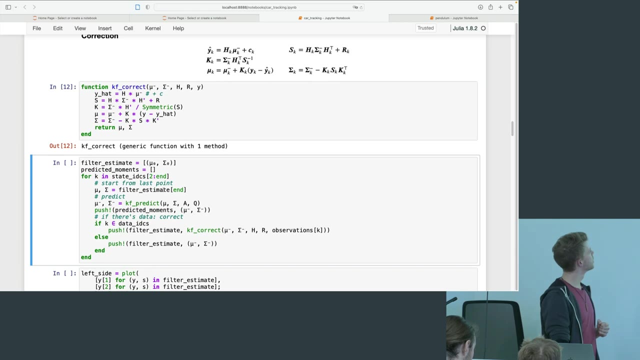 divide by operator and Julia does a fancy matrix decomposition intrinsically and solves the linear system instead. So don't use inverses. This is our Kalman filter correct function. And now I just wrote down the loop that we saw in our pseudocode. I start off with: I initialize a list with our 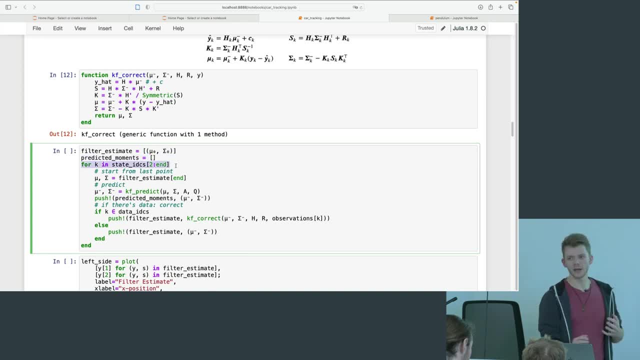 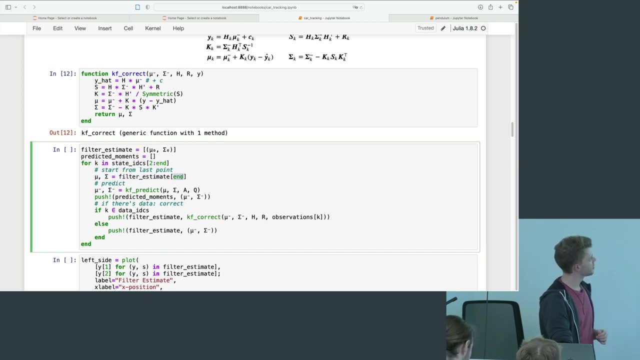 initial moments. I enter this for loop. It's not a while loop here, because then we would sit here in two weeks and wait until it finishes. This is not really interesting. I take from the end of my current estimate our current filtering estimate- I use this- and our dynamics. 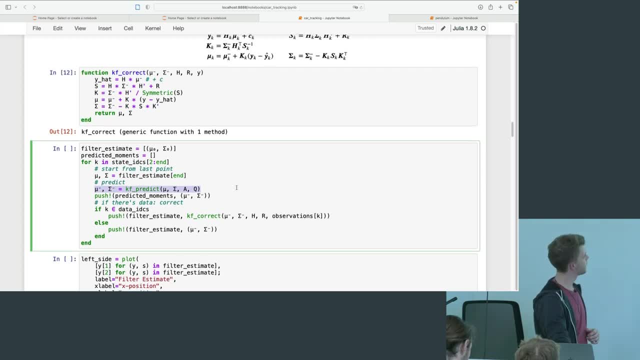 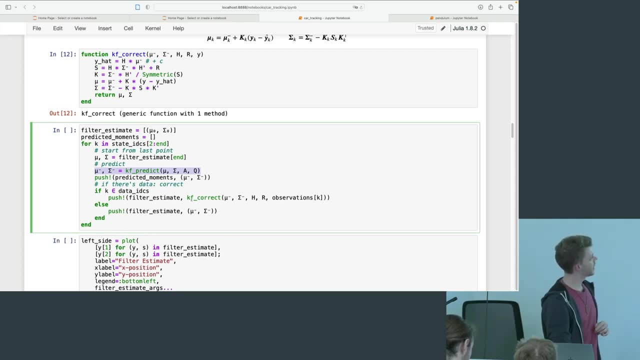 model And I take from the end of my current estimate our current filtering estimate. I use this and our dynamics model to predict the predicted mean and covariance. And then here's the twist, and this is related to the question you heard earlier: If there is data, I use the correct. 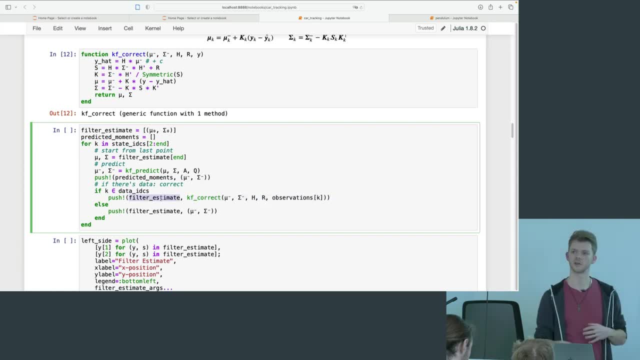 function and save the filtering estimate to our filter estimate. So the filtered moments, the corrected moments, If there's no data, I'm still going to save something. I'm just going to save the predicted moments just in order for you to see what happens in between measurements. 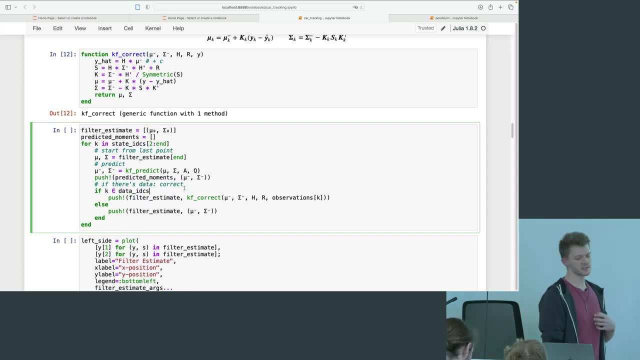 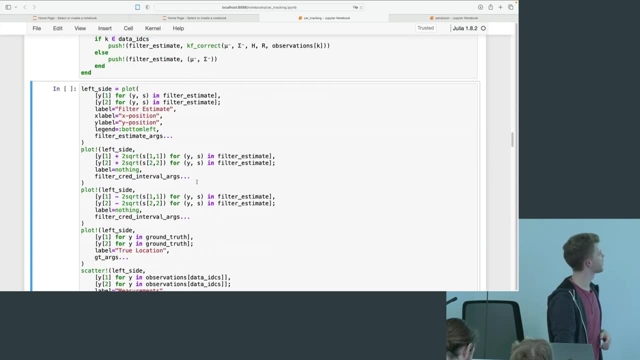 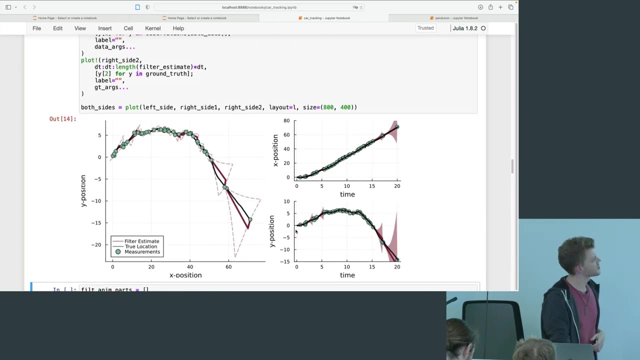 if you execute the Kalman filter- But this you don't have to do, It's not necessary- OK, We execute this loop- It's actually already finished because it's not a lot of data points- And then we plot it. So this is complicated code we don't have to look at, And we see that this is. 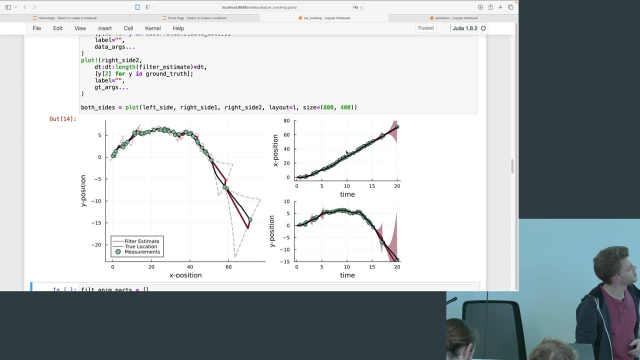 our resulting estimate. You see, here on the right the x position is regressed in a way, And here in between those measurements you see the uncertainty. So this is the marginal uncertainty, or two marginal uncertainties, marginal standard deviations. Now we got it In between those measurements and you see the 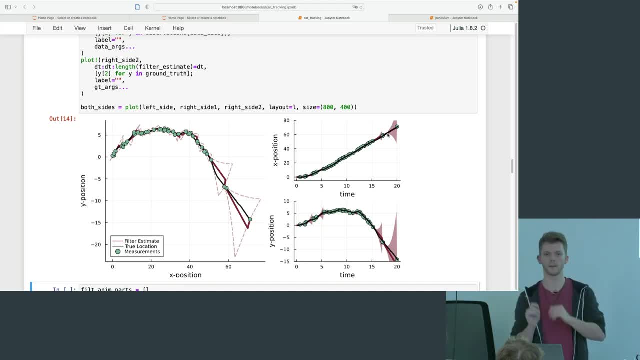 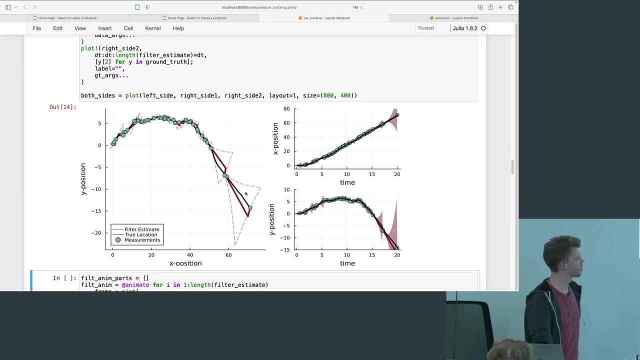 further away we get from the previous data point, the larger this and the larger and more rapidly this uncertainty grows. You see this also here. It's a little bit difficult to plot this uncertainty in two dimensional space, or in the state space, so to say, because we would actually, in order to make 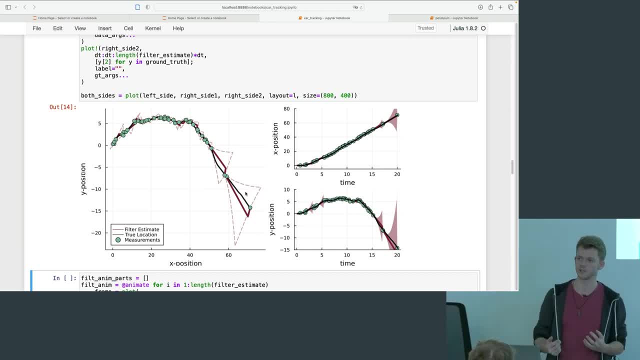 this correct plot: Gaussian contour lines around every step that we take, And then this plot would just be cluttered. So I didn't do that. This is the best we get, but it's kind of inaccurate. Yes, No, we don't do anything fancy like that, We just use the prior as given by our A metric. 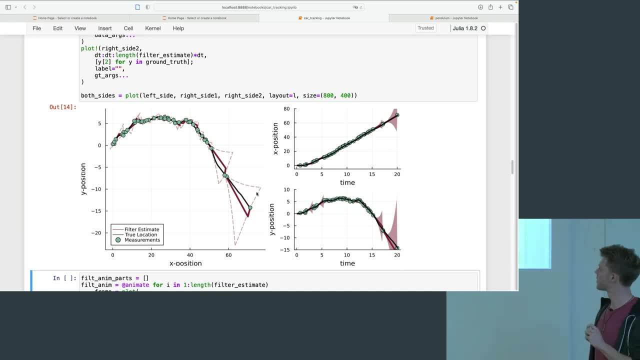 Oh sorry. the question was whether we somehow correct using the time step or by decreasing the time step in between those measurements, Right, If I understand your question correctly. I'm not entirely sure what you mean by it's different from the usual discretization, Maybe. 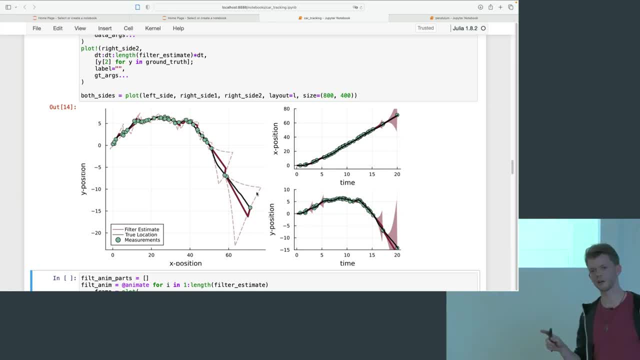 should we? maybe I can try and answer this question offline, Okay, Anyway, so you see here that also here the fact is reflected that our model just predicts in between measurements using its dynamic model. And because it's linear, it's just a linear line, right, And as 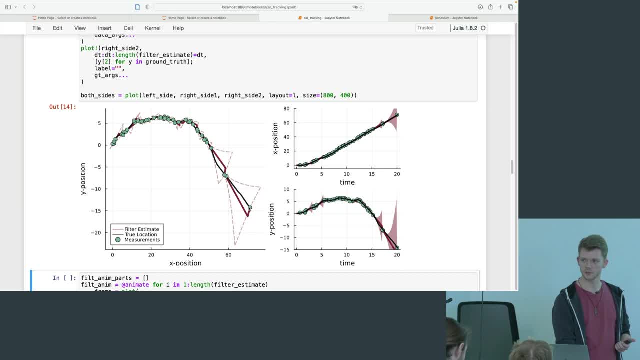 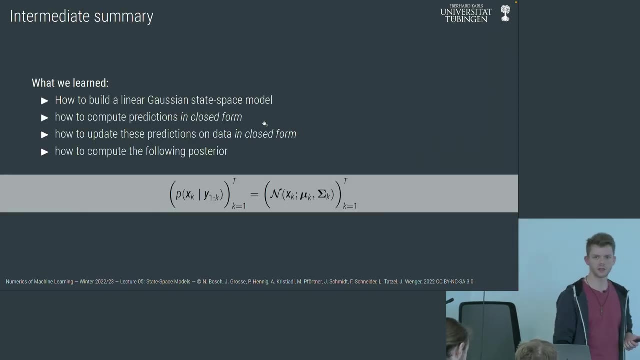 soon as new information trickles in, we snap back onto the trajectory because we trust our data, And the uncertainty also rapidly decreases, And this is our filtering estimate for this task. Okay, Now we go back to the slides And look at what we have learned so far. We learned how to build a state-space, model A. 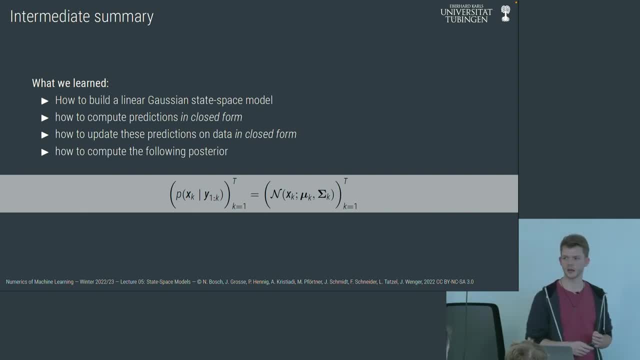 state-space model is the language that we are going to use to describe dynamical systems such as a moving car or a pendulum. We chose it to be linear Gaussian because then we can compute all the interesting quantities in linear- no, not in linear- time, using linear algebra with metrics vector. 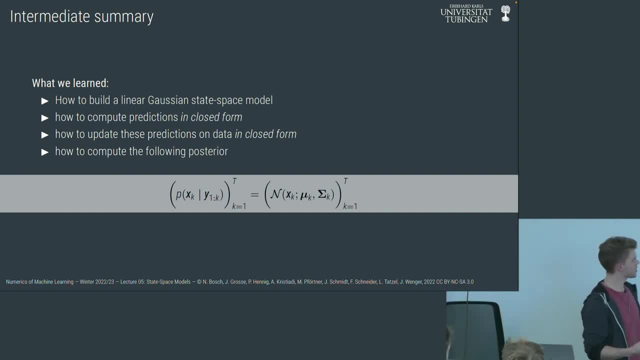 products and so on, And basically, the essence is: what we learned to compute is this posterior, So the sequence of filtering estimates that are only informed by the past and the present being a collection of Gaussian random variables, And this is really cool for this online estimation setting. 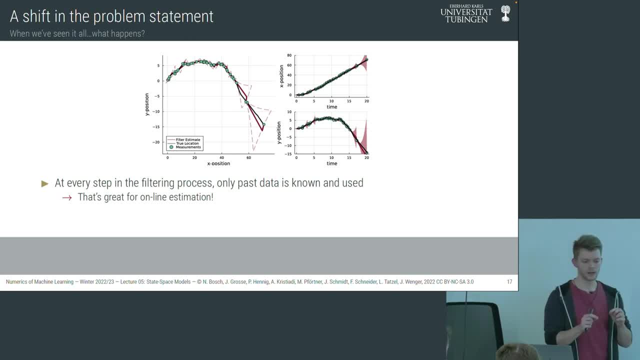 that I've been mentioning so often today, Because at our current, our most recent estimate, we have seen all the data that is available right Here, at this point the estimates are at the very end. Here it is informed about all the data points we have seen so far. 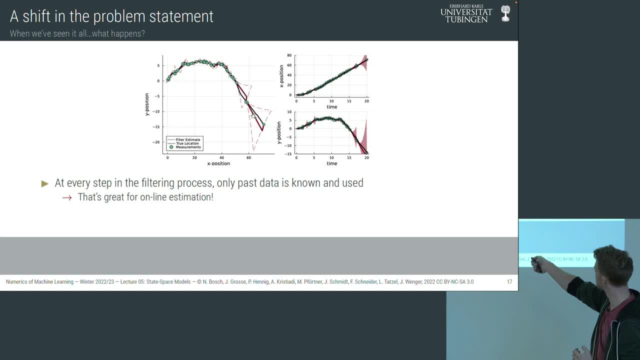 But this point here- I hope you see this- this point here- is not informed about this data point. This is just something this algorithm doesn't do. But if we now know our car at some point stops, it reaches its destination, and now we want to shift our problem statement. 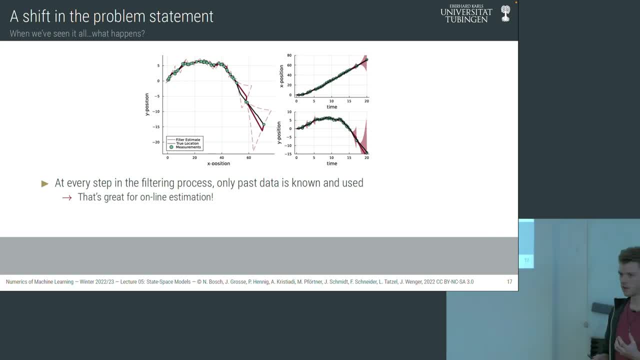 we shift away from. we want quick online estimation to the problem setting that we now want to know what the perfect estimate is, given all the data. So the correct estimate or the best possible estimate of this trajectory the card shows, given all the data, at every time point. 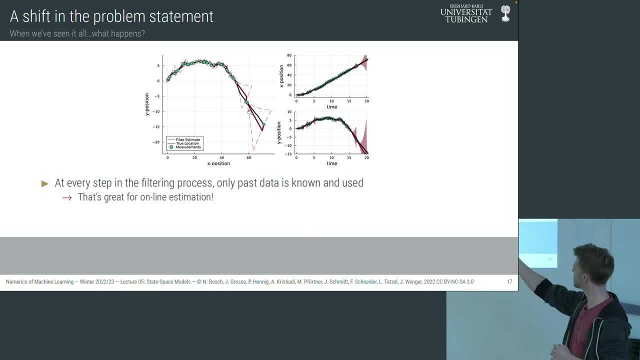 So basically, roughly speaking, we want, for example, to inform this estimate here about this data point here. Okay, Yes, and this shifts our problem statement- to compute a sequence of posteriors that have a different form. These are called smoothing posteriors. 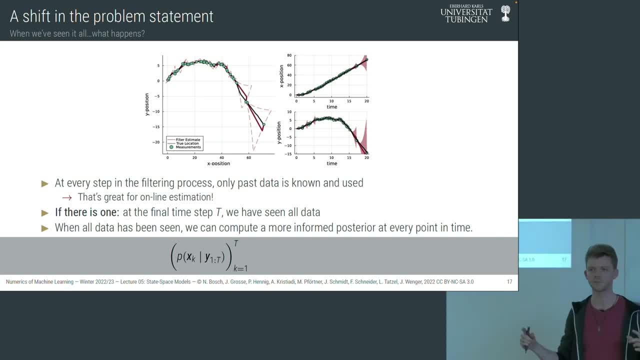 It's the measure, it's the distribution about our current state. given all the data points available, Why want to capitalize? Why do we wanna capitalize? Let's say that you calculate. Now, if I dot expert press, sorry, which is ct pocket did we just take? 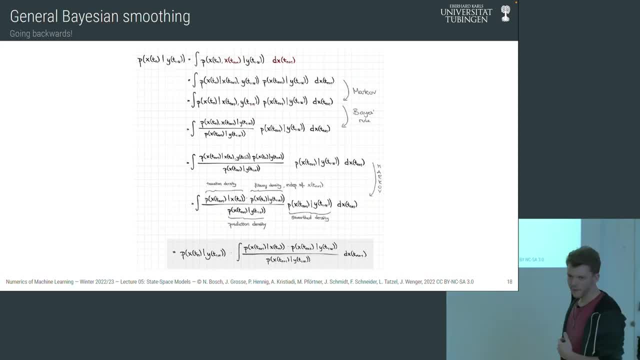 Yeah, ct is an instant log with cubit and instant, which is ab Boss, And I'm already going to tease it. This is going to be a collection of Gaussian random variables as well, So this is quite easy to compute, as we will see, and the derivation is actually quite difficult. 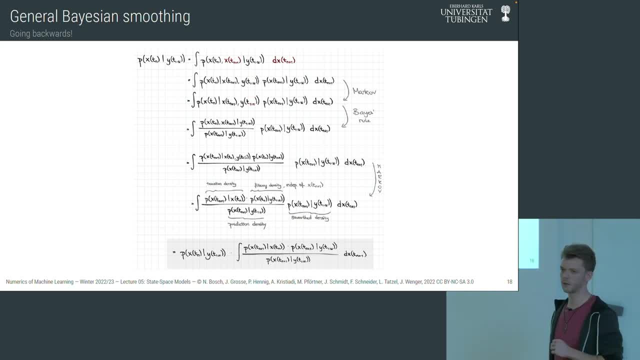 So this is just a handwritten note from when I was a master student on taking a course on time series analysis, And I don't want you show you what I used in order to make this derivation. I used the Markov property. I used 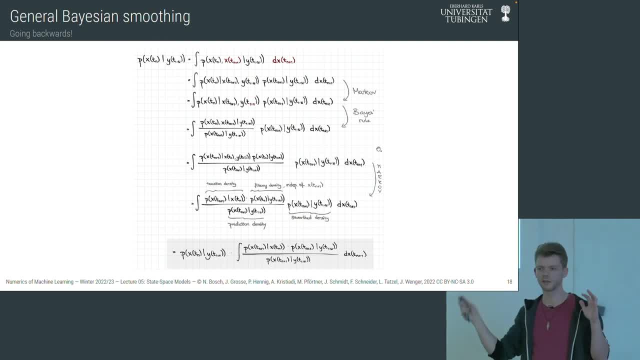 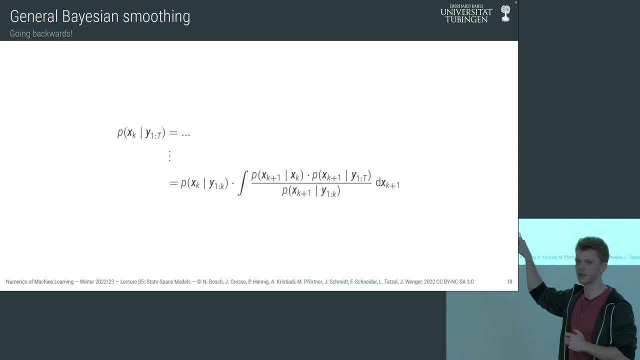 Bayes' rule and I used the Markov property again, and then some probability theory stuff in between. What I want you to look at is the thing that we compute, or that we want to compute, and the result in the end. So this is what we end up in. These are the general smoothing. 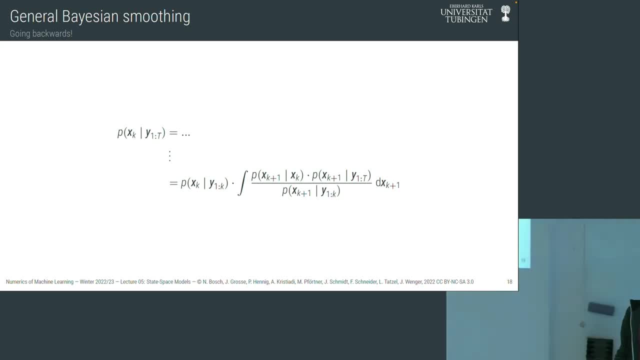 equations, so to say, And even though this might seem complicated, all of these conditional distributions, all these terms over there, you know already. You see here the filtering distribution and it already tells us something. We have to compute the filtering distribution. 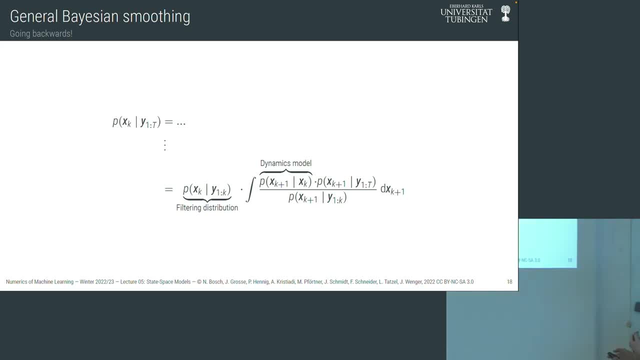 in order to compute the smoothing distribution. Okay, here we just have our dynamics model p of the next state. given our current state, This term is especially interesting. This is the smoothing distribution at the next time step. This is the quantity we want to compute. 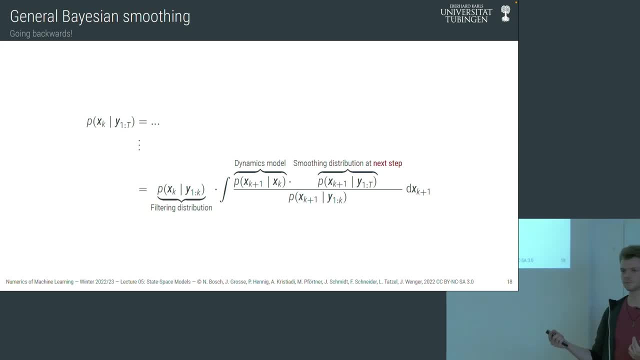 just at the next time step. So what does this tell us? Yeah, I saw a good gesture over there. What do you mean Exactly? We have to go backwards. This is going to be a backward recursive algorithm Based on our filtering distribution, the dynamics model and the thing down here. 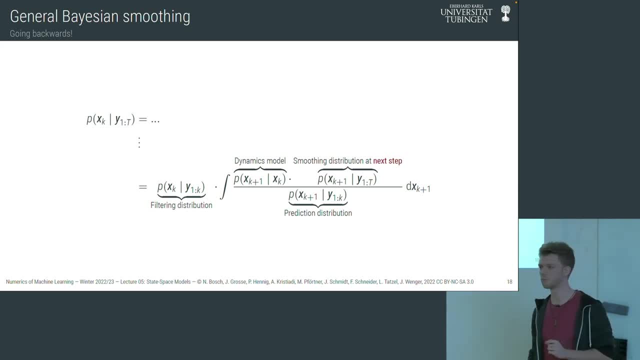 this is just our prediction distribution. Notice that there is no measurement model involved here. It's just using the filtering and prediction and the dynamics model and our smoothing estimate at the next time step, And then we just marginalize over the next time step because we don't care for it. 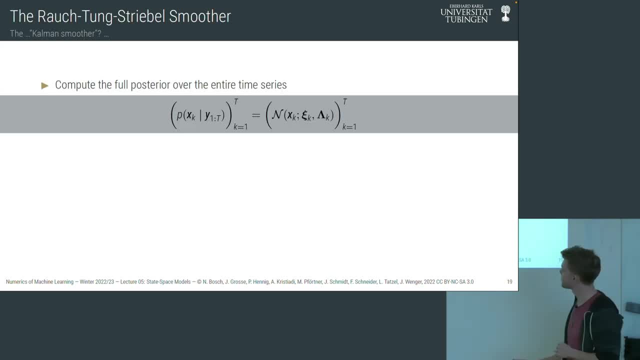 If we now go back to the setting of linear Gaussian state space models, I already told you it's going to be a collection of Gaussian random variables. We can write down matrix vector product operations to compute first the smoothing mean. It's a matrix G. No smoothing mean Smoothing gain, Smoother gain. this thing is called. 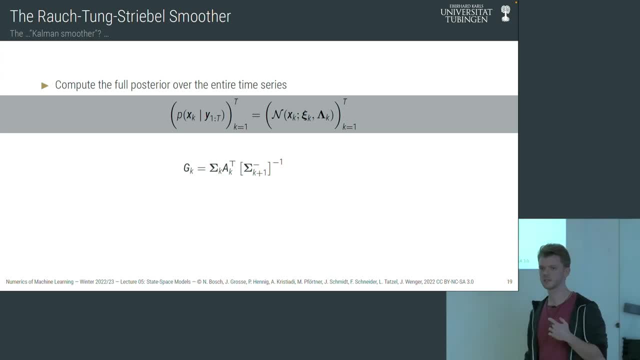 It is a product between the filtering covariance matrix times, the, the transition matrix transposed times, the inverse of our predicted covariance at the next time step, And this matrix is all we need in order to compute our updated mean, in which we just add to the filtering mean the product of the smoother gain times, a residual term. 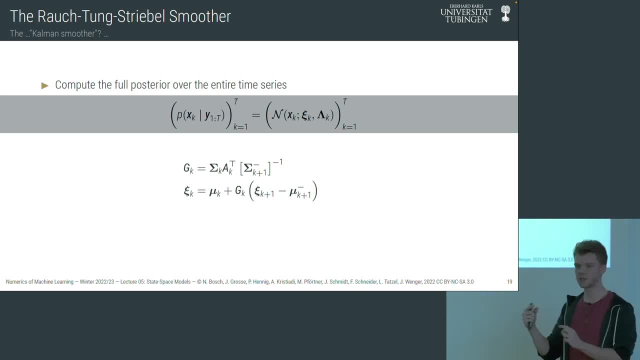 between the smoothing mean at the next time step and the predicted mean at the next time step. And the smooth covariance matrix is comes about by adding to the filtering covariance- Uh, the product of. so we first built this residual term between the next smoothing covariance and the predicted covariance. 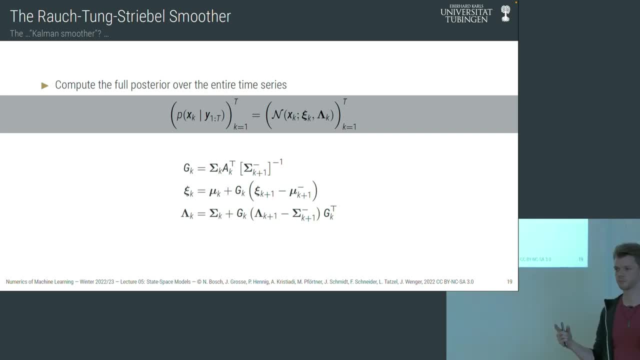 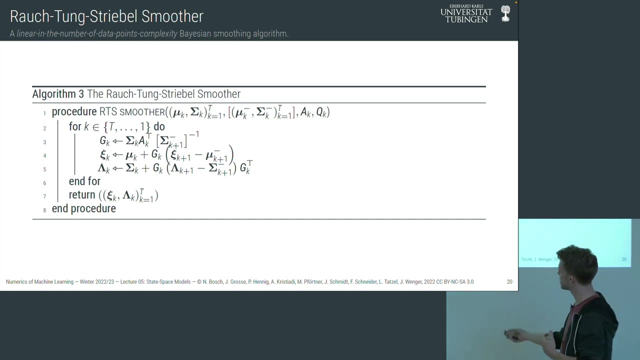 And then we just multiply the smoothing gain from the left and the right. Just three equations makes it possible to compute this posterior from our filtering posterior, And then we can write this into an algorithm as well. Notice now that we shifted from formulating Y loops to four loops, because this algorithm only makes sense if we have any. 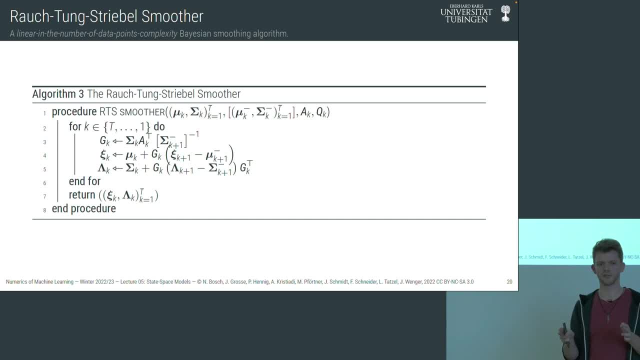 a data set or at least a fixed portion of time steps that we want to consider, because from the very end we go backwards now up until the beginning. It is highly unlikely that there are new measurements coming up in the beginning of the time series. It's just not how time works. 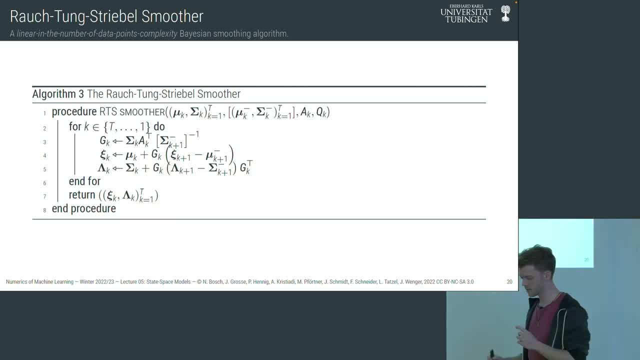 Anyway, we start from the end of our time series because, as I already told you at the end of the time series, our filtering estimate coincides with the smoothing estimate. and then we go backwards in time- See here for for K In T, up until the one. we compute the smoothing gain and we use the smoothing gain to compute the smoothed moments. 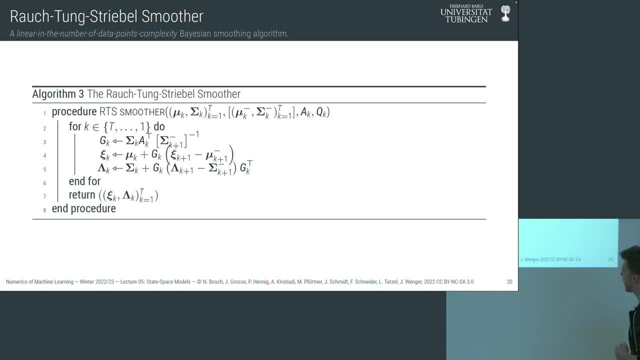 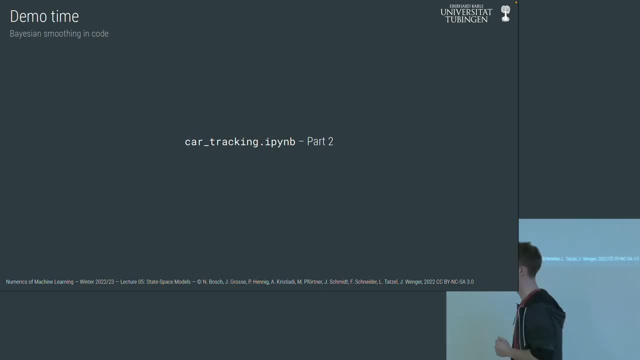 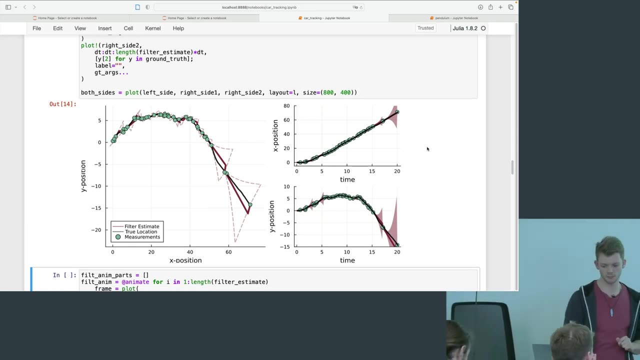 And then in the end we return the sequence of Gaussian random variables and this is our smoothing estimate. Okay, let's look at this in code again. Well, nice, Okay, we're still in the same example. It's just part two. basically, We scroll down for a bit. 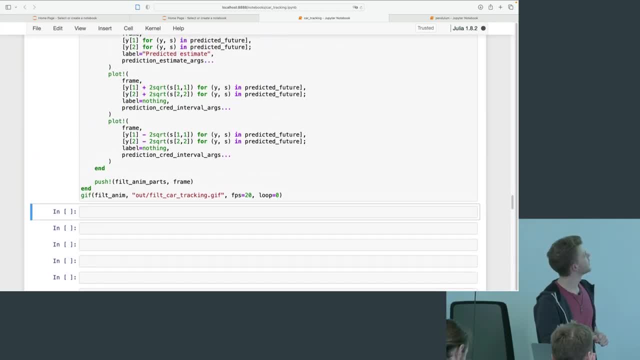 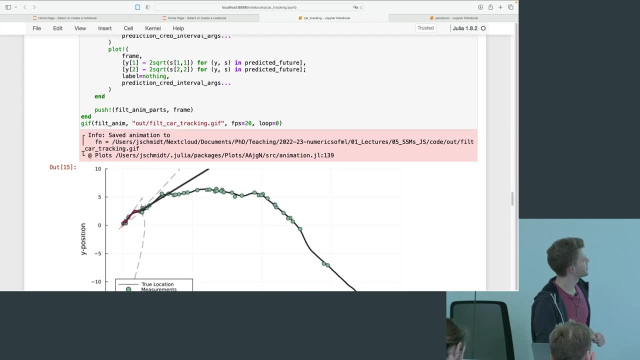 Oh, actually I forgot to show you the animation. Wow, Let's look at this really quickly. It's an animation of the filtering estimate. Real quick, because I like animations. Whoop, you see how this comes about. You see, here again, for visual reasons, plotted, a prediction. 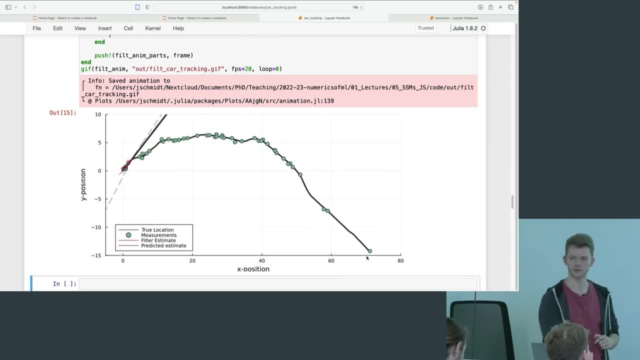 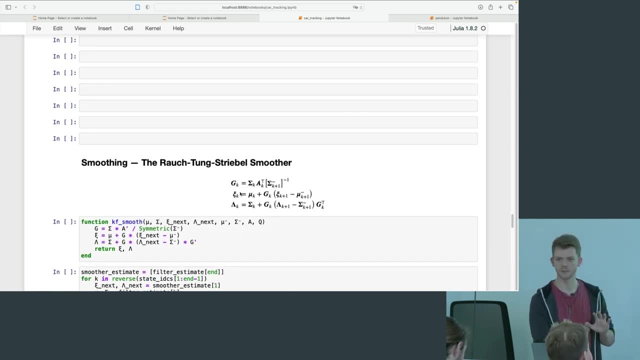 every time, and then you see how the uncertainty snaps back every time we see a data point. Now for smoothing, we again translate the equations we just saw. You don't have to memorize them. Of course, I put them on the slide such that you can look it up later, but we just translate them into code Again. 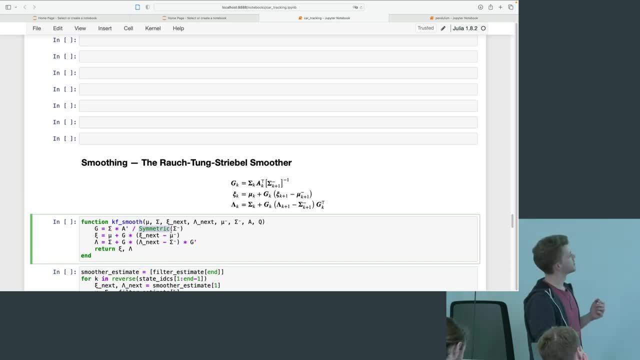 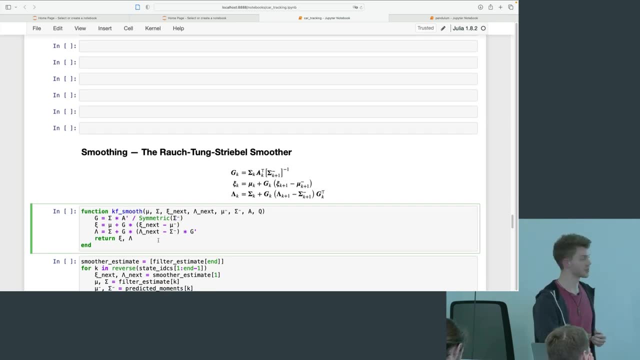 we are going to tell the algorithm or we tell the compiler that this matrix here is symmetric. It's a covariance matrix. So we divide by that. by solving a linear system, We use the smoothing gain to compute our smooth moments. We return them. 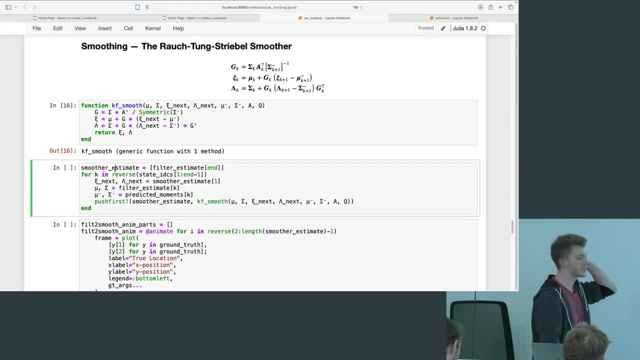 Execute. and then we're going to initialize our smoother estimate, our trajectory, with the final filtering estimate from before, And then we go k steps in reverse over our state indices Select from the beginning of our list because we're going backwards our current smoothing estimate. 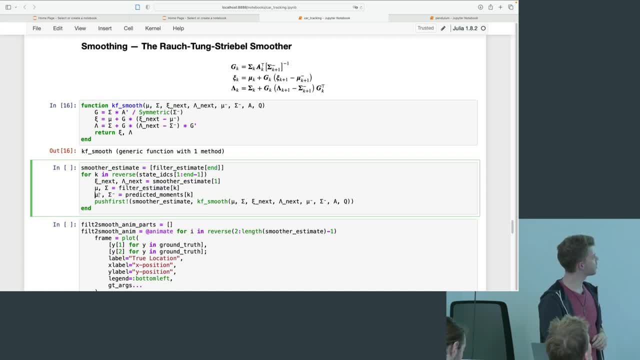 We select our filter estimate at time step k and our predicted moments at the time step k, which I sneakily saved earlier. I didn't tell you about that, but I saved them because we don't have to compute them again. right, These are pre-computed during filtering anyway. and all of that we are going to provide this smoothing function with, together with our dynamics model. 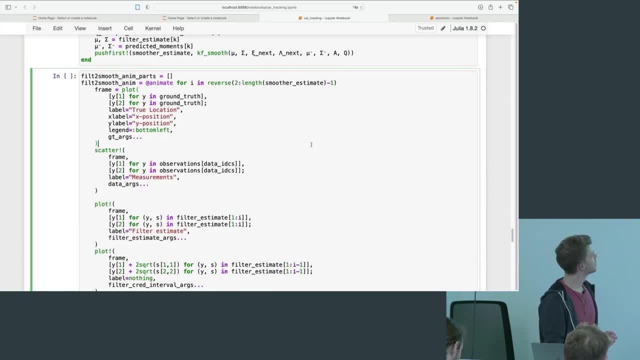 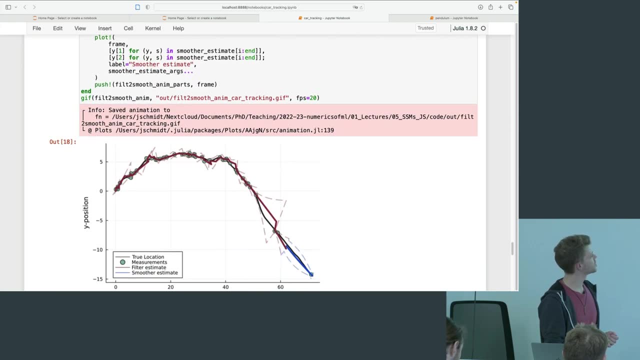 We're going to execute this loop. It's already finished. And look at the fancy animation in which our smoother now smoothes out our filtering distribution. I've started off here with this plot in the xy-plane because it's just nicer to look at. but 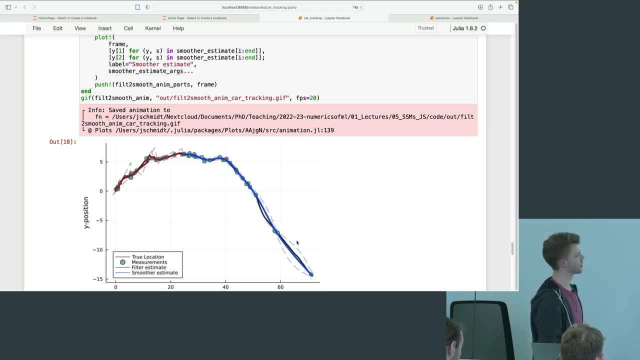 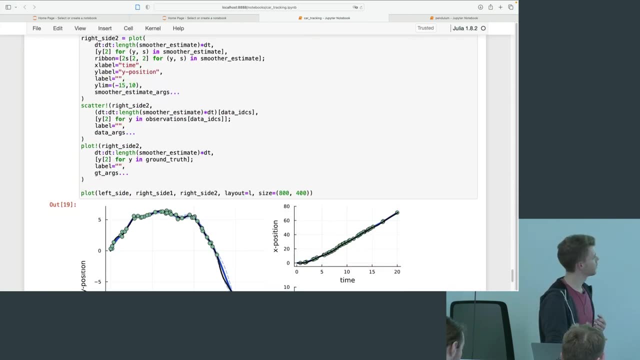 this uncertainty here is, as I said, a bit difficult to interpret. So if we want to see the actual clean truth, we have to look at this plot which plots the same thing. So if we want to see the actual clean truth, we have to look at this plot which plots the same thing. 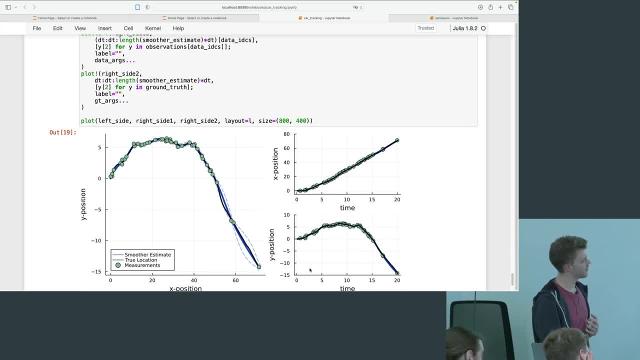 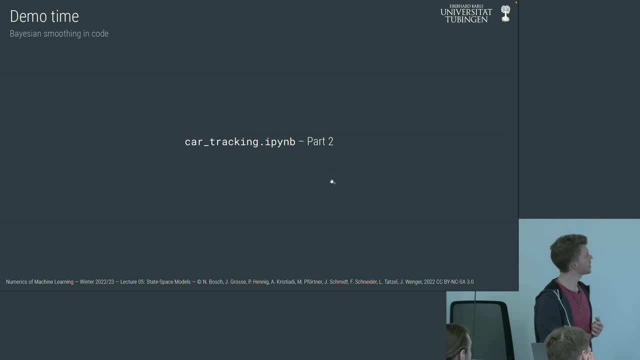 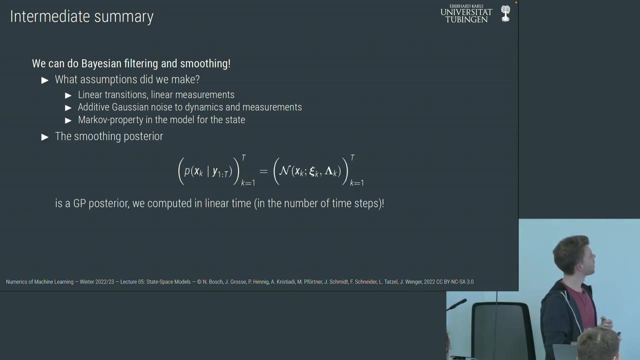 Just as a time series here, and you can see that now we have a nice interpolant between those points. Actually, this nice interpolant is a Gaussian process posterior we just computed. So the smoothing posterior, this collection of smoothed random variables. 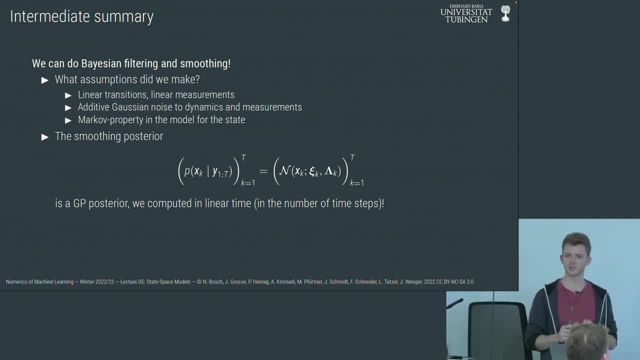 are the marginals of a Gaussian process posterior. we just computed in linear time, going one time forward and one time backward. Again, I cannot tell you why exactly this is. I'm just going to tell you If you are very interested. we can talk about this a bit in the tutorial. but this again has to do with 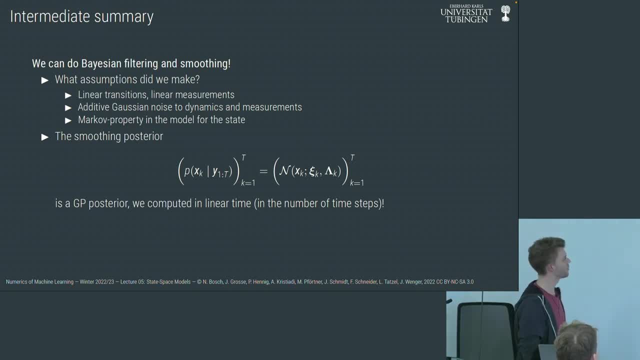 stochastic differential equations and very complicated math, Anyway. so what assumptions did we make for that? We assumed linear transition, linear measurements, we assumed additive Gaussian noise to both these dynamics and measurements and we assumed the Markov property. Okay, now we can compute Gaussian process posterior. 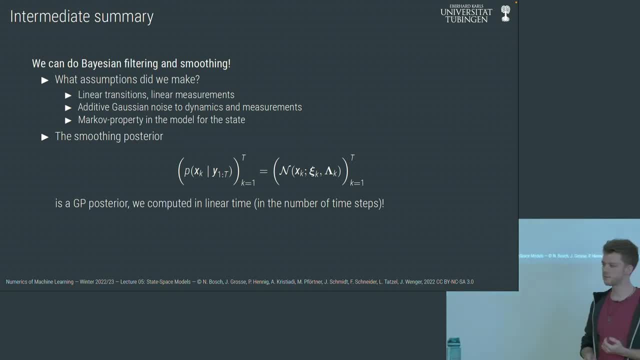 which is a Gaussian process posterior in linear time. Does that mean that you can forget everything that Jonathan Wenger told you over the past couple of weeks? No, I only told you that every smoothing posterior is a Gaussian process posterior, but not every Gaussian process posterior that you can compute can be computed using Gaussian filtering and smoothing. 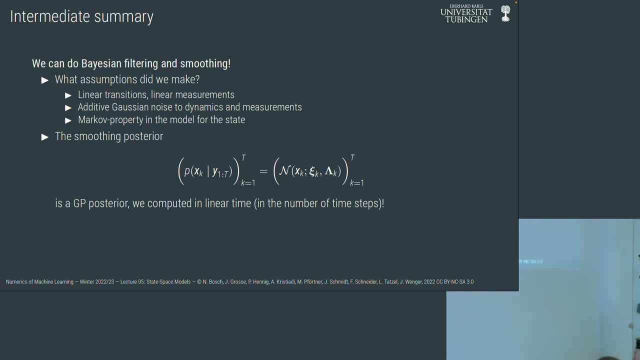 This is just something that you can keep in mind. Okay, now we can do Bayesian filtering and smoothing- Cool. Are there questions? I know it's a lot of stuff that you're going to learn at the moment or that you are learning at the moment. 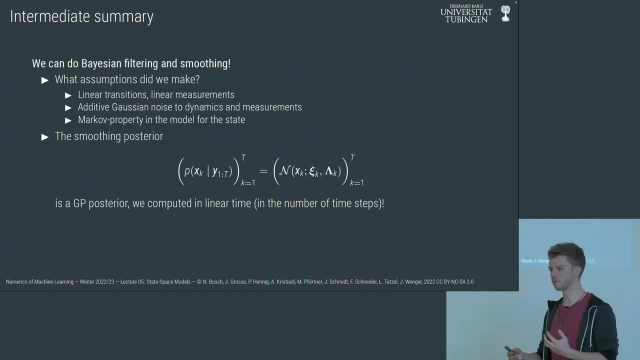 You don't have to memorize every equation, I just want you to have them, such that you can look them up. Far more important are the principles I keep repeating over and over again Before now taking the next step. What could this next step possibly be? Remember that our ultimate goal 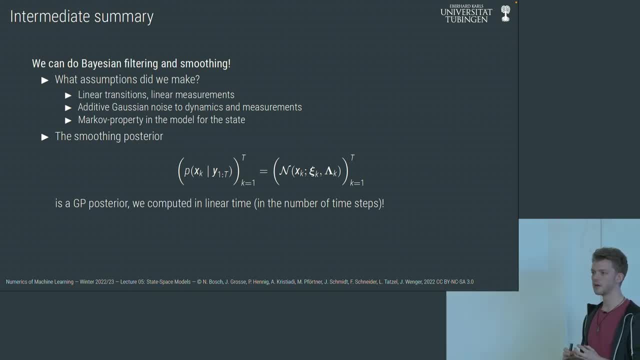 why we actually are chewing through this theoretical part now is simulation of complicated dynamics. So what kinds of models do we have to look at? next, One keyword. One keyword that makes everything so much more difficult. No, we're going to stick to the Markov property, because otherwise it would screw up our framework entirely. 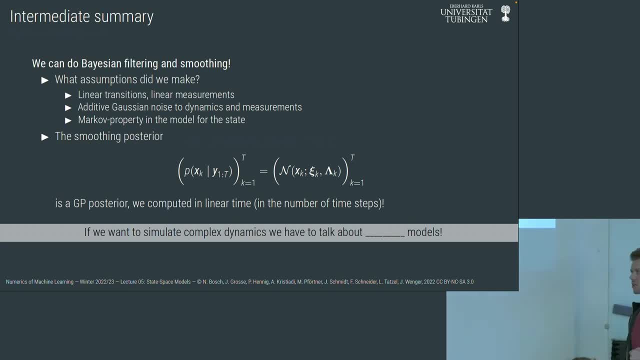 Yes, Non-Gaussian is also something we're going to. Why did I ask this question? No, we are going to stick to Gaussians. I'm going to tell you that it is possible to drop the Gaussian assumption in the very end. 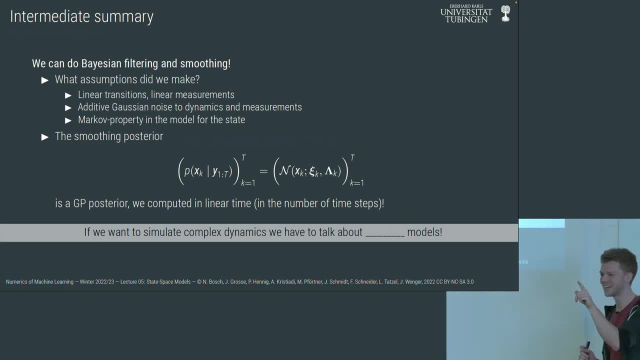 But I'm not going to show you how. Yes, Yes, Thank you. We're going to talk about non-linear models, But these are very good comments that bring up. Especially the non-Gaussian thing brings up an entirely new class of algorithms. 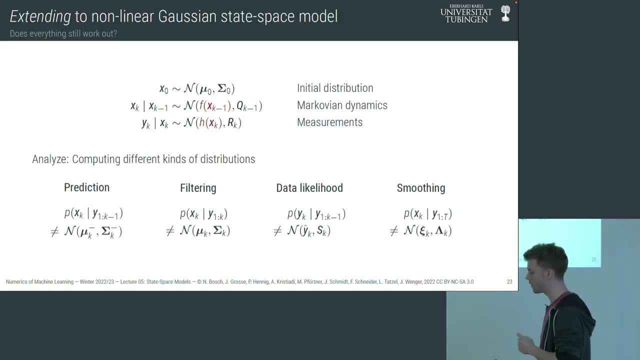 Anyway, we're going to talk about non-linear models. If we return now to our state-space model, you see here that this F-line transformation of the previous state has been substituted, has been replaced by a general function F for the dynamics model. 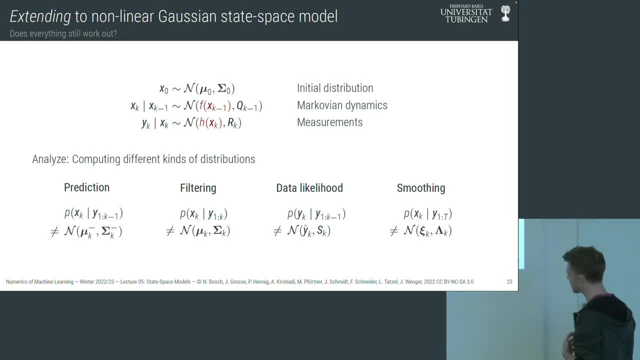 and a general function H for the measurement model And, as all of you probably know, non-linear functions of Gaussian random variables are not Gaussian random variables anymore, So everything doesn't quite work out yet. So this doesn't mean that we have to stop here. 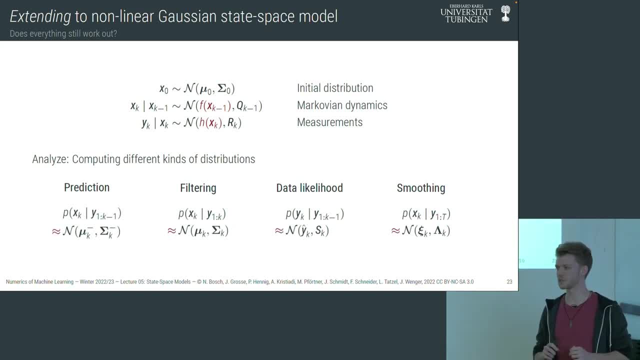 We just pretend that we are dealing with Gaussians. We're just going to approximate our model and use Gaussian inference again. How are we going to do this? The principle is actually quite easy. We are going to use both of these functions, F and H. 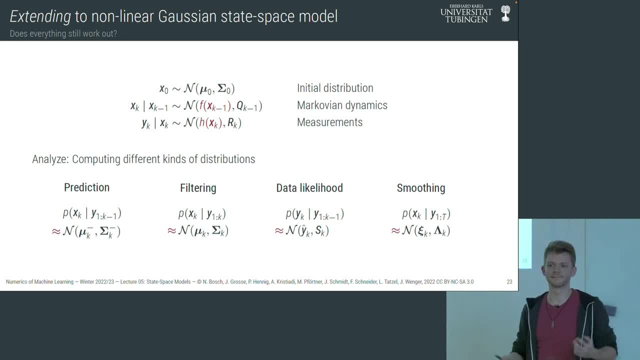 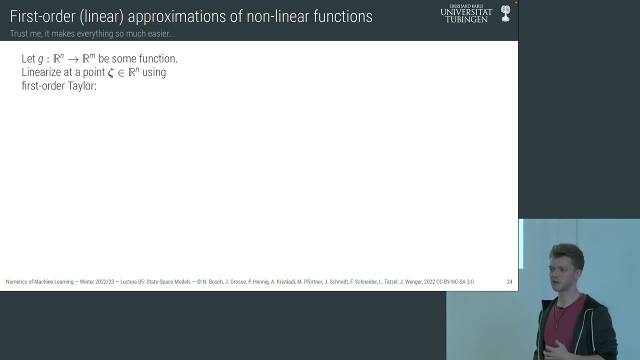 and we're going to linearize them and then use Kalman filtering again. It's as easy as that. How are we going to linearize them? As you probably know, we're going to use a Taylor approximation in first order, because we linearize. 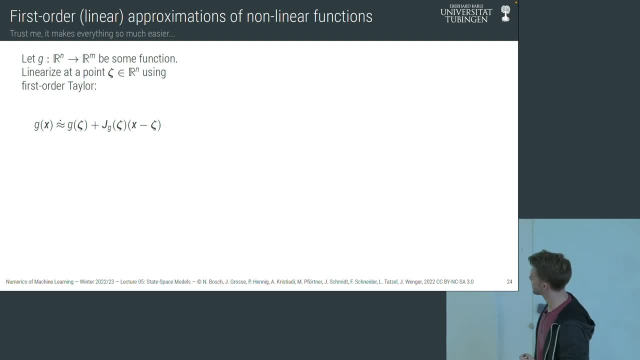 I just quickly wrote this down here again. So for a general function G you can form a first-order Taylor approximation which is an approximation as a linear function in a linearization point, theta, Theta, And it involves the Jacobian matrix which I denoted here. J, sub G. 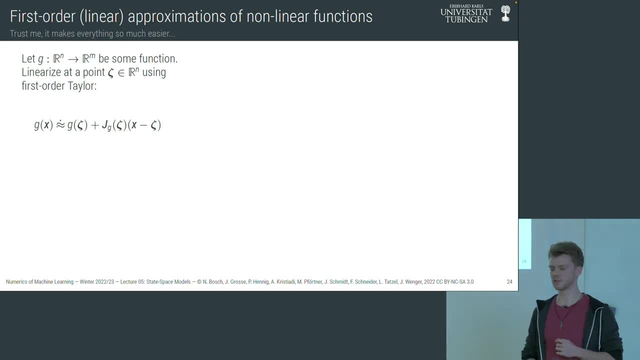 of the non-linear function G evaluated at this linearization point theta. We can rewrite this Taylor approximation and reorder the terms such that we see that we have a linear or affine function, again, AX plus B, where A and B arise from this Taylor approximation. 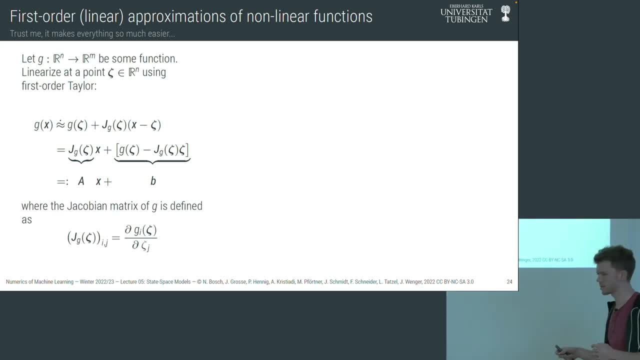 Just for you to remember, the Jacobian matrix is just the matrix containing all the combinations of partial derivatives of this vector-valued function G. All of you probably know this. Okay, let's look at a few pictures quickly. So here we have this non-linear function G in blue. 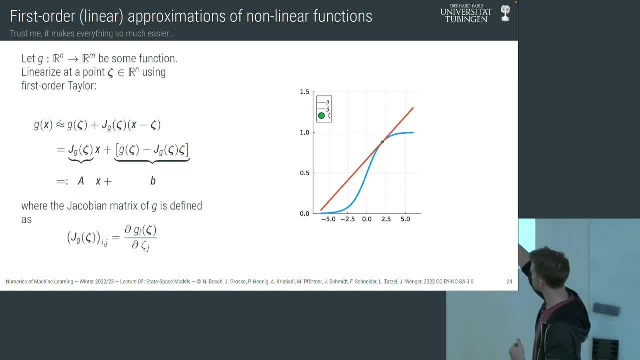 It's just a logistic sigmoid function. We chose one linearization point, theta, this green dot, And in this dot we approximate the non-linear function G with the linear function G hat. This is this orange line And you see, the further we get away from this linearization point. 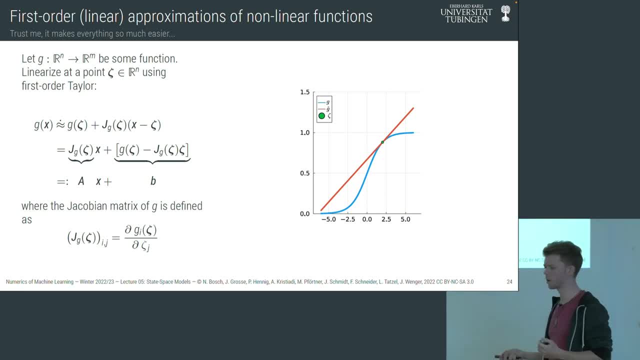 the worse the approximation gets Okay. but we don't want to talk about analysis here, We want to talk about random variables. So let's draw a few samples from a random variable, And this is Gaussian distributed with mean 2 and standard deviation 1.. 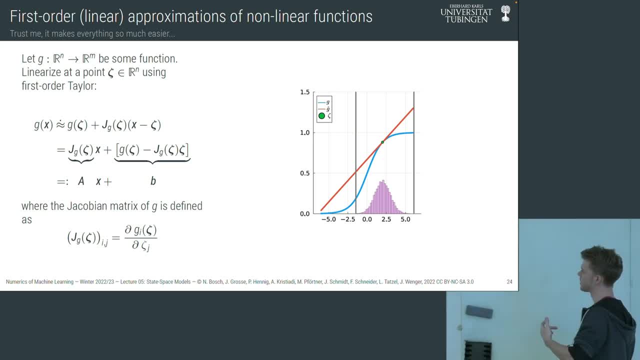 And now we see what happens if we map these samples and compute the push-forward measure, so to say by mapping all of these samples through this non-linear function, And we end up with this distribution, which is clearly not Gaussian. It doesn't look Gaussian. 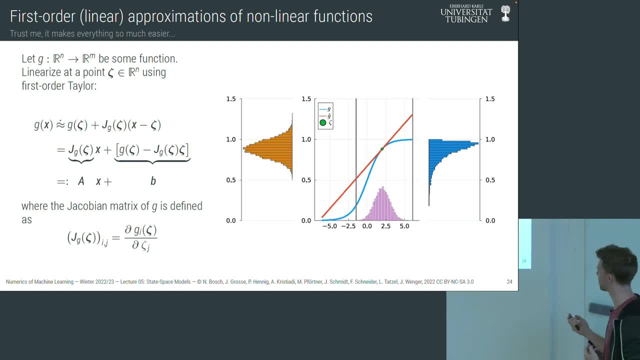 However, if we map it instead through this linear function, we get this distribution, which is again a Gaussian distribution, as you would have expected, And we can see it's just an approximation of the true distribution. It's really quite different. This one is not symmetric and the means doesn't really match up. 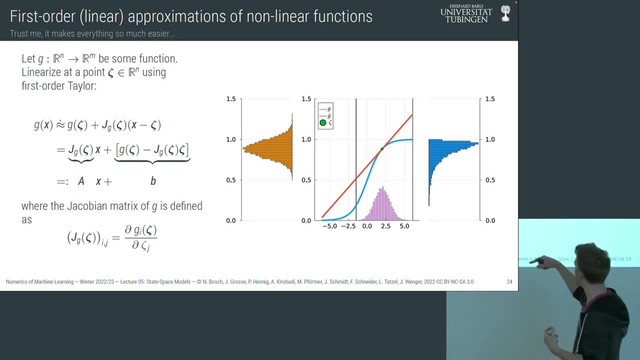 And this here the map samples to outside of the image space of this non-linear function, everything. But we're just going to use this approximation for now because we want to use Kalman filtering, because it's so nice. Okay, So how we proceed now is we just: 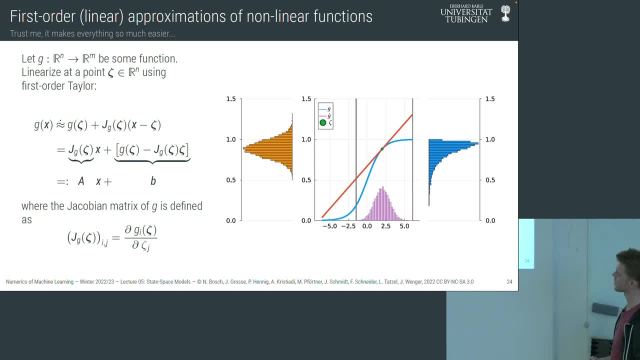 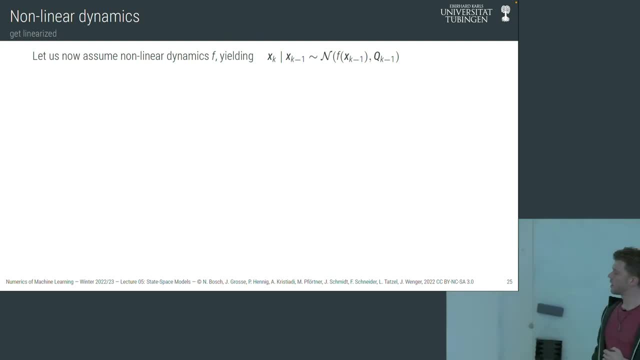 we just linearize everything that is non-linear in our state-space model and we will begin with our non-linear dynamics. So we are given this model xk, given xk minus 1, is this non-linear function of xk minus 1? 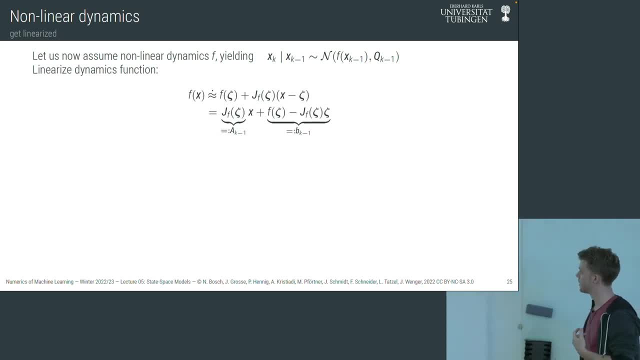 under additive Gaussian noise. We are going to linearize those dynamics and we are going to have these terms involving the Jacobian as our new matrix A and this affine term involving the evaluation of our non-linear function and something else involving the Jacobian. 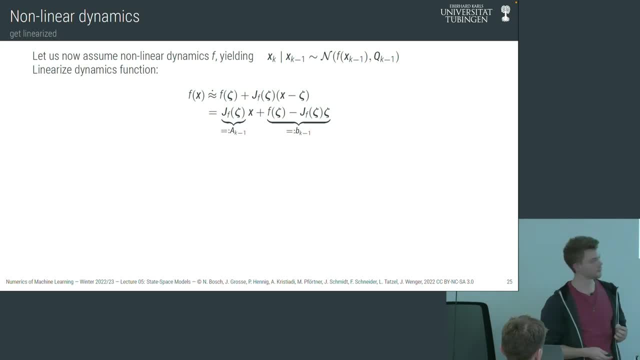 as our affine term. This just drops out of the Taylor approximation. Okay, As soon as we did this, we ended up with a affine model again. So we have a linear Gaussian dynamics model here, where the terms just arose from the Taylor approximation. 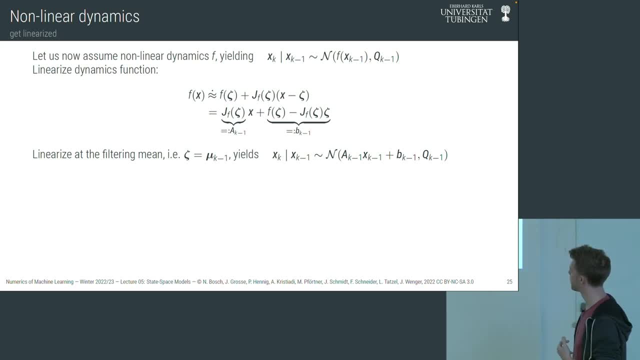 And what we do now is we just insert those new system components into our Kalman filter equations. So for the predicted mean- and this is really nothing else than the Kalman predicted mean which we saw before we insert instead the Jacobian and this affine term, 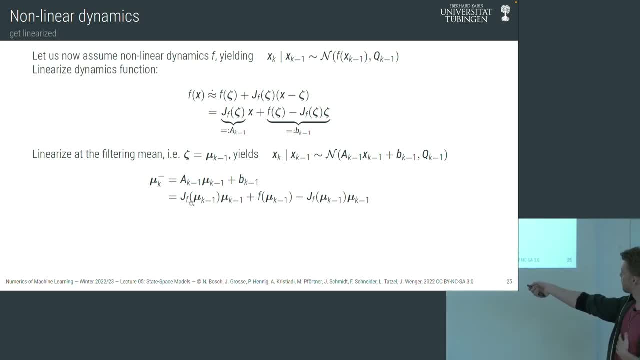 And we see already here that we have here plus this Jacobian term and minus this Jacobian term, So these two cancel out And the predicted mean is just the non-linear dynamics function evaluated at the previous filtering mean. I forgot to say that we choose. 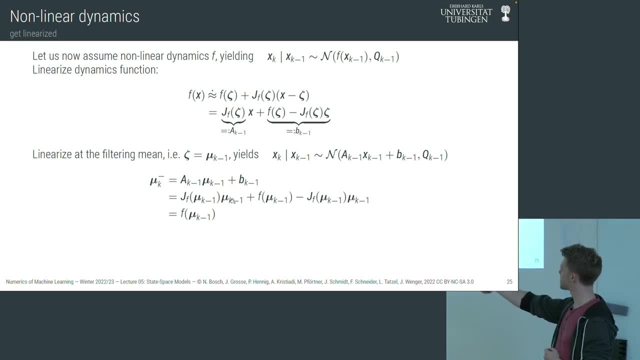 this comes about because we choose the linearization point smartly. We choose theta to be the previous filtering mean. So this way all of this cancels out nicely For the predicted covariance matrix we also just insert. for every transition matrix we find the Jacobian matrix of the non-linear function f. 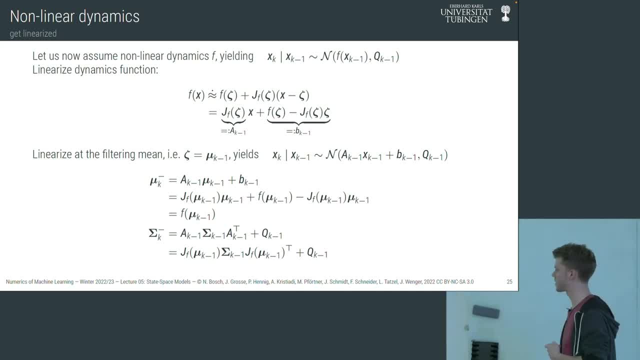 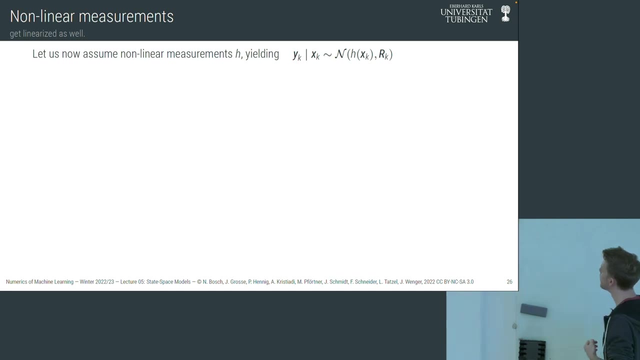 And then we have this term Jacobian times, filtering covariance times, Jacobian transpose, plus our process noise covariance matrix Q. Okay, So we now have equations that allow us to deal with non-linear dynamics, And we do the same for the measurements. We have this non-linear measurement model, yk, given xk. 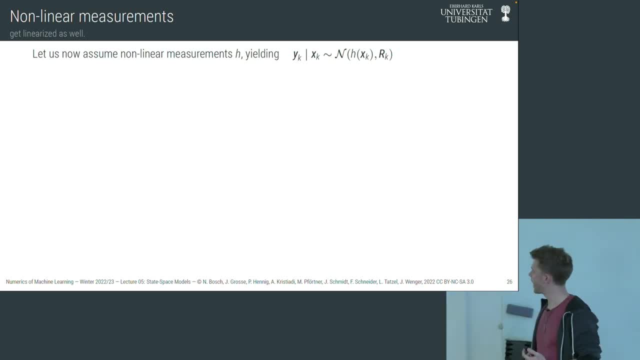 is this Gaussian random variable that involves this non-linear function, h, evaluated at xk. We linearize this function. We get this form: hx plus c, where h and c comes about from the Taylor approximation. as before, We choose as the linearization point: theta equals the predicted mean. now, 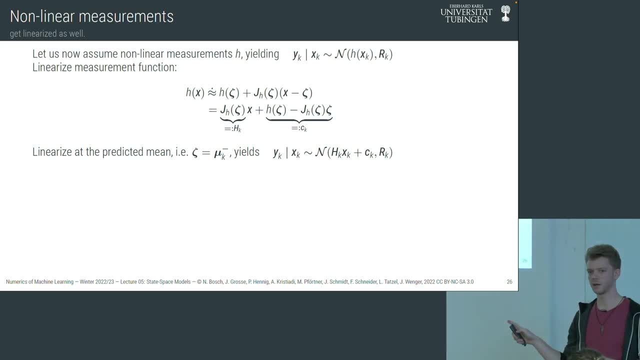 We recognize that we have a linear Gaussian model again and we insert everything into the Kalman filter equations. We just compute our Gramian matrix S just using the Jacobian. now, instead of the transition matrix, The Jacobian is our new transition matrix, if you will. 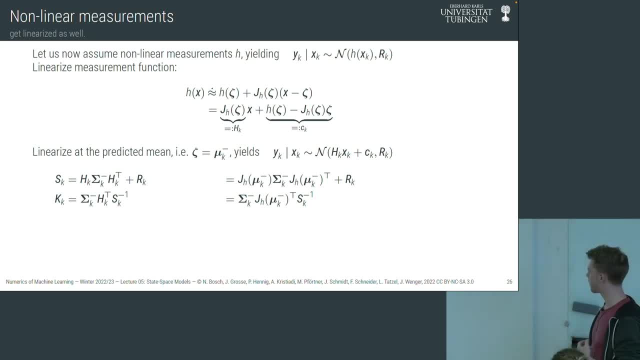 At our measurement covariance matrix R, we compute the Kalman gain in the same way For the updated mean we recognize. again if we insert our Taylor terms into this equation. here we end up with this term after rearranging the terms for a bit. 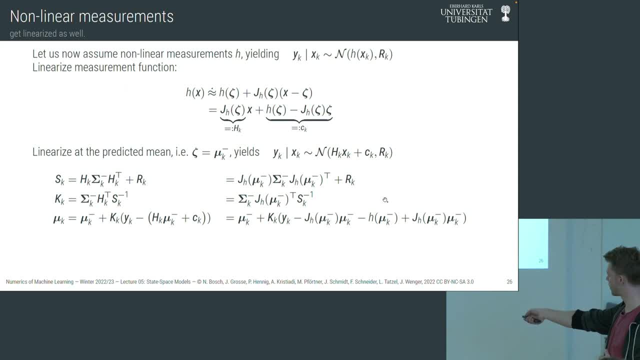 and we have minus Jacobian, plus Jacobian again. So our measured predicted mean is just the evaluation of the non-linear measurement function at the predicted mean. So the residual term is this: yk minus h of predicted mean. Okay, And for the updated covariance matrix, 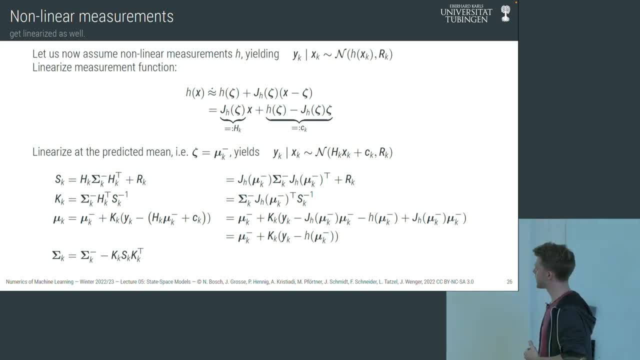 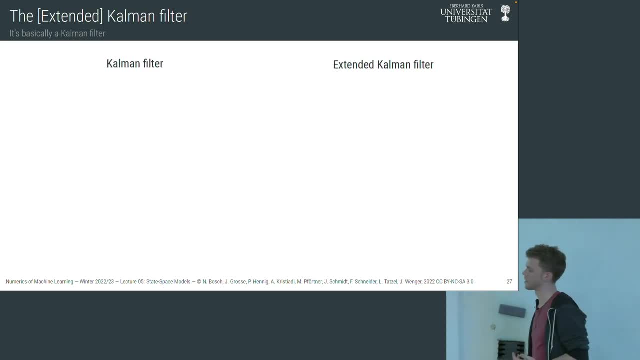 actually nothing changes. What we end up with are equations for the so-called extended Kalman filter, And it's nothing else than this. It's just an extension of the Kalman filter for non-linear dynamics and measurements, And they are actually so similar. 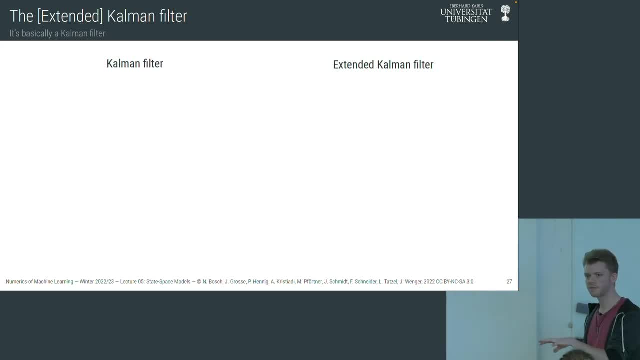 that I chose to introduce a slide again where I just write down the Kalman filter equations next to the extended Kalman filter equations and highlighted in red everything that changed. We just predict our mean with this non-linear function. substitute every transition matrix with the Jacobian. 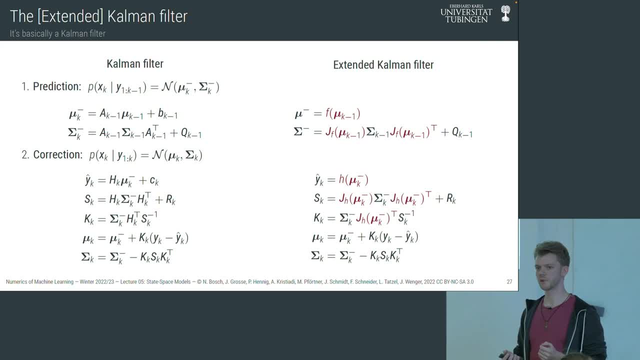 and think of our Kalman filter equations. That's basically all that matters, Just for these two parts. we see that we just have to evaluate our non-linear functions. Questions regarding the extended Kalman filter. Okay, Yeah, It still makes sense. 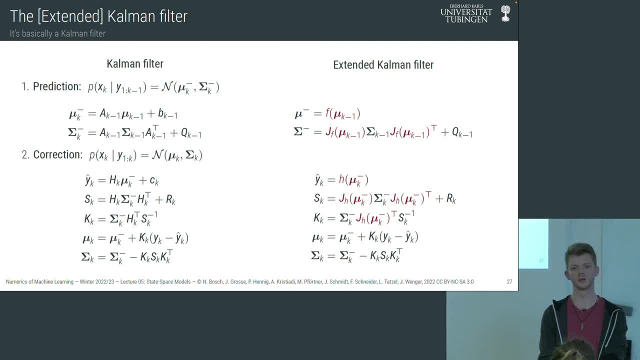 to do something similar with a function that you can't differentiate or don't want to differentiate for a reason, And use linear approximations there too. So linear approximations like calculating the function at different points. Hmm, Oh, okay, Interesting question. 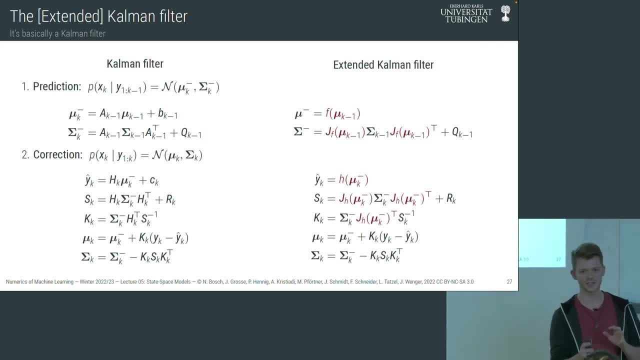 So the question is, what happens? or I slightly rephrased the question: what happens if we cannot differentiate our function? So what happens if we cannot compute a Jacobian? And you already gave a suggestion what you could do, like a finite differencing scheme, right? 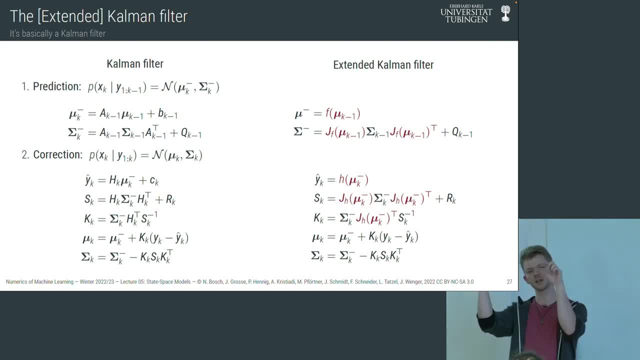 You've taken function evaluation at this point and the function evaluation at that point, build a difference like standard for finite differences and then do the same thing. I don't know if this works actually. Might well be that it actually works. 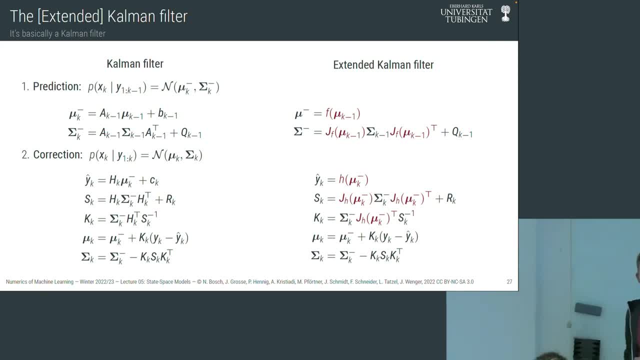 You can. you are free to try this instead of using a Jacobian. I think it works. Just maybe it gets unstable at some point. But yeah, feel free to try it out. We can talk about it in the tutorial, maybe. 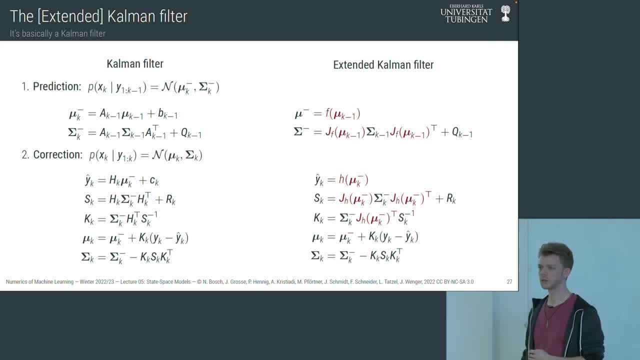 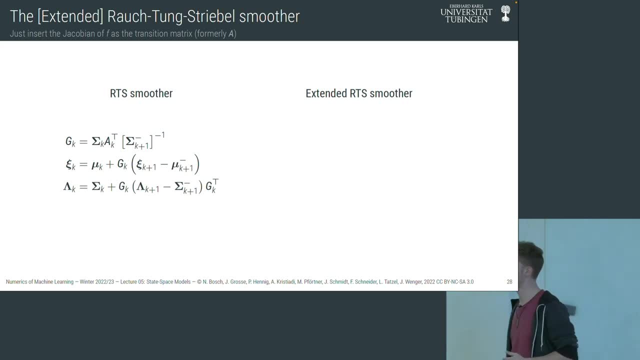 Okay, Cool, You can do the exact same thing for the Rauch Tum Striebel smoother or Kalman smoother, which is sometimes called, but it's not the correct name, So we just built the extended Rauch Tum Striebel smoother. 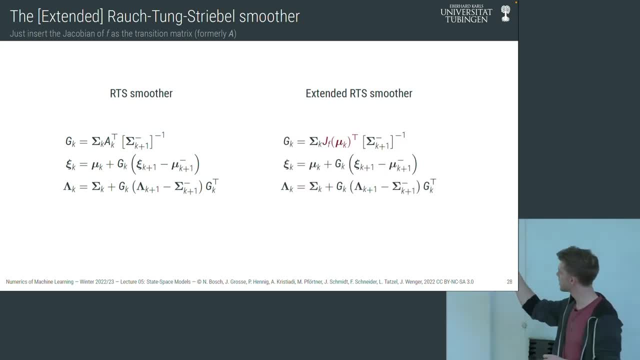 again by looking at the Rauch, Tum, Striebel smoother equations and insert as the transposed transition matrix again our Jacobian matrix of the nonlinear function f, evaluated at the filtering mean, mu, k. That's it, That's nonlinear smoothing. 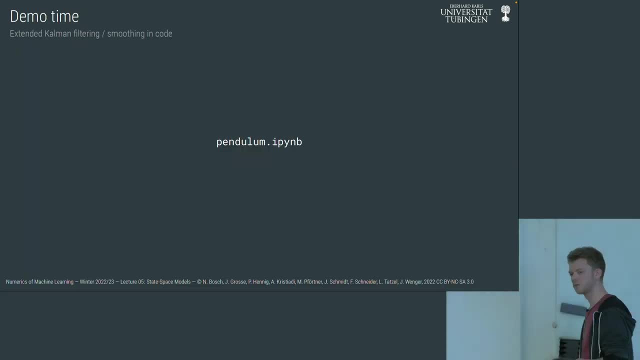 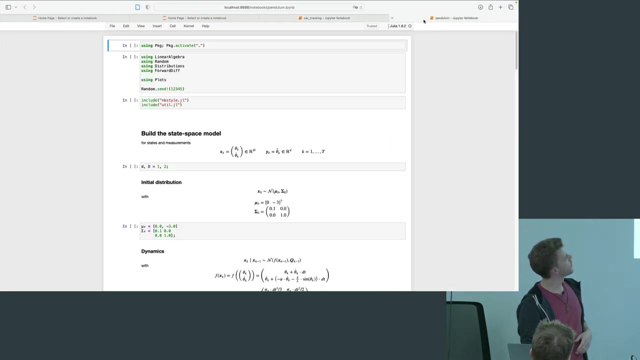 or one way to do nonlinear smoothing. Let's look at this also in a code example And, as the name already suggests, we are going to look at this dynamical system I've been talking about earlier, this pendulum Whoop Going to open the next notebook. 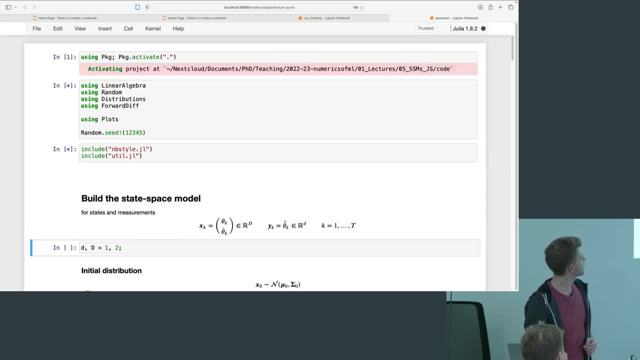 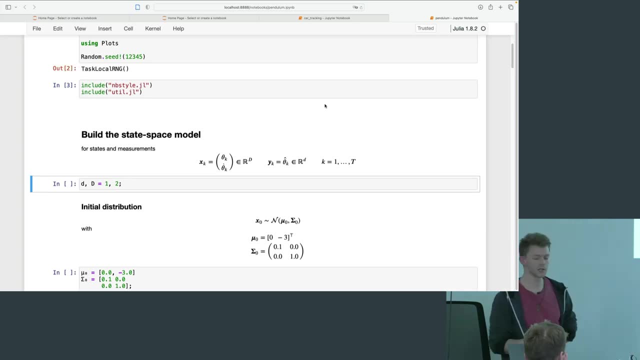 import some stuff and build our state space model. Our state space now consists of two components: theta and theta dot. Theta is just the angle of the pendulum and theta dot is the angular velocity, So our state dimension is two. 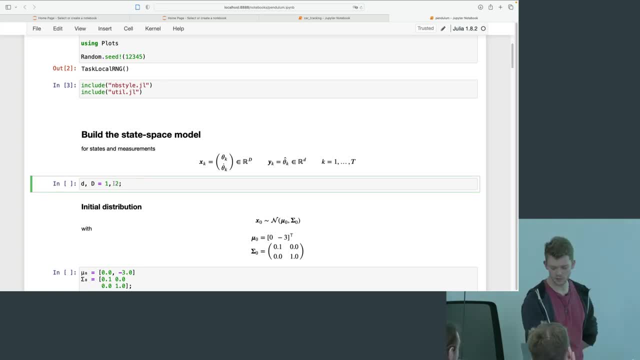 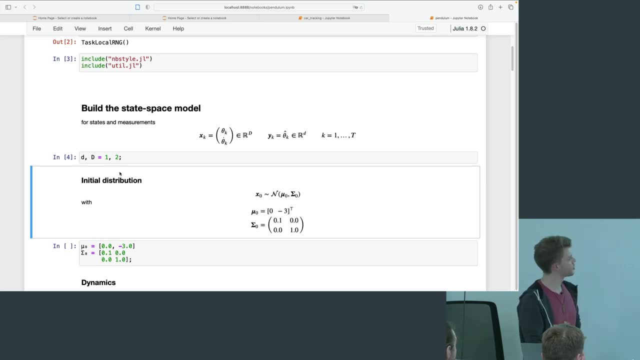 and our measurements are actually scalar. Okay, so this is quite simple so far. We are going to start off with an initial Gaussian distribution. We are going to initialize the mean at zero angle but an initial momentum, by setting the angular velocity in the beginning. 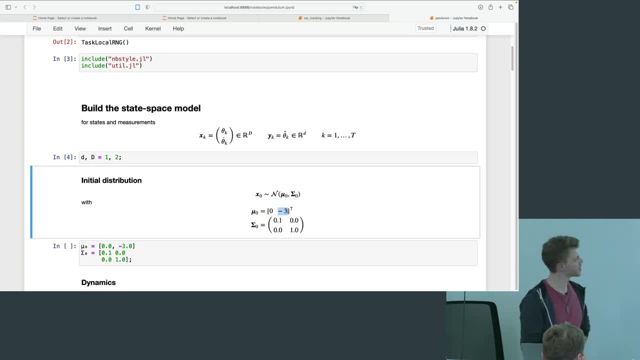 to a non-zero value minus three. I just chose this. It's not set in stone. We are going to encode that we are quite certain about the initial angle but a little less uncertain about the initial angular velocity by having here not a scaled identity matrix. 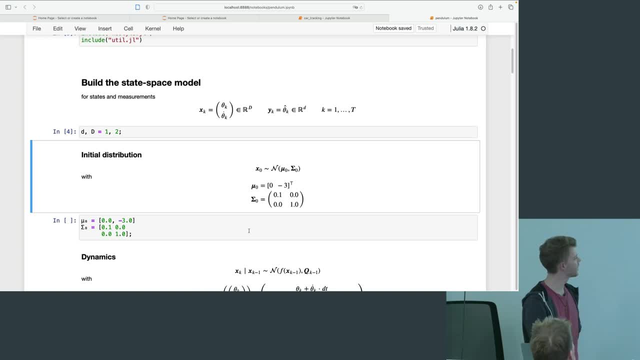 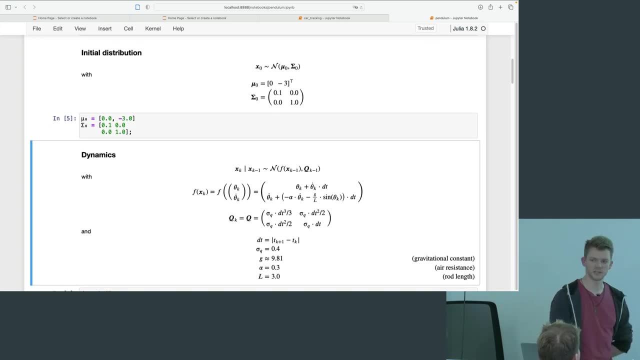 but still diagonal. It's just this initial covariance matrix. We are going to execute this in code as well, And now we are going to set up our dynamics model. So this now gets a little bit more interesting. We have now this non-linear state space model. 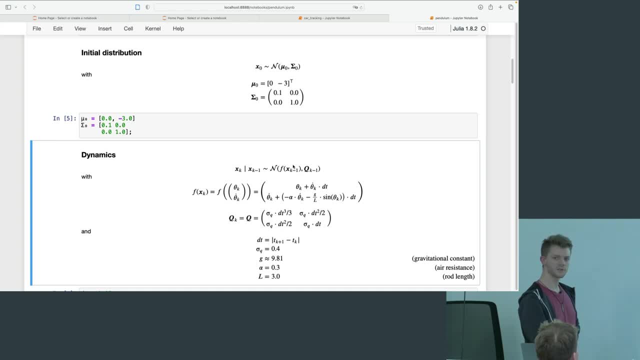 where xk given, xk minus one, is this non-linear transformation of our previous state? and this non-linear transformation looks like this: So f maps our state vector of angle and angular velocity to a new vector of angle and angular velocity that changed To the previous angle. 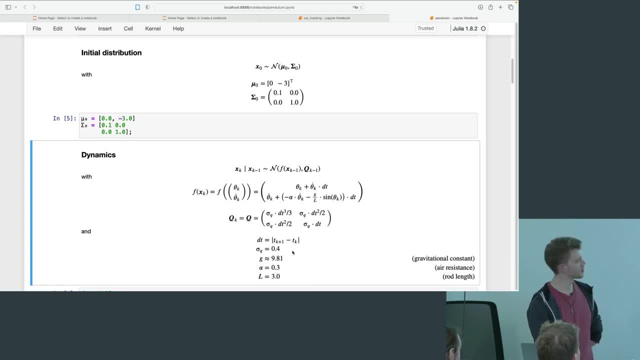 we add again this time step that is computed from the difference of the subsequent time steps: k plus one and k times the angular velocity. We just build this product and add it to our current angle For the angular velocity. we add to our current angular velocity this term. 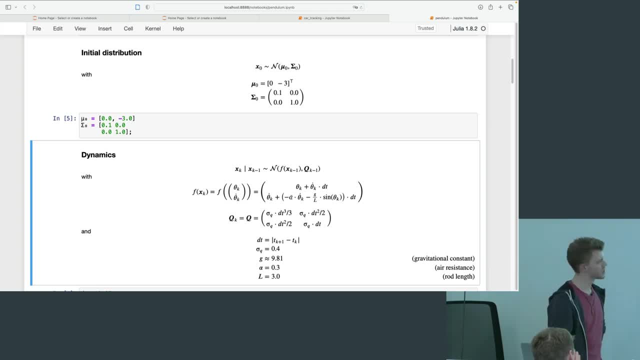 where we have this resistance or friction parameter alpha, which I just set to 0.3, multiplied with the angular velocity minus g, divided by l, where g is the gravitational constant of our planet Earth, which is roughly 9.81,. 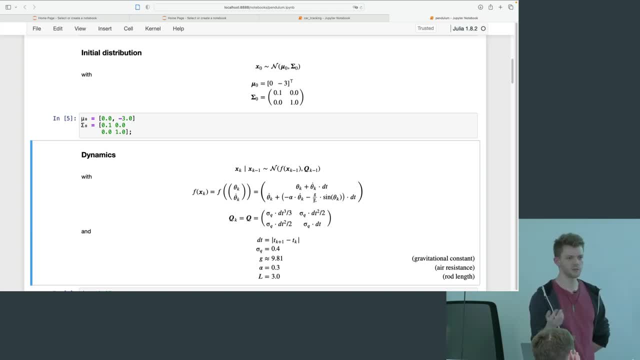 divided by the length of the rod of the pendulum- which obviously also affects our dynamics, which I just set to 3, multiplied with the sine of the current angle, And all of this we again multiply with our time step. Okay, You don't have to understand how this function comes about. 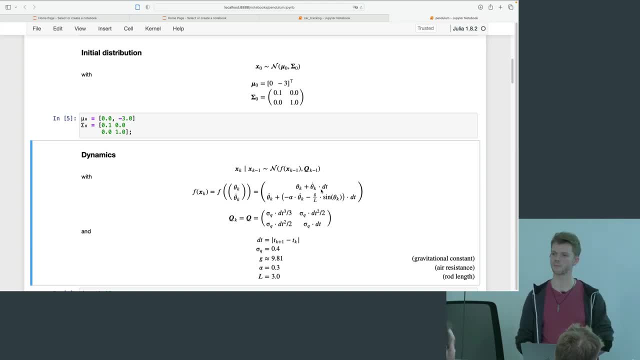 or why on Earth this thing here models the dynamics of a pendulum. But I promise you you will learn about these types of equations next week from Nathanael, And these are actually quite interesting- one of my favorite topics to study. Very cool stuff. 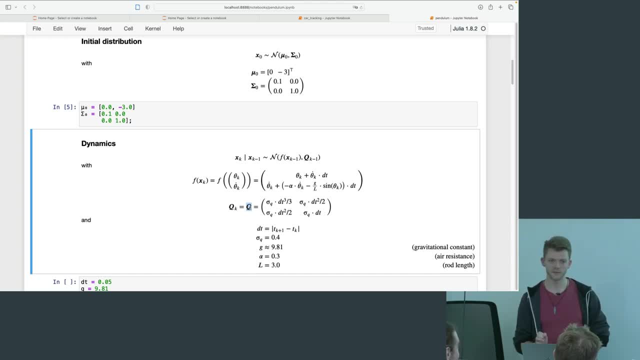 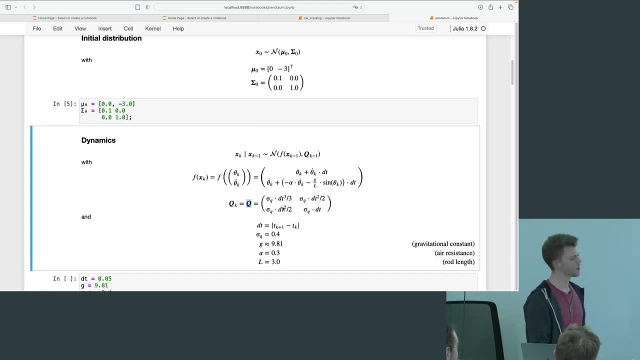 We are going to choose as our process: noise, covariance, again this very complicated matrix which involves some weird polynomial terms of our time step. I'm again not going to talk to you about how this comes about, just have to accept it for the moment. 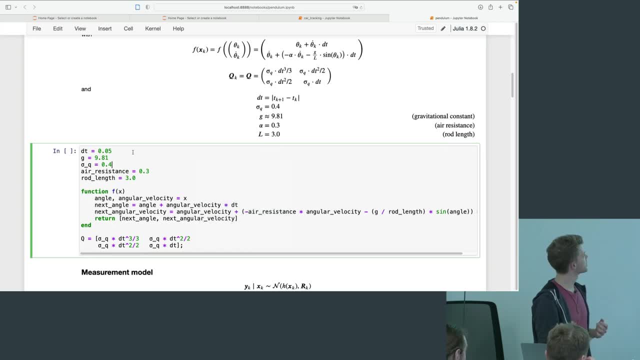 And this is our dynamics model. Okay, How does this look in code? We set our time step to 0.05.. We set our gravitational constant. This sigma Q term just basically scales all the terms in this process: noise, covariance matrix. We could also put it in front here. 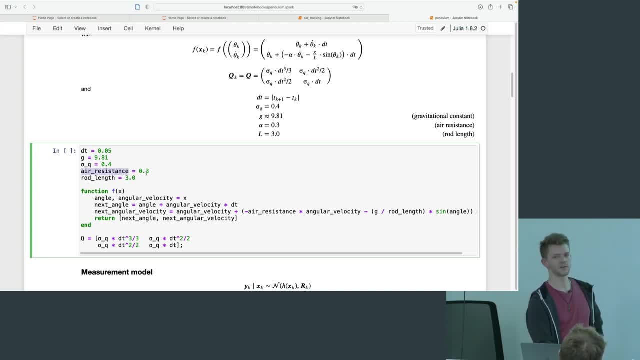 It's not very interesting. We have this air resistance term that influences our dynamics, or maybe not air resistance, maybe a better term would be the friction right, Just a general resistance term, And we have this rod length of the pendulum. 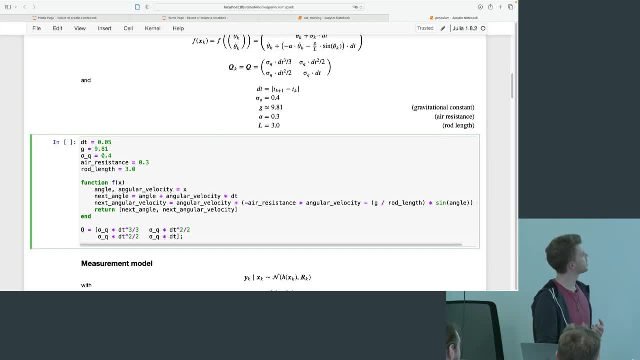 And we are going to write this down in code. This is just basically what you see here, just that I substituted every theta with angle and every theta dot with angular velocity. It gets quite complicated here. in the end, We return the new state vector. 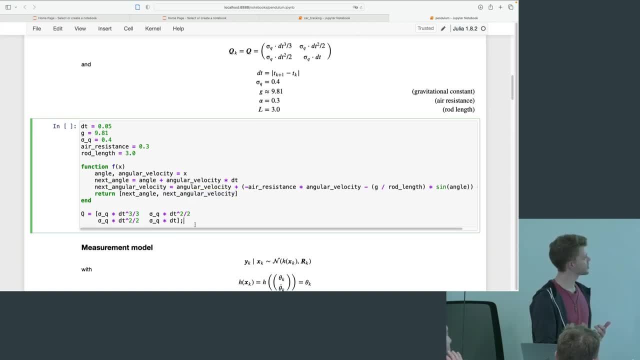 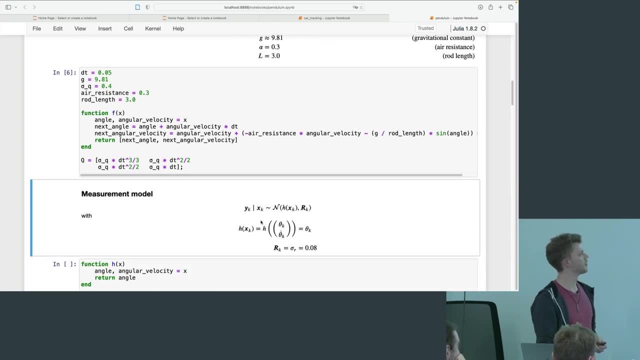 and this is our nonlinear dynamics, Our process noise covariance matrix, and we have our dynamics set up. As for the measurements, we actually have quite a simple model. H of the state vector is just the first component of the state vector, similar to the car tracking example. 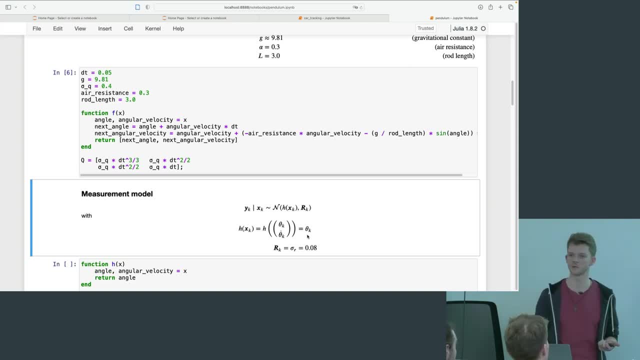 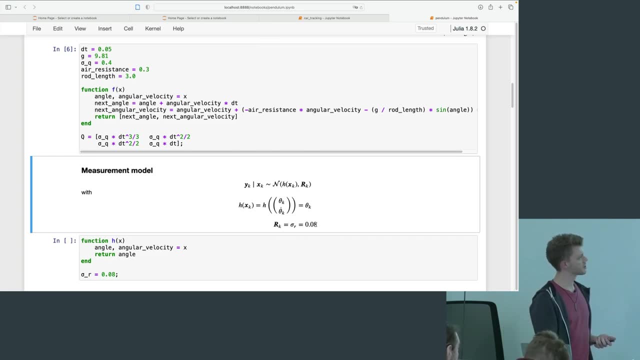 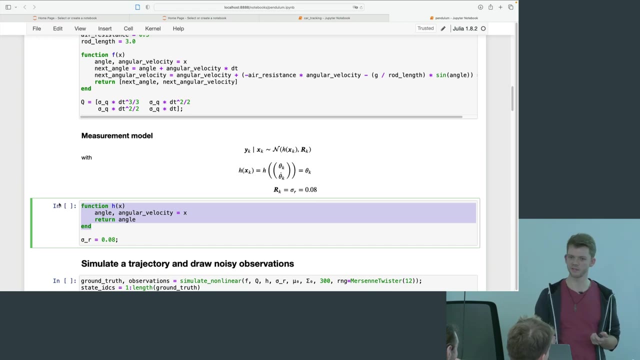 Notice, this is actually a linear model, so we didn't even use a nonlinear measurement function here And we have a scalar measurement noise of 0.08.. Just for the fun of it and that you can see the extended common filter equations later on: 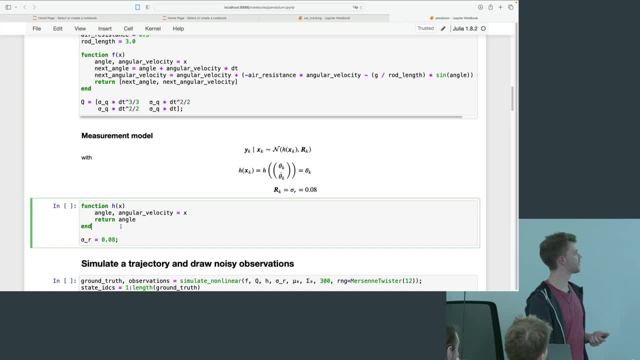 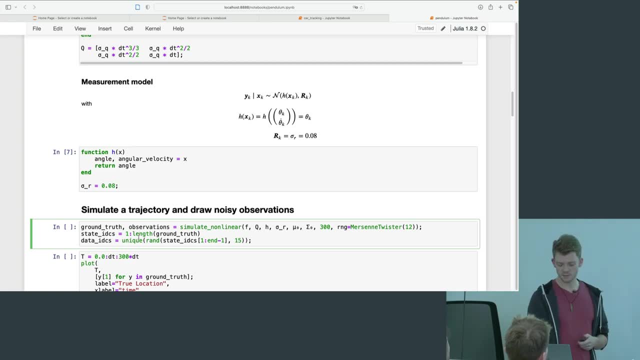 I actually wrote down this linear measurement model as a function h of x. Okay, let's execute this. We are again going to simulate now our state space model, where we draw one realization of the state space model, so one dynamics unrolling, so to say. 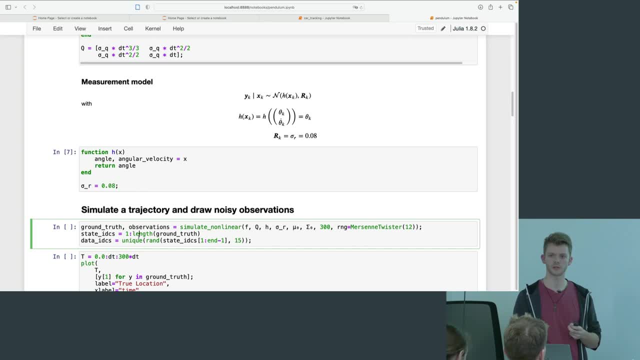 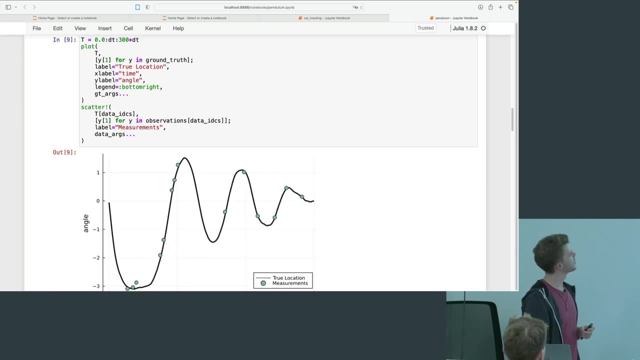 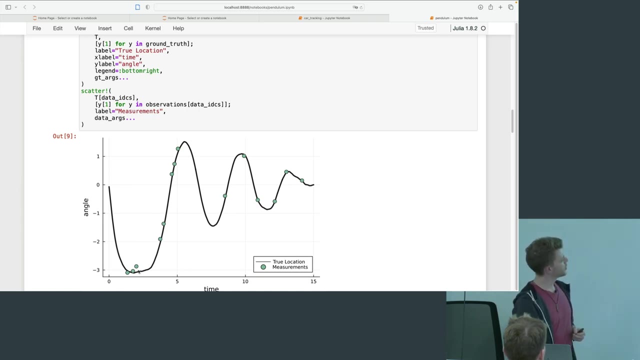 that gives us our ground truth, and we are going to draw the according data as well And we're going to plot it And this is what we end up with. Okay, that looks familiar, but a little bit weird, right? You see here that we have some wiggling going on down here. 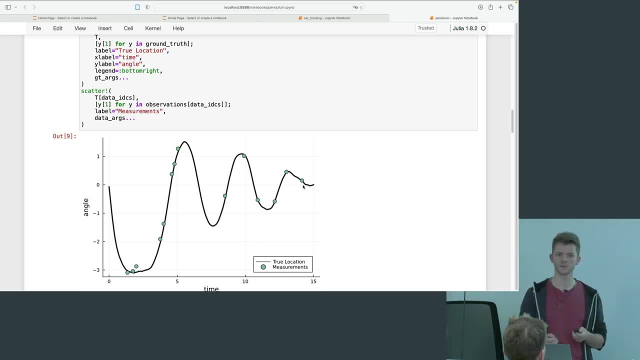 and also here that it's not a perfect oscillator. This is because we are looking at one realization of a state space model with a stochastic system. This is, if you will, a pendulum in the wind, So from time to time there's random momentum coming in. 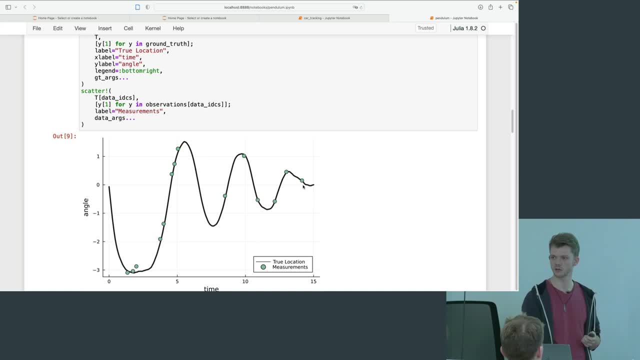 changing the dynamics of the pendulum. That's why we don't see perfect oscillations here And we have some measurements- also noisy measurements, at a few random time steps, And we are going to use these measurements and the extended Kalman filter in Smoother. 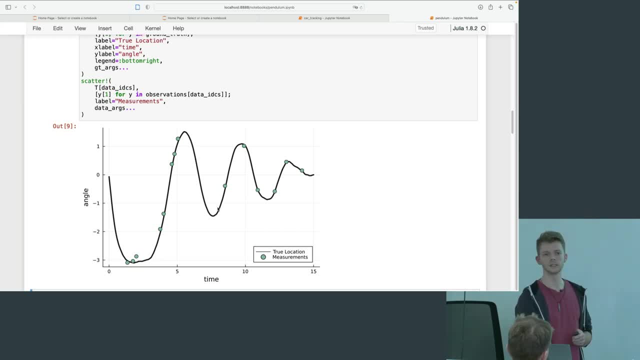 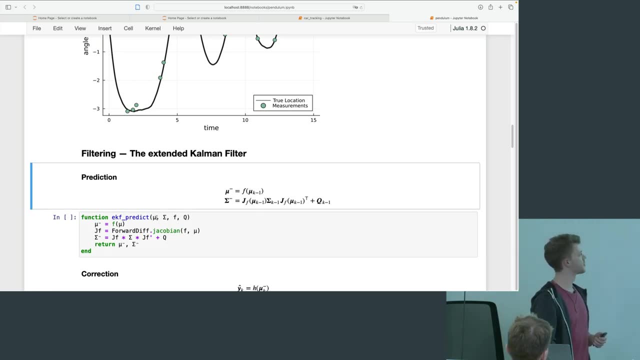 in order to get a good estimate of this ground truth trajectory. Okay, The Kalman filter, extended Kalman filter. equations in code. just take the filtering mean, the filtering covariance. the nonlinear function f that describe our dynamics and the process. noise covariance matrix Q. 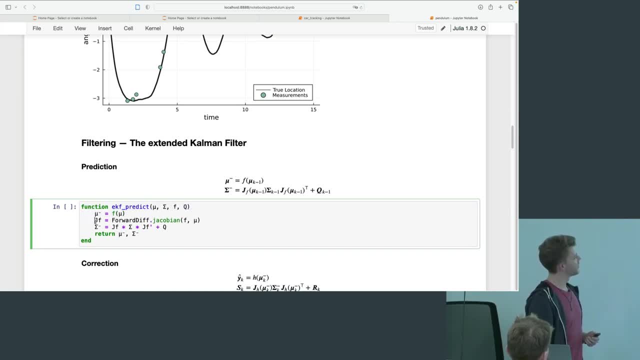 compute our predicted mean by evaluating the function, then computing the Jacobian. And what I'm doing here is I'm calling a package that uses automatic differentiation. Probably all of you know that. Maybe few of you saw it other than in the context of deep learning. 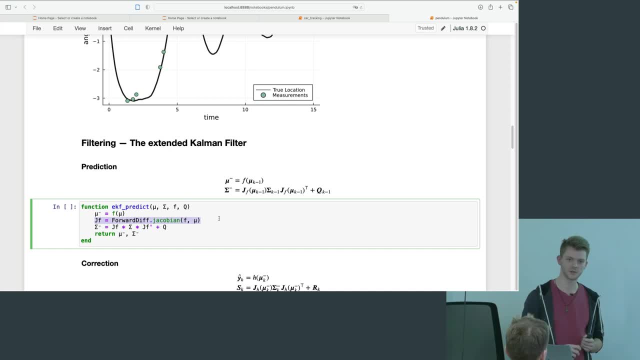 So you can use automatic differentiation for other things than training deep networks. So that's cool. Of course, for this very simple model you could just write down the Jacobian on paper. but as soon as the models get very complicated you might want to consider making use. 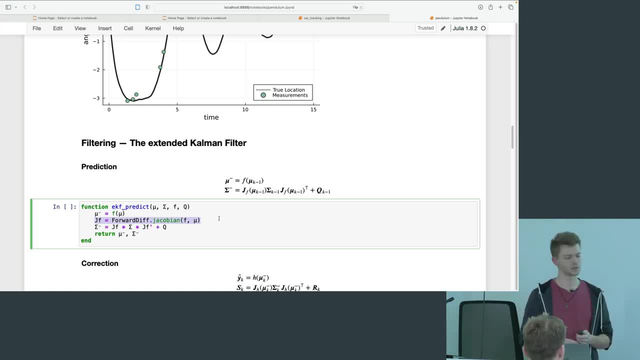 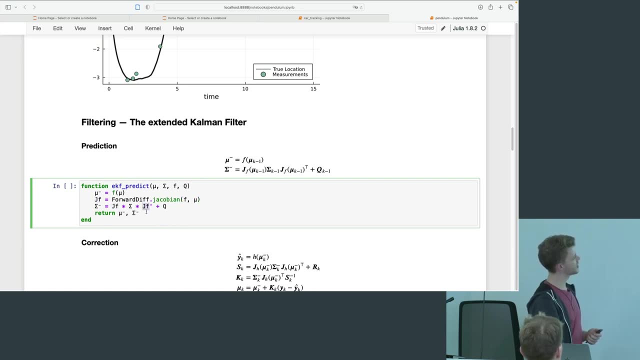 of this very cool technique called automatic differentiation. So I do this here for the simple model, because I'm lazy, I use this Jacobian matrix, substitute our transition matrices with that and return our predicted moments For the correction. we do exactly the same thing. 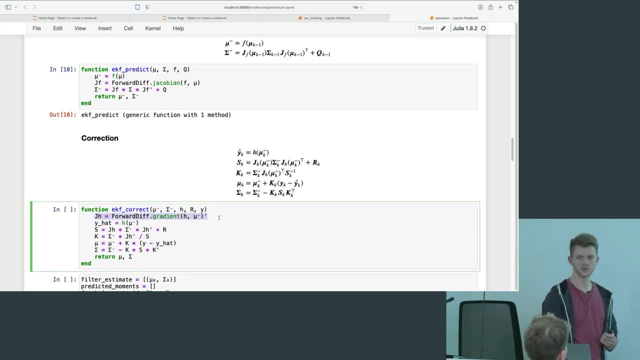 We compute our matrix, our gradient information. So this is not a Jacobian now, because we have a function mapping from R2 to the real line, so it's a scalar function. So we just have basically one row in the Jacobian: It's our gradient. 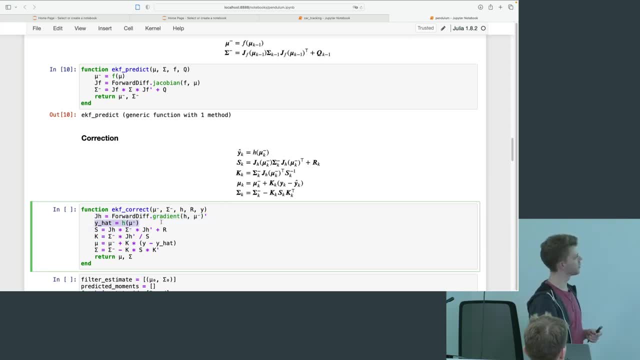 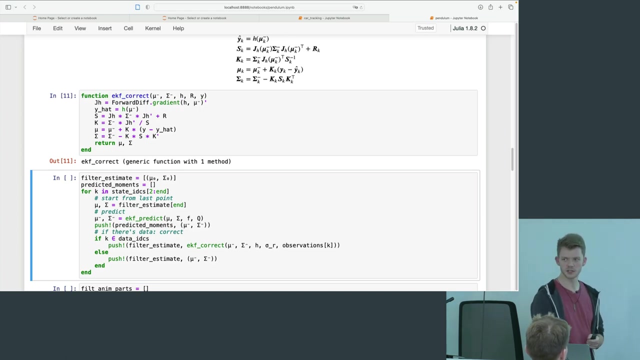 And we compute the measured observation, No, the predicted observation, using the measurement model on the predicted mean and then compute basically just using the Kalman filter equations, our predicted or our updated moments, mu and sigma. Okay, Clear, Then everything I changed in this loop. 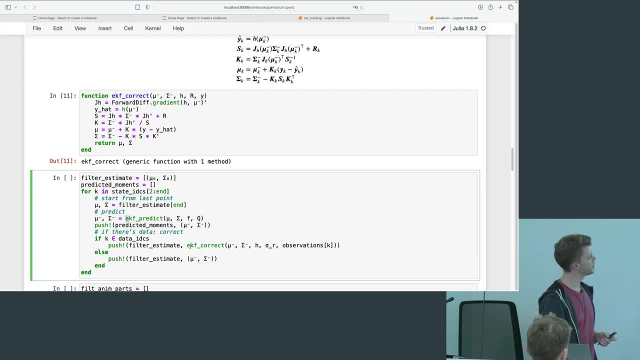 is. I added an E here and an E here. Everything else stays exactly the same. It's just a loop going over our state indices. We spare the first one because it's just our initial moment. We select from the very end our current filtering estimate. 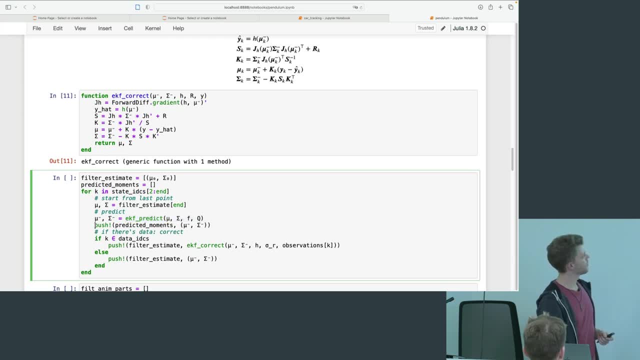 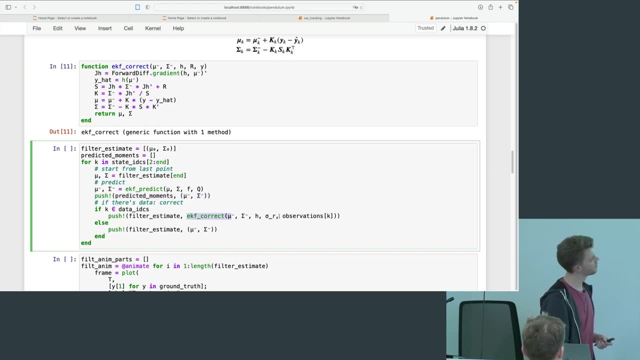 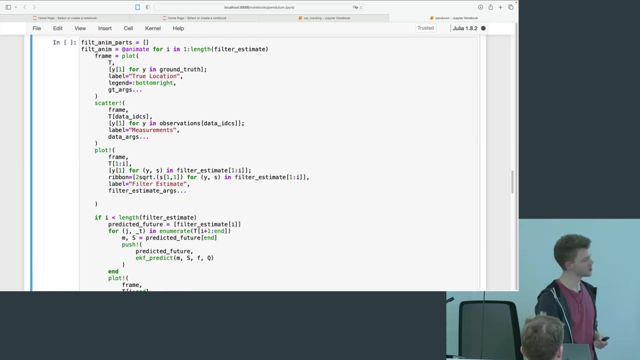 predict the next ones again. push them to a list because we need them later for smoothing. If there is data we correct for the newly gained observation Else, we're just going to push our predictions. Okay, Let's execute this. It's actually very fast. 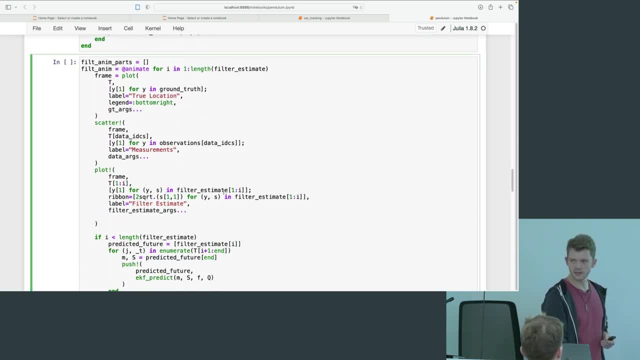 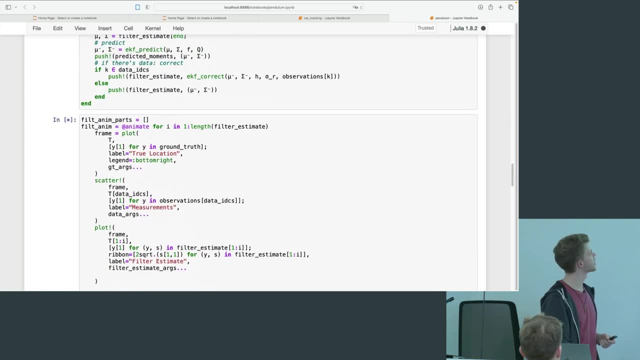 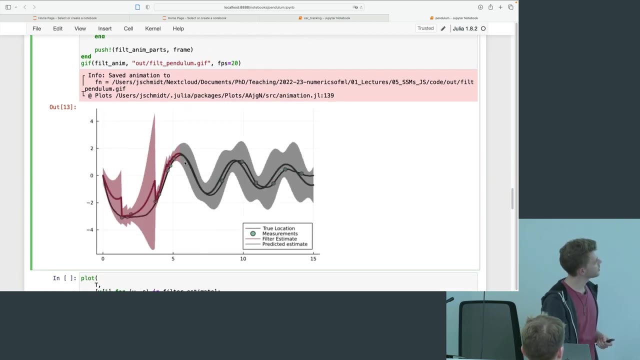 It's already finished. And now let's look at the animation. No, let's look, Yes, let's look at the animation that shows us our filtering estimate of this pendulum trajectory. What? Okay, Here you see it. See, here in the right. 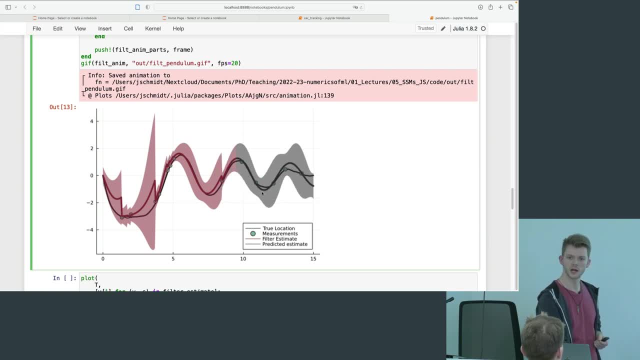 it's very interesting: The predicted trajectory already encodes now this oscillatory behavior, because we informed our prior dynamics about our model and it's nonlinear, So it's not just one line going in the future but it's already exposing these nonlinear dynamics. 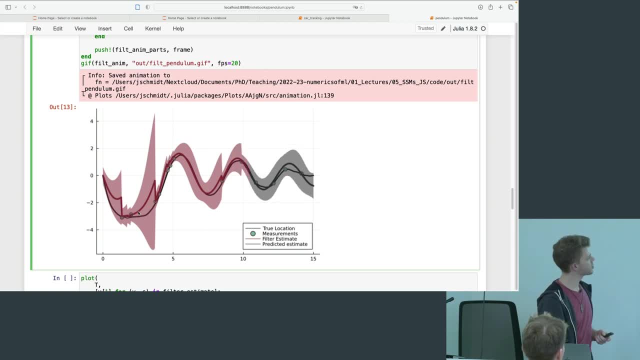 So this is quite cool. And in between measurements where the prediction maybe was not so good, the uncertainty goes fans out very rapidly And then, as the new data point comes in, it snaps back onto this data point and corrects on the basis of the data we've seen. 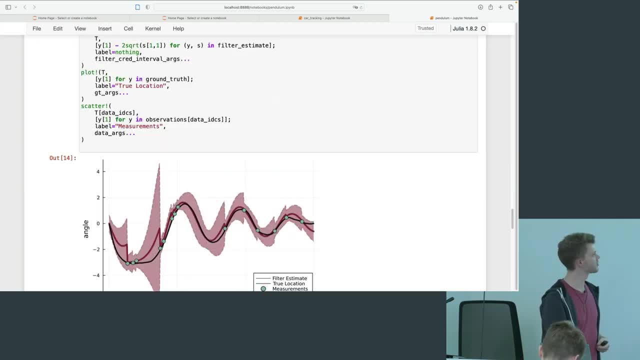 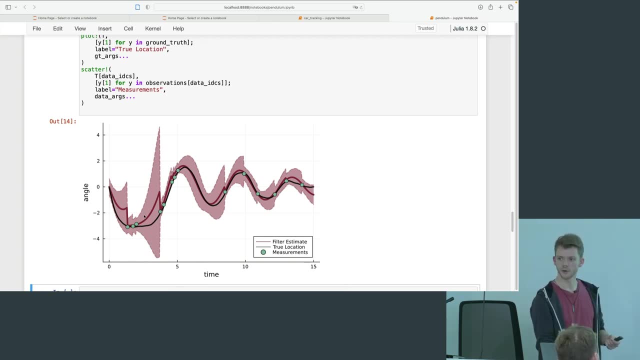 Okay, So this is our filtering estimate. We don't have to make multiple plots now because this is a time series And these two marginal standard deviations here in this shaded area are the correct depiction of our uncertainty estimate. And this is the filtering estimate. 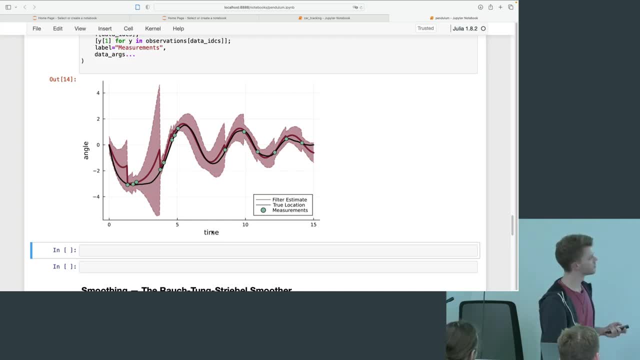 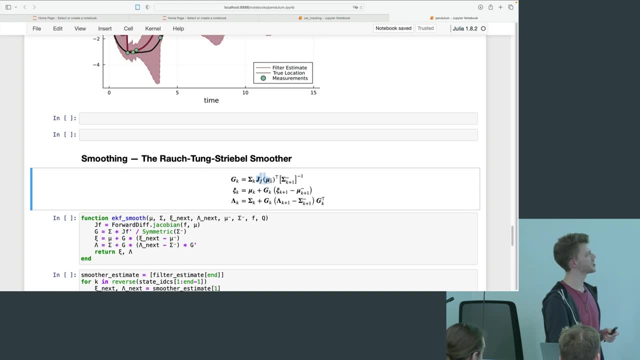 Okay, cool, Looks nice, doesn't it? Now that we already learned about smoothing, we can just go on and implement the extended Rauch-Tung-Striegel smoother as well, where we just substitute our transition metrics with our Jacobian of our nonlinear dynamics model. 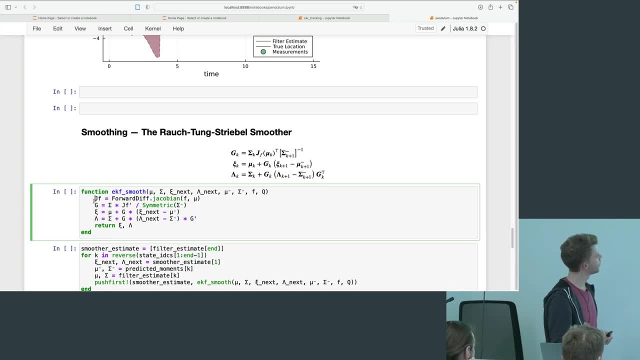 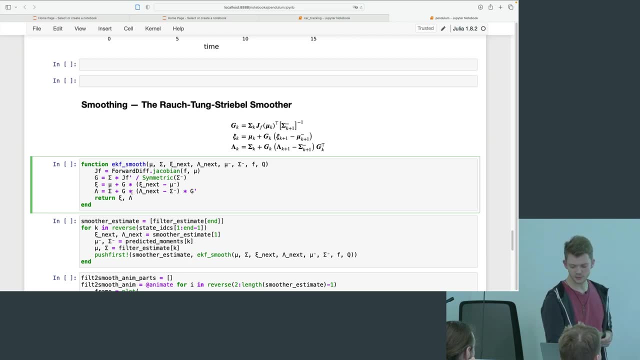 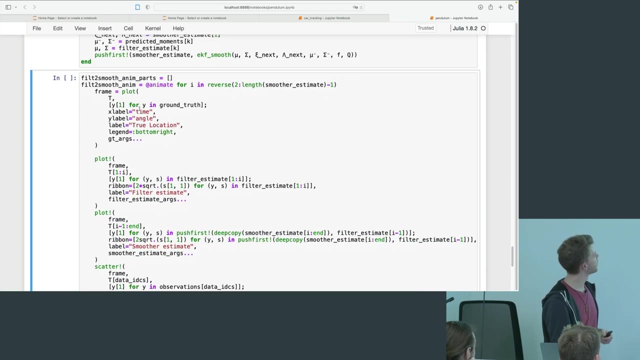 Okay, The smoother again. uses automatic differentiation, computes our smoothing gain. smoothed mean smoothed- covariance returns it, and then we execute again our backwards loop. You know this already, Not going to go over that again. And then we again can look at a fancy animation. 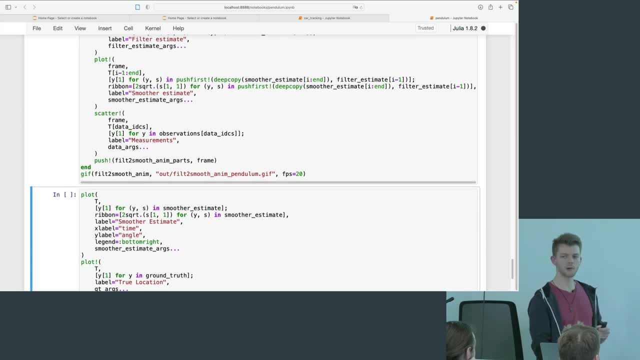 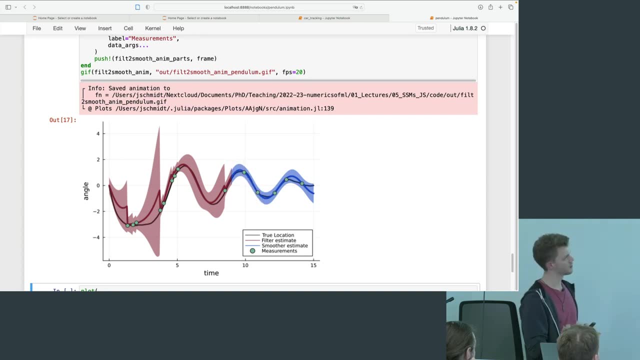 where our smoother again tidies up our filtering estimate from before by going backwards through time and computing. actually quite nice interpolants in between those data points. This is a Gaussian process, posterior, marginal evaluated at all the points that we considered in our sequence. 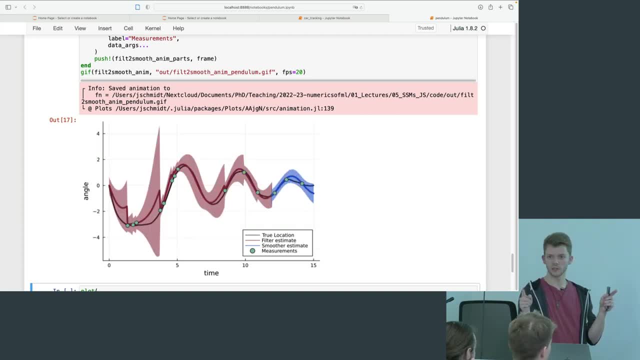 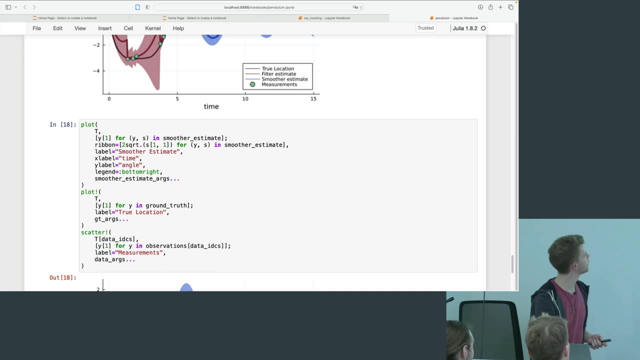 Computed in once linear and forward direction and once linear in the backward direction. So this is quite cool, right? So this is how it looks, what it looks like in the end. It's a nice interpolant in between the data point and it covers the ground truth trajectory nicely. 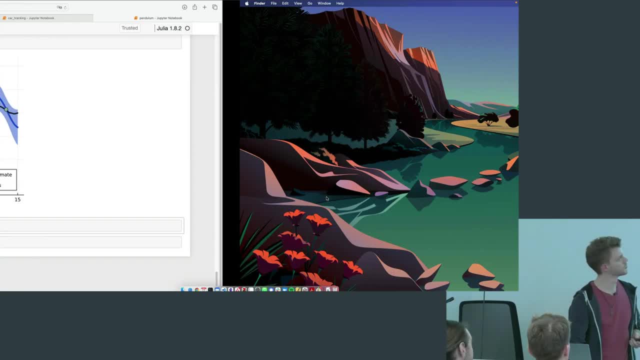 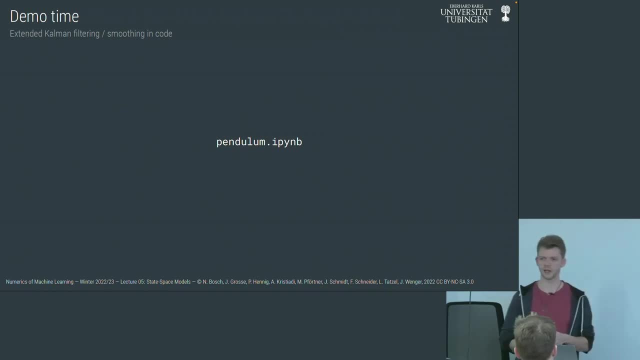 in its uncertainty. Okay, Whoops, wrong direction. Okay, With that, I'm actually almost finished with my lecture. So you made it through the theoretical part such that we can go on next week to actually really nice dynamics That we can look at. 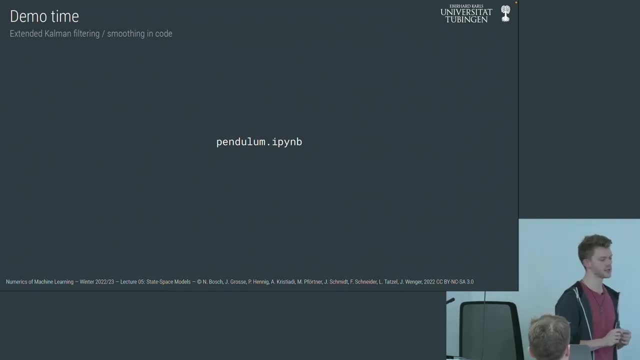 First of all, though, I don't want to leave without telling you that extended Kalman filtering- of filtering Kalman filtering in general, is not the only way to do Bayesian filtering and smoothing. It's just one way, and it's a way that, most of the time, 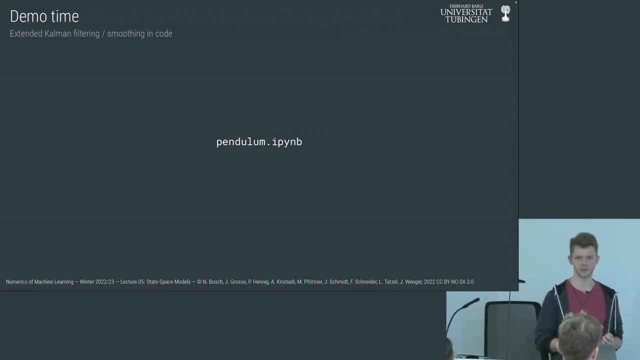 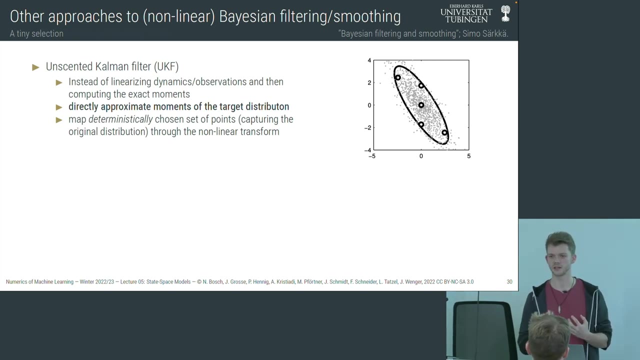 actually works quite nicely and it's very easy to understand and implement. However, I want to present to you now an alternative, and I'm not going to present it, I'm just merely going to mention it: that there's an alternative that's called the underline. 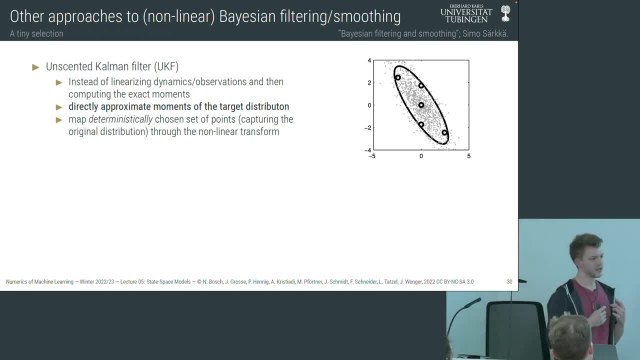 It's an uncentered Kalman filter and while the extended Kalman filter approximates the model and computes the exact solution, the uncentered Kalman filter leaves the exact model intact, so the nonlinear function, but approximates the distribution, It does so in a very complicated way. 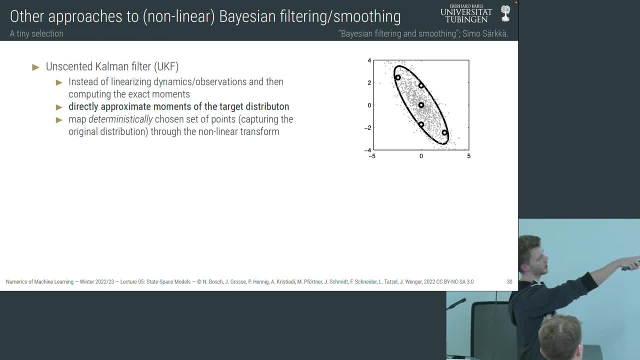 It deterministically chooses points called sigma points from this Gaussian distribution that you see here on the right, represented by these samples in the background, and maps these points through the nonlinearity and then uses the mapped sigma points to compute a Gaussian approximative distribution on the basis of these points. 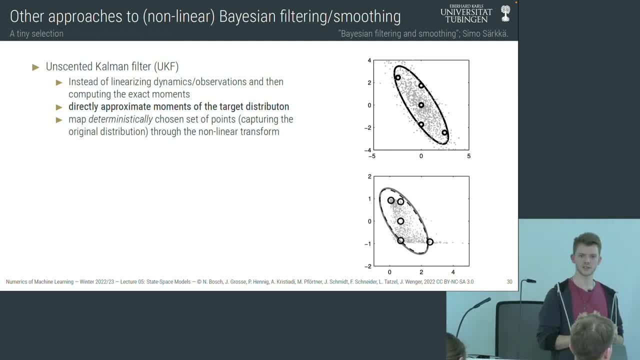 I'm not going to go into detail. I just want to let you know there exist other methods that you can use if the extended Kalman filter doesn't work. Now, coming back to your question over there somewhere, when you asked me whether we can drop, 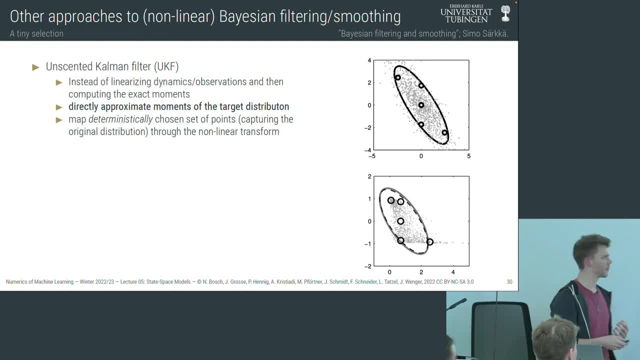 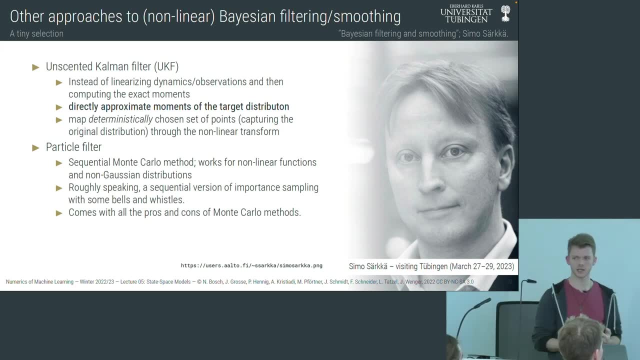 the Gaussian assumption as well. there, I told you, we have to open up a box of more complicated algorithms, and one of these algorithms is the particle filter. It's a sequential Monte Carlo method and it works for nonlinear models. it works for non-Gaussian models. 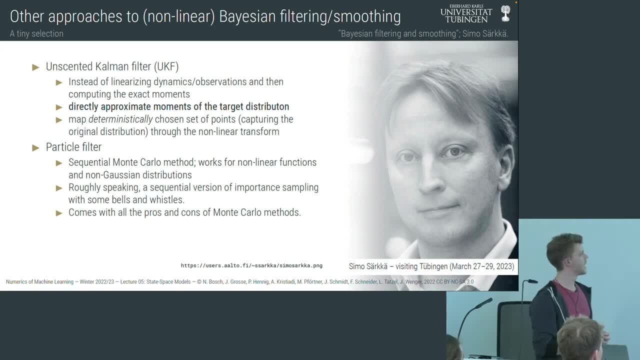 it approximates the actual true posterior under your model. It's, roughly speaking, a sequential version of importance sampling and all kinds of complicated stuff added to make it work, and it comes with all the pros and cons of Monte Carlo methods, in that, for example, first and foremost, 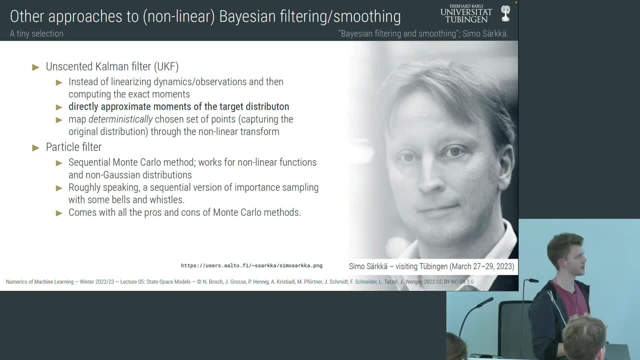 it's very expensive to compute and a bit harder to implement than the extended Kalman filter, But it's a very cool method and if you want to learn about this, there is a book called Bayesian Filtering and Smoothing- Bayesian Filtering and Smoothing. 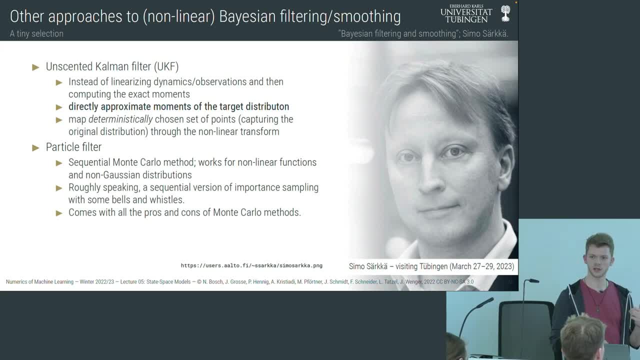 I actually used a lot of this in this lecture to create this content. It's written by Simu Zerke. Simu Zerke is a researcher in Aalto in Finland and he's actually going to visit Tübingen late March next year. 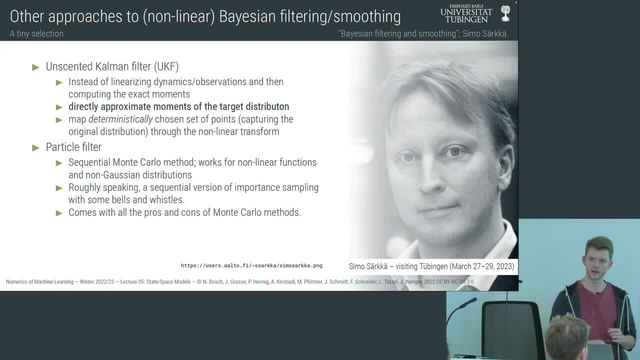 as part of the Probabilistic Numerics Spring School. that has been announced yesterday or the day before yesterday, So maybe you even have the chance to listen to a talk given by him if you're interested in the topic, And I definitely recommend if you're interested. 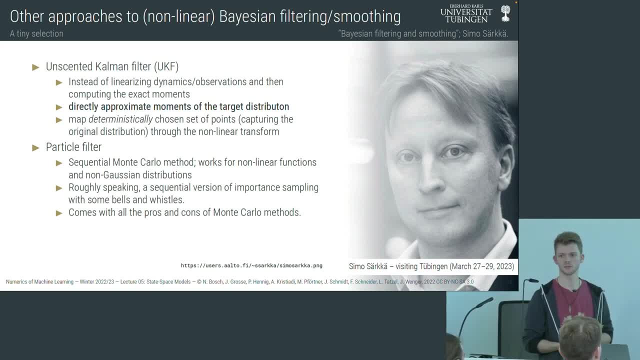 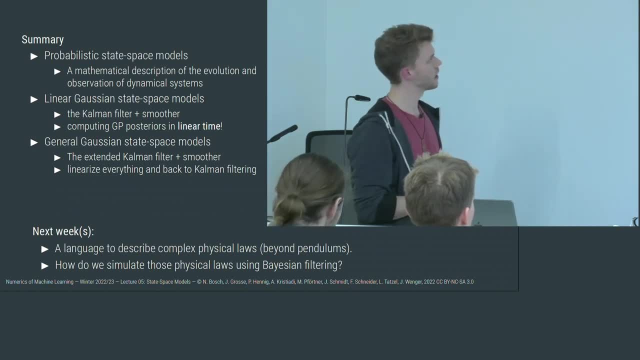 having a look at his book. It's actually very accessible. Finishing off now, let us quickly recap what we learned about today. We learned about the language that we use to describe dynamical system probabilistic state space models, and we chose a special kind. 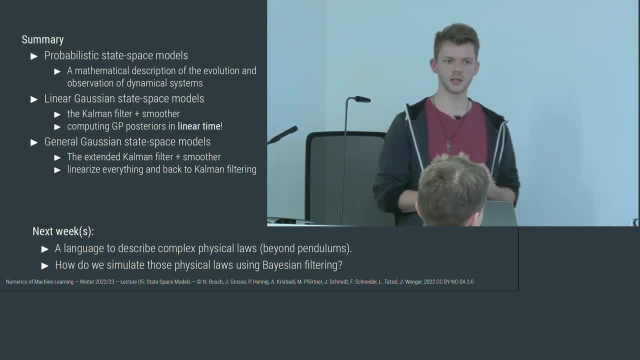 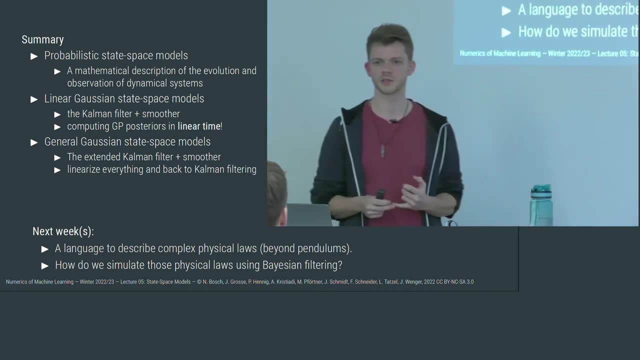 of these probabilistic state space models, in that we chose a linear Gaussian model such that we can compute the prediction and the filtering distribution in closed form, just using linear algebra, by using the Kalman filter. We extended this because we need to do this. 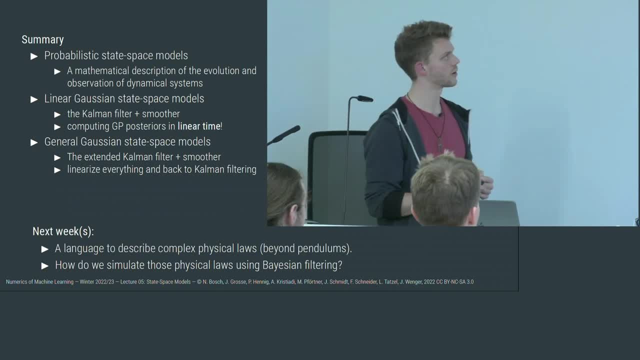 to nonlinear models. We will use this for our simulations later on by using the extended Kalman filter, which is just an extension of the Kalman filter that linearizes everything in your state space model and uses the Kalman filter equations again. And now we can handle. 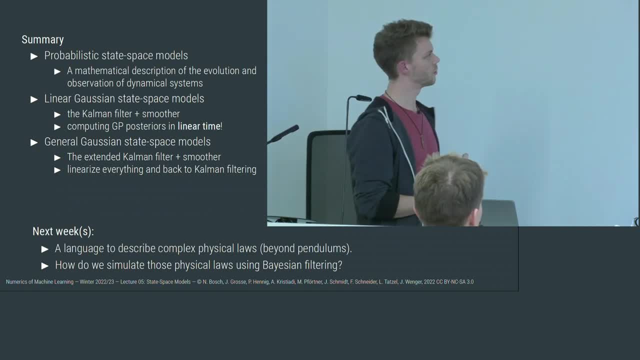 nonlinear dynamics, nonlinear measurements, in a really cool way. Next week I strongly recommend you coming back, because Nathaniel here will tell you everything about how to mathematically describe these dynamics themselves. So not the models for these dynamics, but the dynamics themselves. 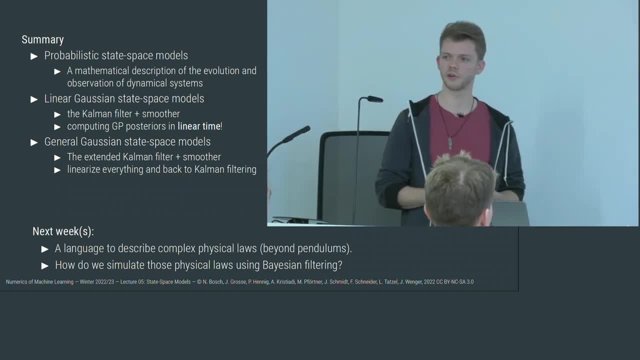 So he's going to introduce you to a language that's very powerful, that captures all sorts of laws of nature And in the lecture afterwards also given by Nathaniel. so in two weeks from now, he's going to combine today's lecture and the lecture given in one week. 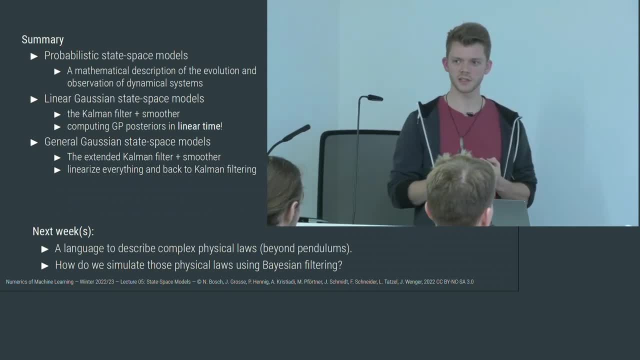 where we will learn how to use probabilistic numerics, ie Bayesian filtering and smoothing, to actually simulate those dynamical systems. So it is the combination of those two lectures. With that, I want to finish off by asking you to provide feedback. 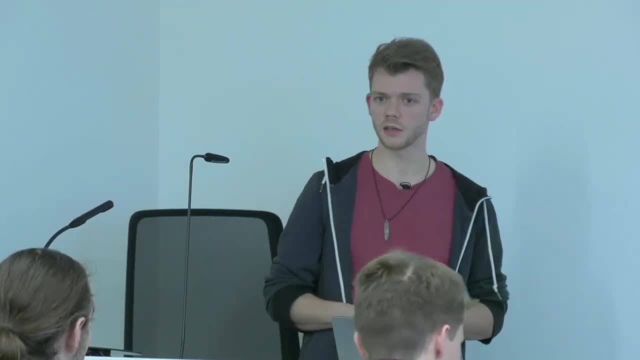 I'm very, I very much appreciate you listening to me today, and with that I finish off this lecture. Thank you for listening.